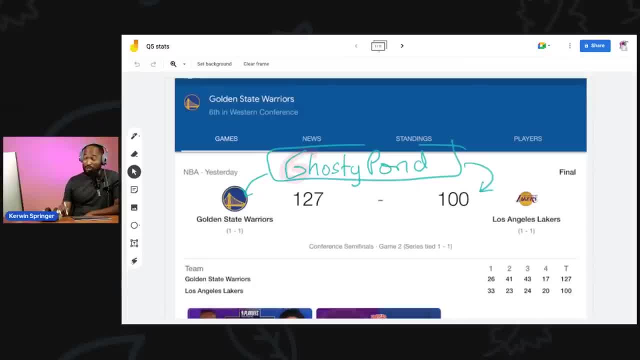 Ghosty Pun. you there, boy. I don't remember Ghosty Pun. Ghosty Pun was in my talks yesterday and saying that we're going to lose this match and thing. Ghosty Pun, have a nice day. All right, Let me jump into it. So today we're going to do statistics. That's the question five. 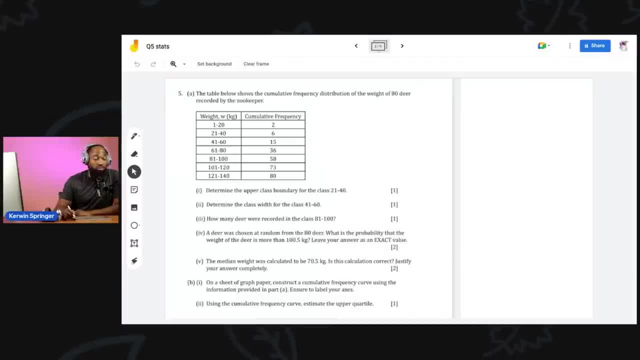 Today is the fifth day we're doing this and it's been a spectacular week. I am very tired, Not really from this, from other things- And I have AdMath class in a little bit. So AdMath students gears up, I have my AdMath lessons class. 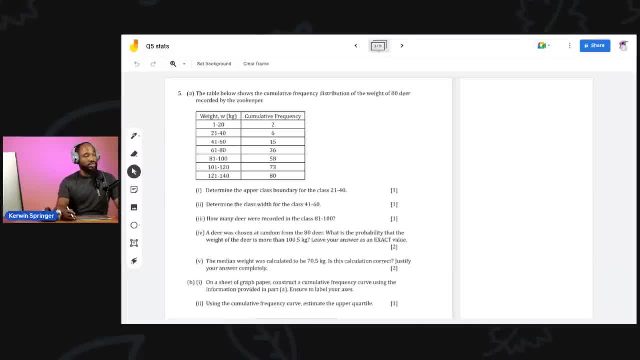 But the maths must go on. So we are going to do statistics today. Statistics: it usually comes in number five. It's one of those topics that isn't really tested in section two, that much. You don't really see any statistical stuff show up in section two of the maths paper. It can have a swing in the paper tree. So private candidates, be ready for that. 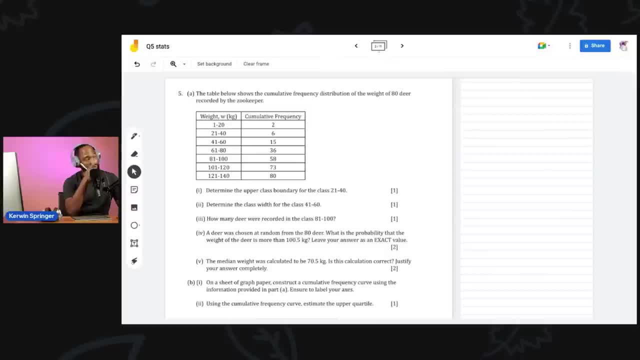 So this is this question here. This question here is about cumulative frequency and it's by far the most popular thing tested in statistics And it's like the hardest thing or the most comprehensive thing. cumulative frequency curves, But what can also be tested? 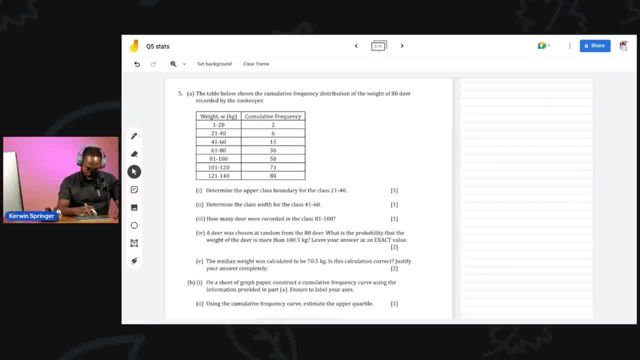 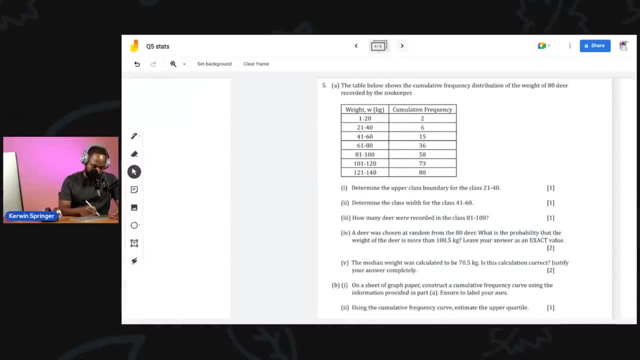 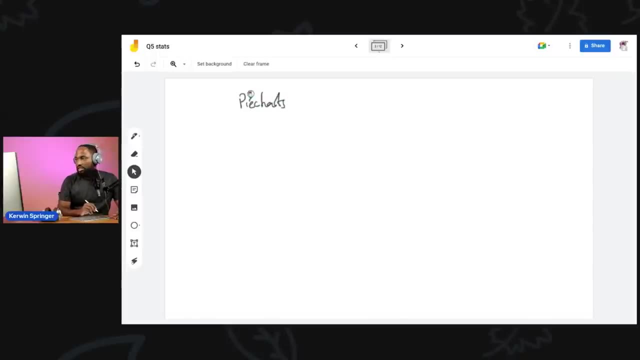 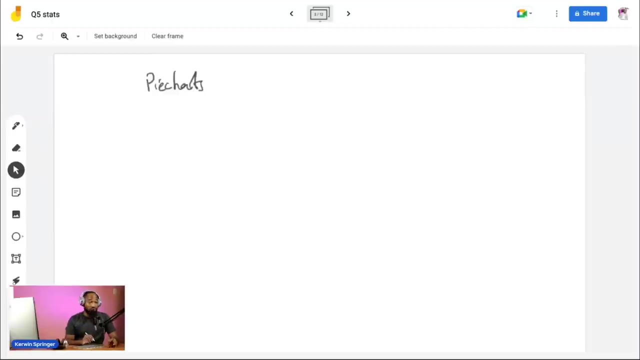 Let me see if I can get a blank page tree, A blank page tree. What can also be tested is different graphs. So of course, there's the pie charts, which have been popular these last few, These last few- What I'm trying to say, these last few exams, pie charts has been popular. Then there is histograms, and there are histograms and there is. 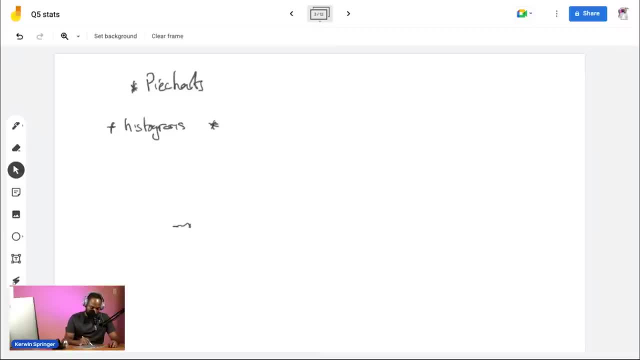 Why am I sticking to remember these things? I'm just Yeah, histograms and bar charts, And we have Frequency polygon And now coming back And line graphs, And then we have the big boy: cumulative frequency, Cumulative frequency curve. 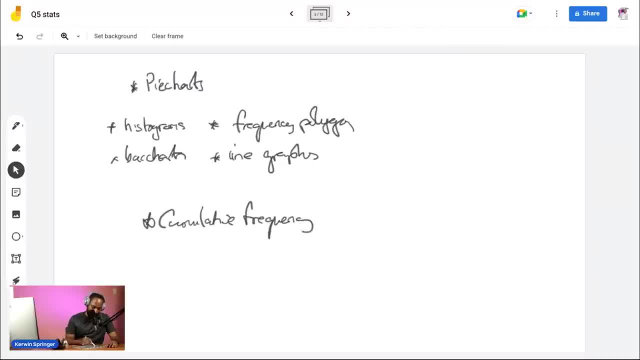 So what you should know is the difference between a histogram and a bar chart, the difference between a frequency polygon and a line graph. The histogram is a cousin to the frequency polygon, The bar chart is a cousin to the line graph, and the histogram and bar chart in the same family, and the frequency polygon and the line graphs in the same family, same vibe kind of thing. and pie chart, see by yourself. 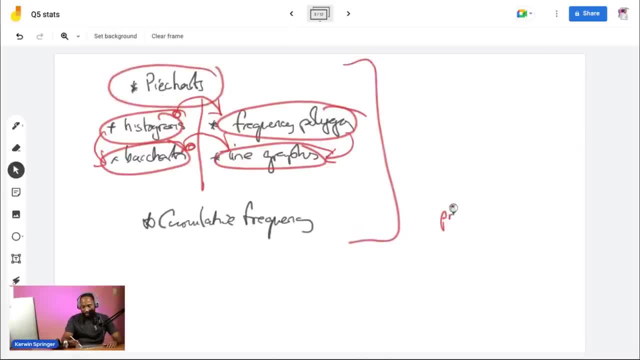 And, of course, all of this you would be. you would get a question on probability in the ending, a simple question: probability for CX is not a big thing, probability and you could get you know the quartiles and group data versus on group data stuff. 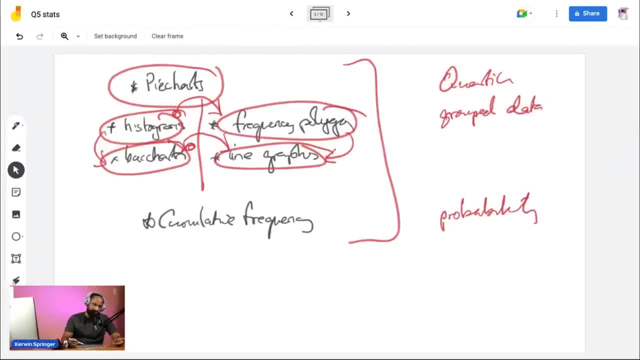 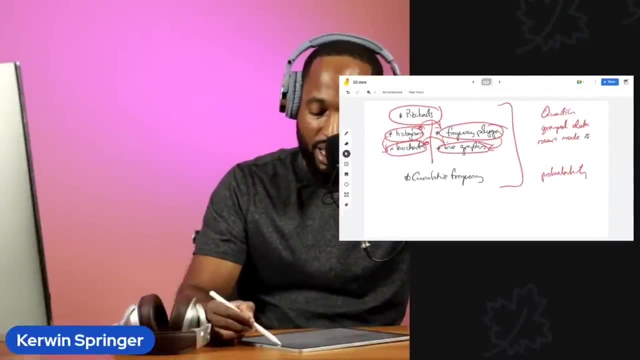 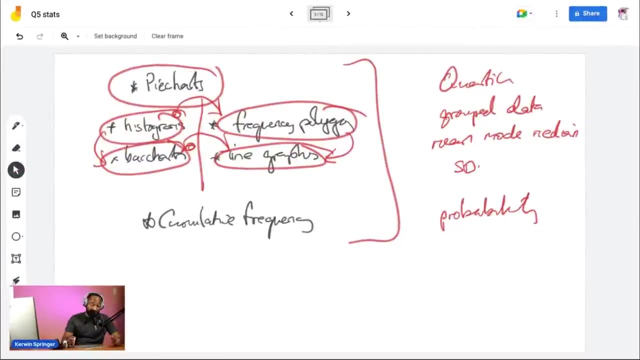 Yeah, Which would be A four. So on your list, if you have different measures of the statistical average, statistical mean mode, Media, and you could be asked to explain standard deviation S, the standard deviation. So we have a bunch of different things that you could be naked. 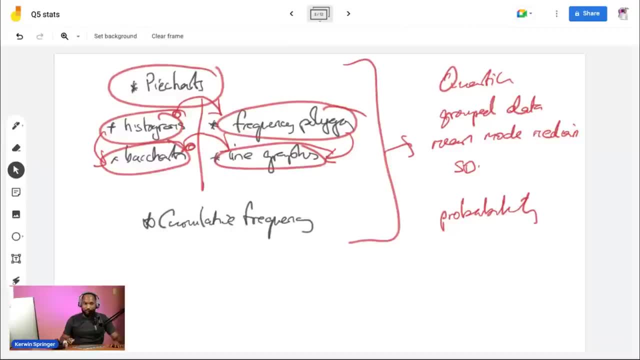 Push your pusher at With statistics. mind that everyone here to press the like button and that we're going to have a massive crash course, not this saturday, not tomorrow. the following saturday, from 12 to 12, 12 any day to 12, any night. 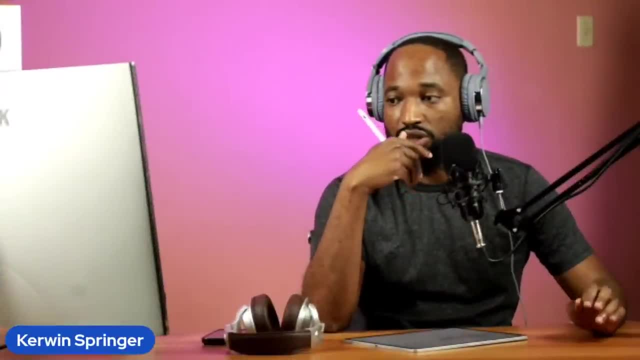 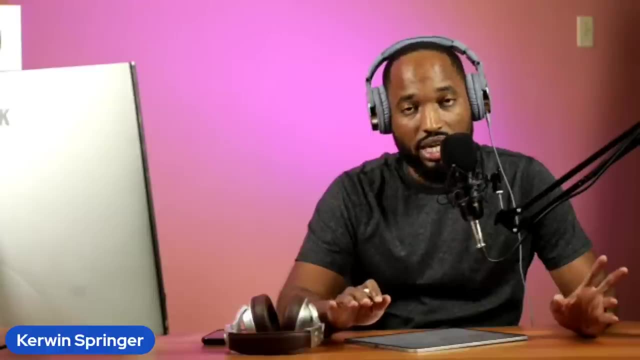 and, of course, you- you know the drill- your whatsapp, this number to join the crash course, the number that's showing up below here the screen, your whatsapp, that number, and you would talk to the admin and tell them: i want to join that crash coaster, so hold in and jump in, jump in, all right. 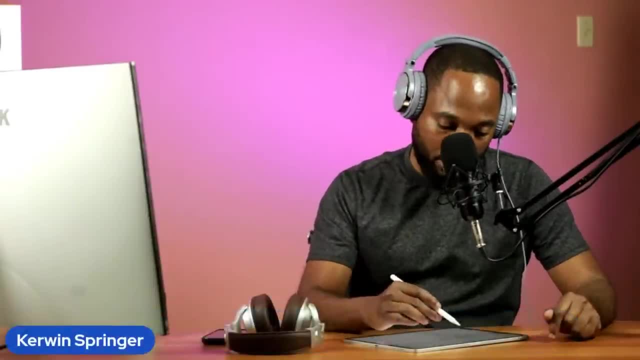 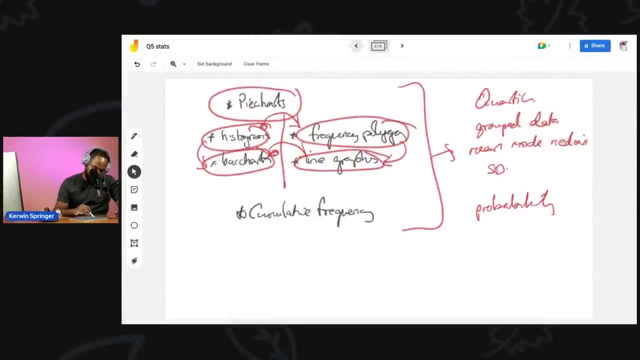 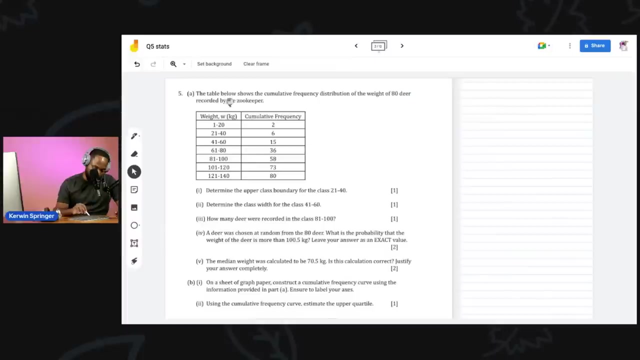 so good evening to everybody, ariel. let me just jump into the question now. so what we're seeing here, this is the weight. this is the cumulative frequency distribution of weight of 80 day, thereby recorded by a zookeeper. which zoo have 80 days in it, right? 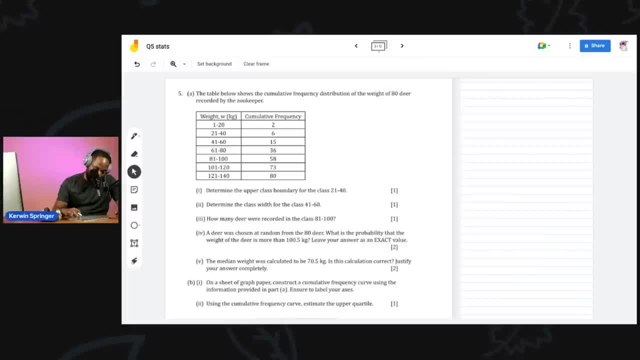 okay, there's really be making up some way things for this math thing called matter, what we know in these days they're now born- oh, this was so light. and then again more and more, now the cumulative frequency, and it's 80 days and all, and then you have the and then you need to determine the upper class. 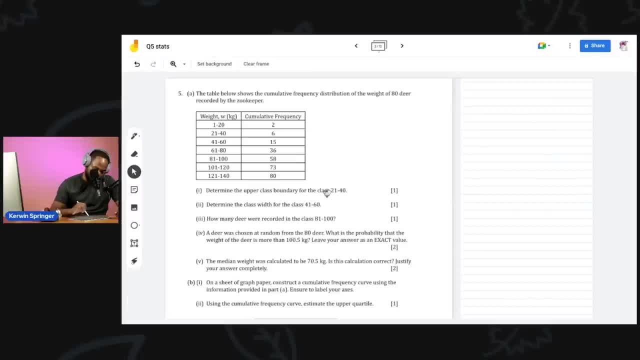 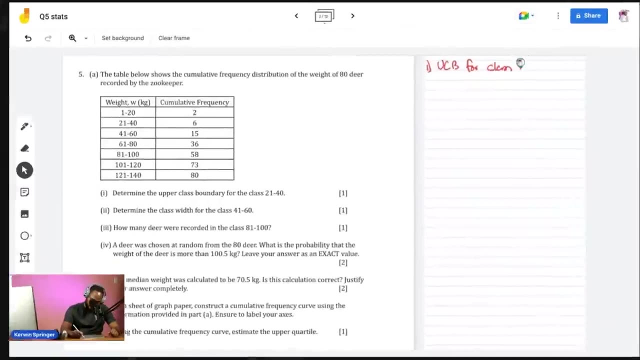 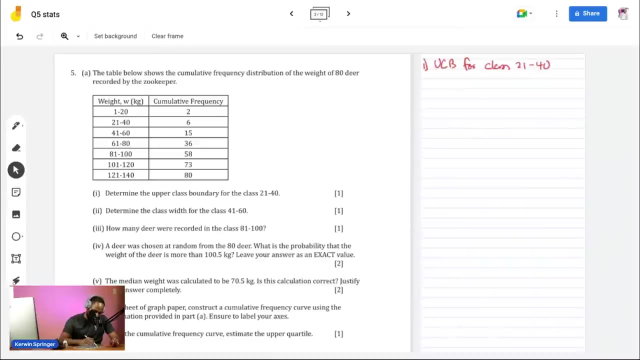 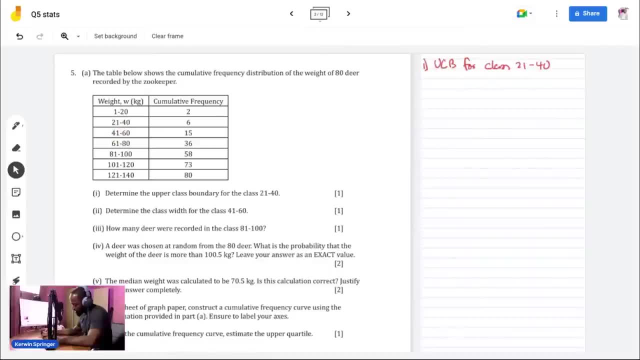 41. so the upper class boundary is 40 plus 41. divided by 2 it's 40.5, and you can just ride alone. oh gosh, kilograms, man kilograms. 40 point five kilograms determine the class with. so it's a class with always find. 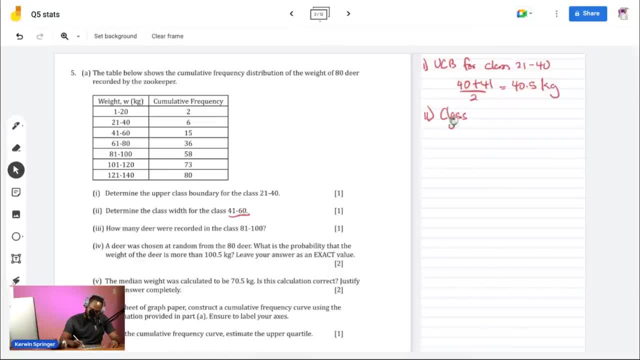 class with class, with any class which you take out, take out a tape and measure the weight of the class. now you don't do, don't turn. of course, Lord is the upper class boundary minus the lower class boundary of any class, class interested in. so it'll be sixty point five minus forty point five. agreed, because the 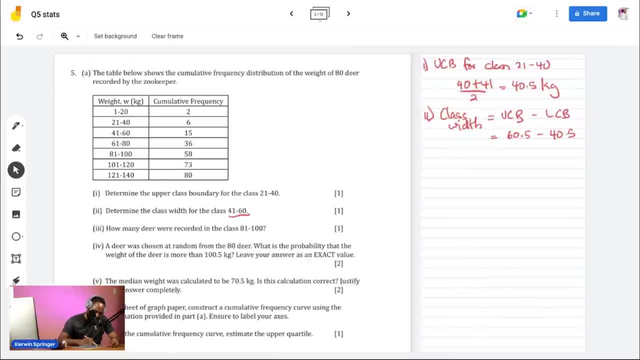 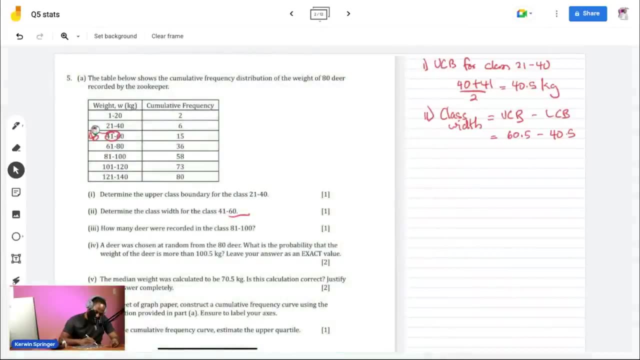 lower class boundary forty one is lower class boundary forty forty one is forty point five and the upper class boundary sixty point five. why is any chat? if you understand what in there, so you know, you know subtracting limits. it will say: for sixty minus forty one is actually six point five minus forty point five, and 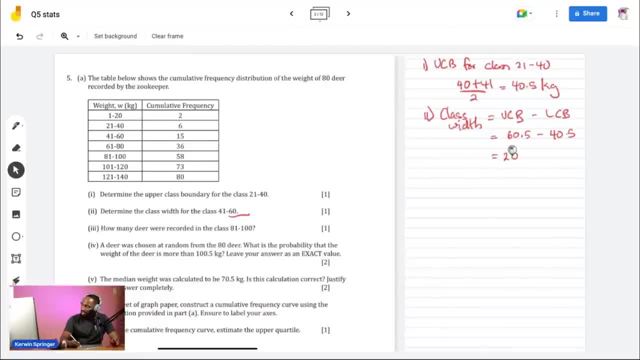 with that you get a nice beautiful twenty million kG. so I just download kG, I'll input kG again, mine. so I live gonna leave them. thing out. early exam: no units in your exam. how many there were recorded in the class? eighty-one thousand- Alright, so well. the 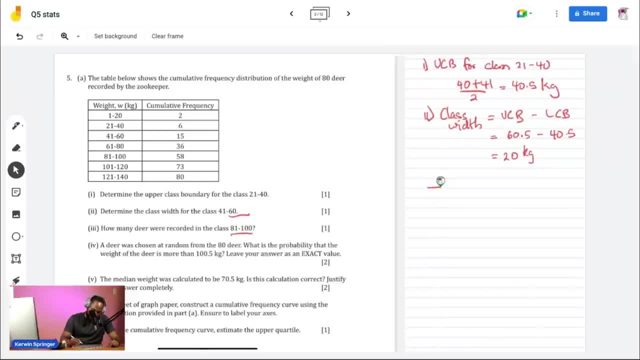 cumulative frequency left off at 36 there in the previous class. how much we had? we had 36 there and at the end of the this class, at the end of class, 81 to 100, all of a sudden we had. So previous class we had 36.. 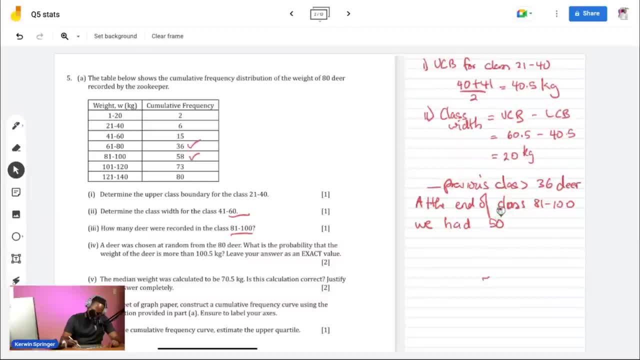 And this class reached 58 there. 58 there, There's is plural, It's plural there, There's, Or you just write there. I don't know. This is not English class, I feel it is this. So then, and therefore class 81 to 100. 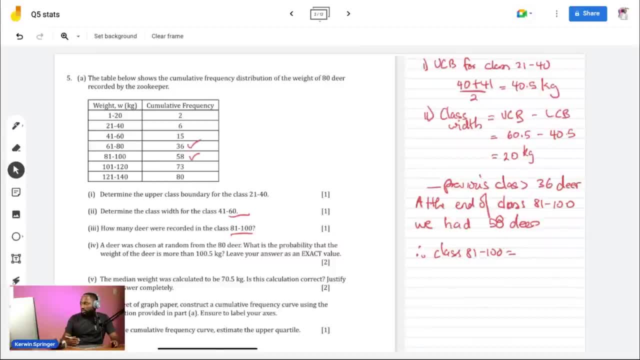 will have to be is cumulative frequency. So you subtract, You subtract. If your screen blurry, you need to go on the settings, the gearbox, and raise your resolution, raise your quality. All you're supposed to be of a generation is supposed to be able to figure out those things that 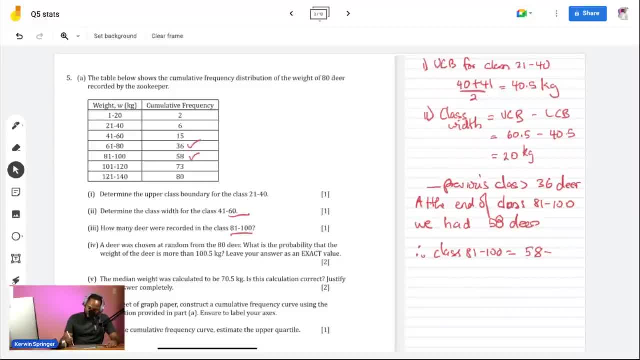 come on, man. 58 minus wait, it's 36.. 58 minus 36 now. So 36 here, 58 here, 58 minus 36 is how much. How much did I get 22 there? 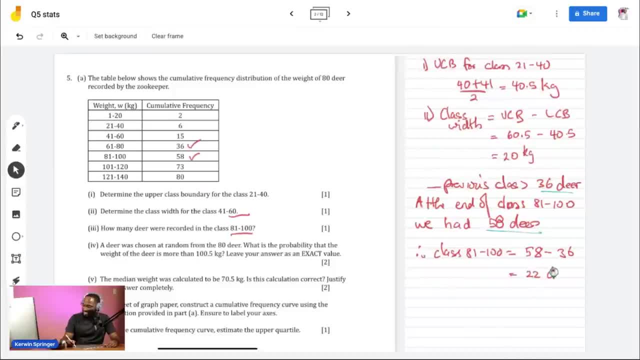 Oh good, I'll put in the units now. Look at all the units. I'm thinking now. Well done, So now I'm going to get all the marks in the exam for units. A day was chosen at random. A day was chosen at random. 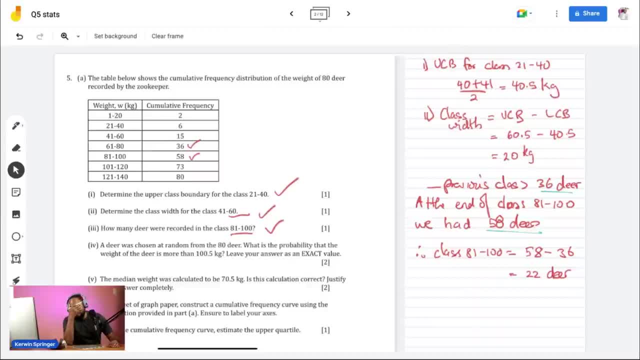 A day was chosen at random. I know they're going to make me make a cumulative frequency at Anyhow, these statistics class are going to inevitably have to draw a couple graphs and things. maybe some pie chart and things might come into this. 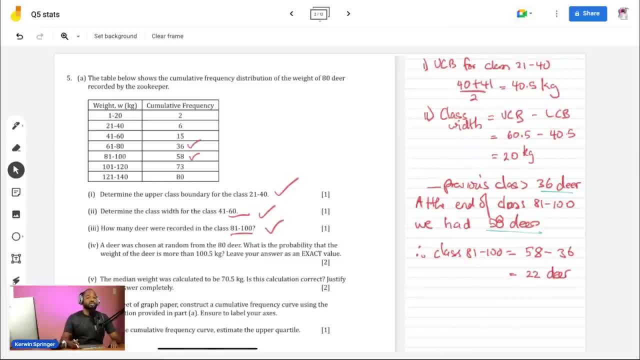 Saying that: see if you see the protractor across the way, because I'm smelling that pie chart from a mile away. Hey, you need that protractor to draw the pie chart. Those are like to go in the exam without a, without a. thank you. 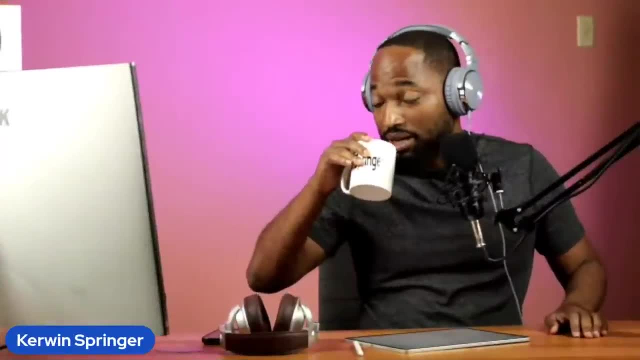 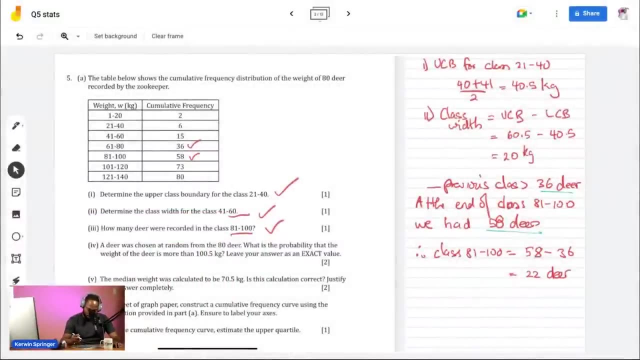 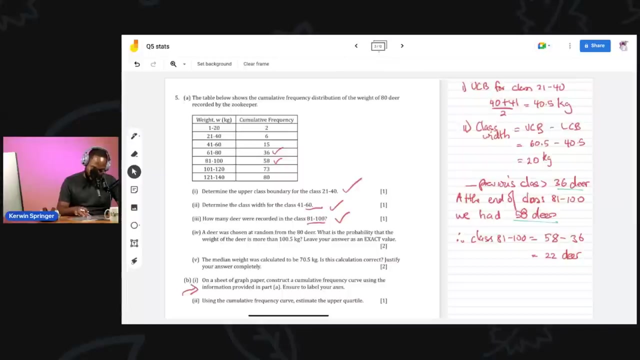 without a geometries, that you need a pie, a protractor to draw a pie chart. Number four: too much talk. Let me see if you can get number four all the way fast. Number four on sheet four. Yeah, number four on sheet four. 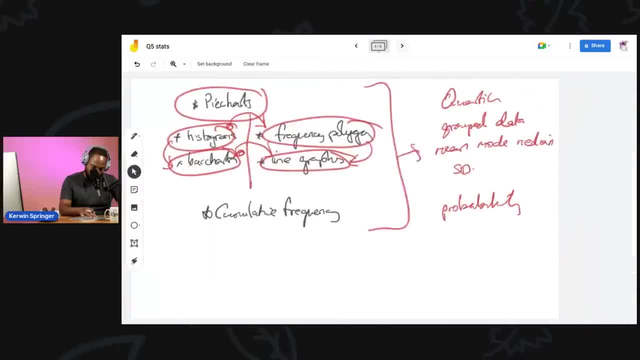 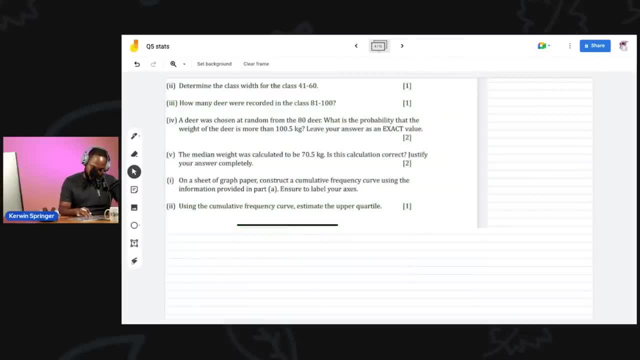 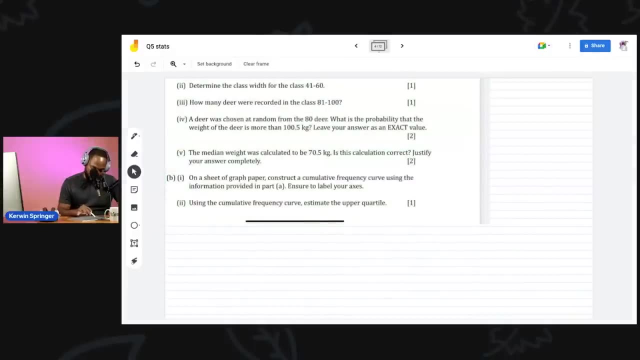 So a day was chosen at random from the 80 day. What was the probability that the weight of the day is more than 105?? Leave your answer in exact value. What is the probability that it's more than 105?? OK, maybe go back and see where 105 stop off. 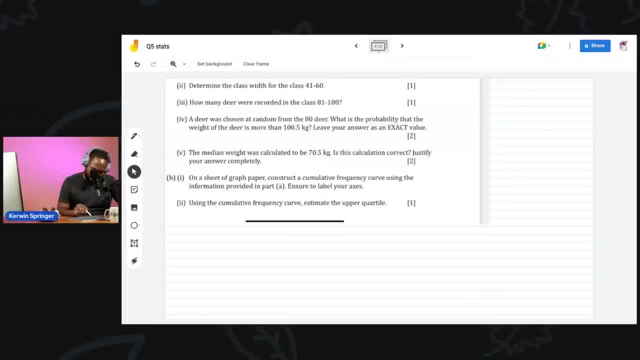 Is it 105 or 100.5?? I just reading things, 100.5.. So where 100.5 stop off? Let me go back to slide one and see where that really stop off. Slide two: that is that slide two. 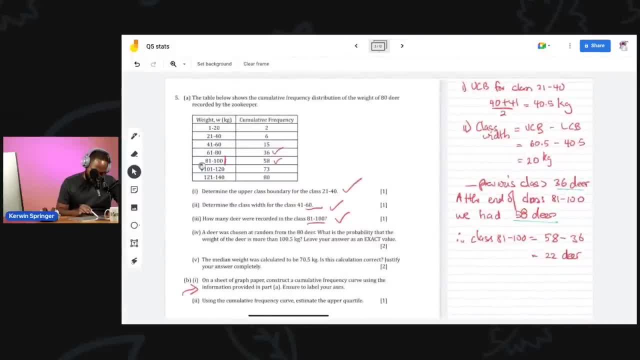 105 is here. That's after this. So what is the probability? It stop off at 58,, 58,, 58 people, 58 days, not day or whatever is the plural of day. So 58 day under 105, OK, 58 day or night. 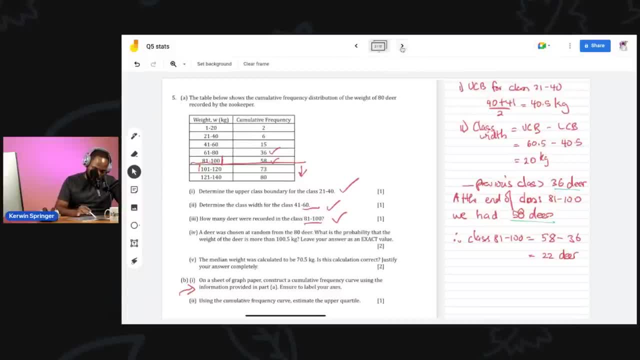 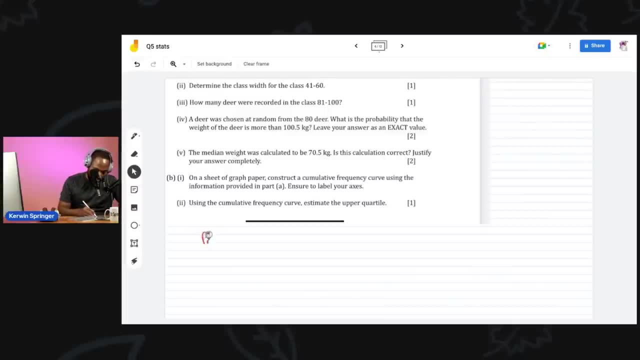 So what is the question? I go back to the question. There was chosen at random from the 80 day. What is the probability that the weight is more So? probability is the number of desired outcomes Over the total number of outcomes, And the desired outcome is 58 day. 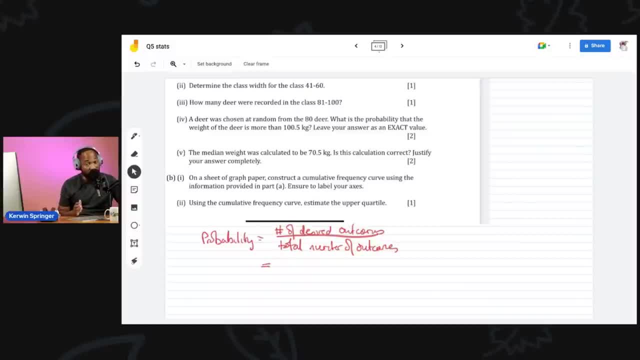 No, it's not. That's 58 day under, It's 80 day. also, The desired outcome is that there are 80 minus 58 day that are over 100.5.. And then What is the probability? And then, 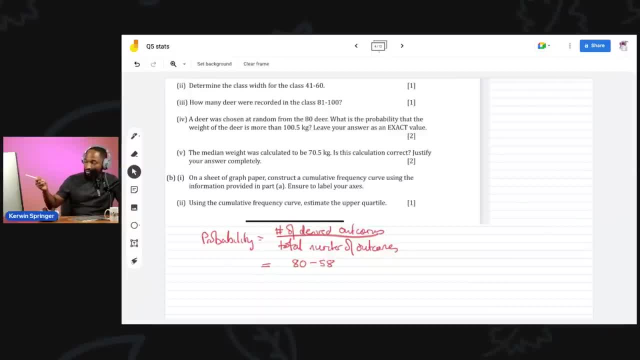 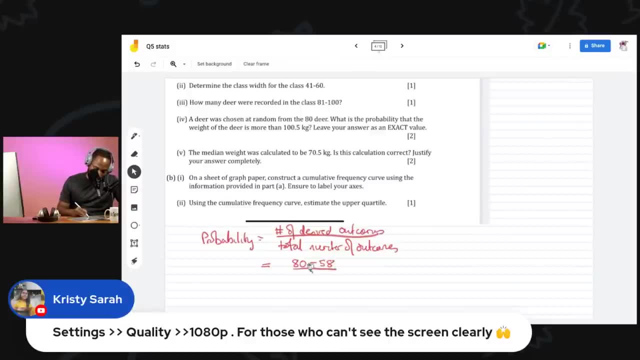 If you could just snap Christy Sarah thing onto the bottom of the screen for a little bit, And then we divide this by the total number of outcomes, which is 80. My calculator too, but don't show the calculator like that. How much are they going to? let me do this. 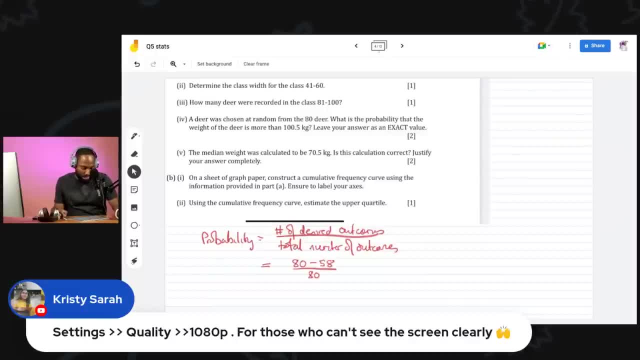 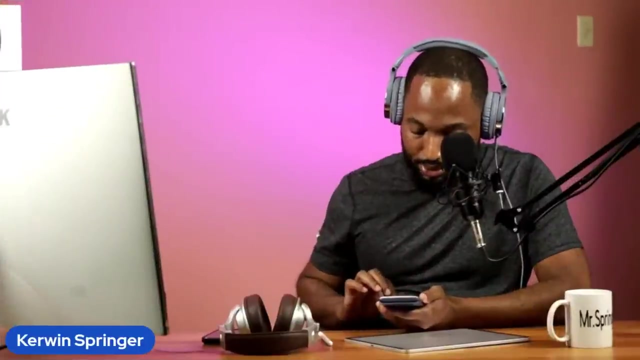 They did not see for? mean They actually probabilities? Why do, right now you jump in the gun, Thanks, So 22 by 80, which could break down to what 11 over 40.. So I might refuse to just think about that a little, a little bit. 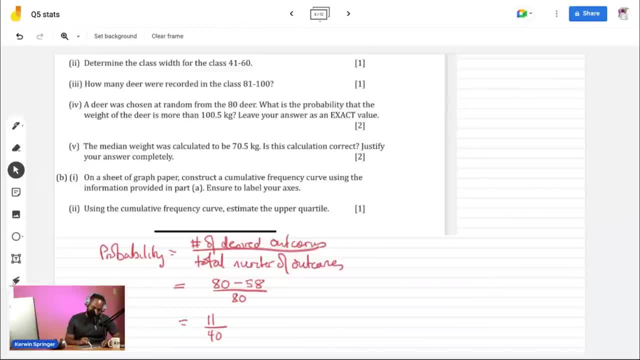 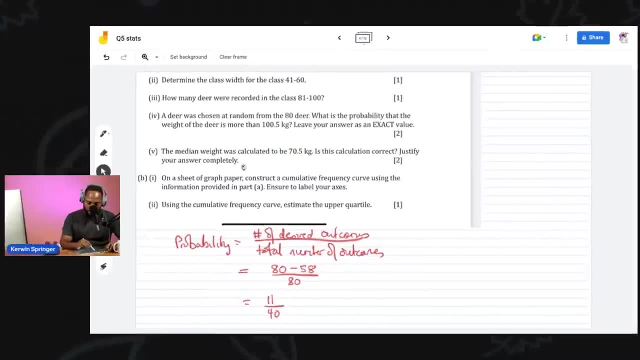 The median weight What It was calculated to be, 70.5, that in middle. Is this calculation correct? Justify your answer completely. So let's go back and use our expert decoding skills to see if that's something median ish. 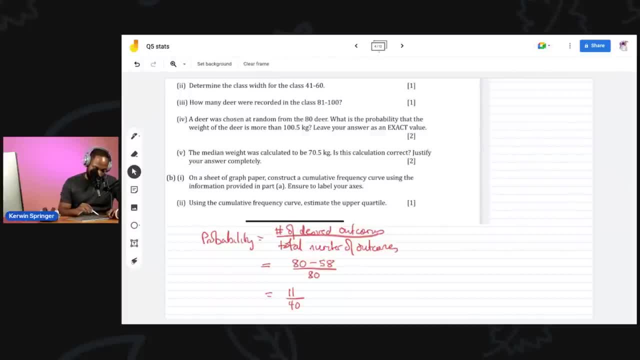 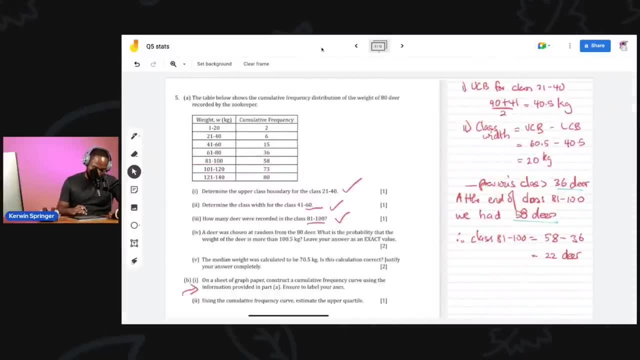 Let's go back to examine this um, this so-called cumulative frequency table curve thing. Wait, wait, wait. I want to just get it table by itself earlier and I'll pay it on a fresh new slide, Cause I feel like I need to see it bigger. 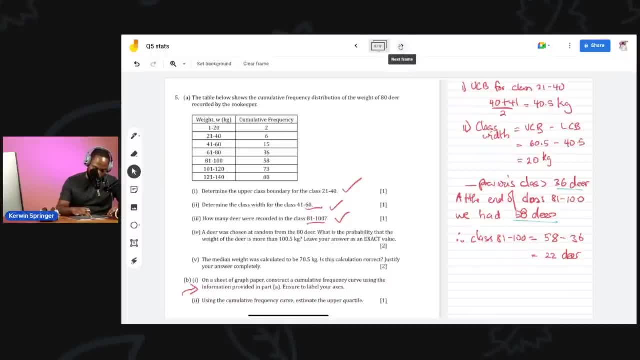 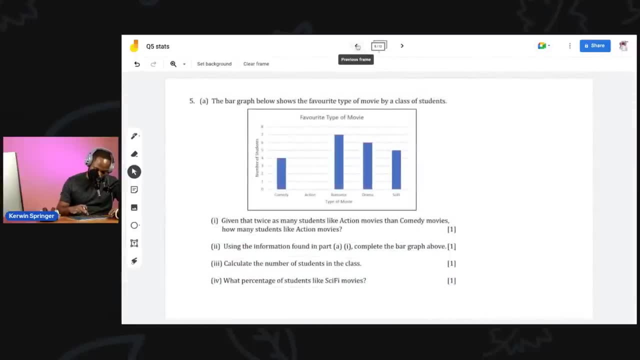 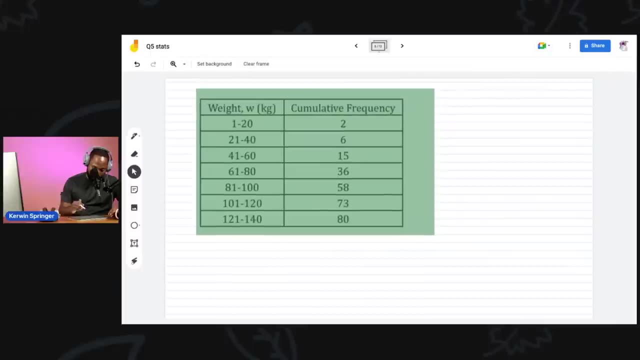 Okay, Okay, I need to see it big and it's small. So let me go on to slide five and slide five and we'll put that the table and we'll look for the median. So they say not in median is found immediately on a 70.5, right. 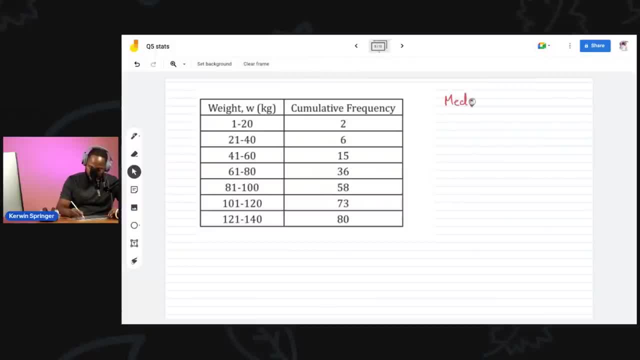 So it is suggesting that the median is equal to 70.5 kg. Okay, Okay, Okay, Okay, Okay, Okay. Now can that be the middle, Can that be the middle way? Now, what's the middle, The middle. you can just watch this and see the middle. two more: 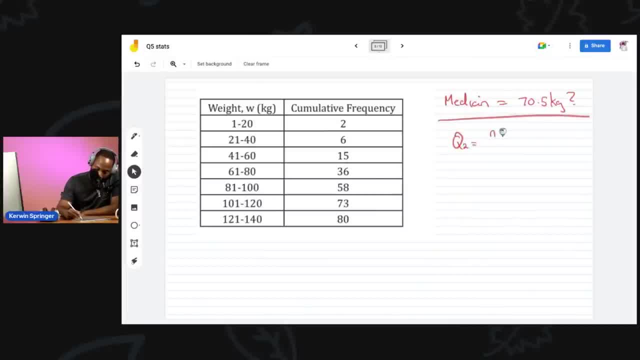 Q two is found by seeing N plus one divided by two. So it's really 80 plus one divided by two, which is 40.5 term. So this is where you'll find the median. Are you understand what we talking about? 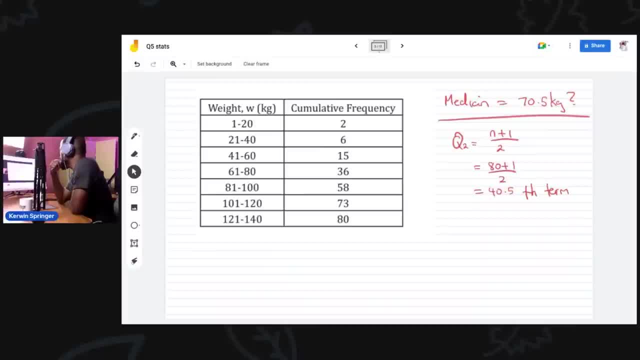 You say Q two, q1, all them kind of thing. no, that's something that some teacher, some students, bounce up to right before exam and like what in the world is that? when they bounce up to it like they have no idea that this existed. so let me just give you a quick little so you feel a little comfortable. 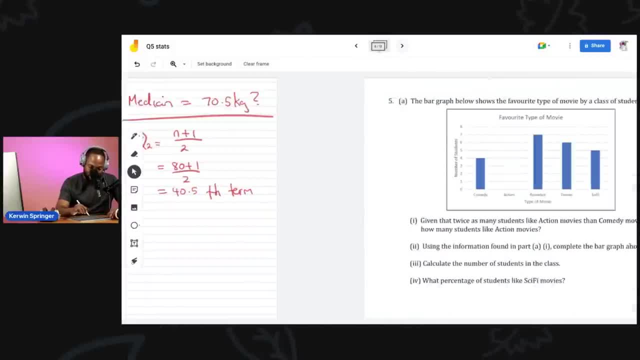 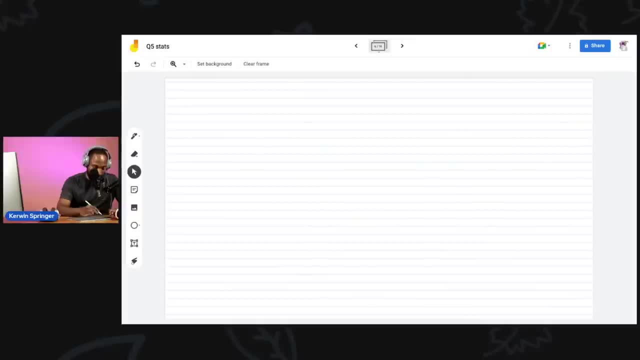 about it. now let me add on our next slide, again this question taking real slides um six and let me see what going on, right? so let me say i give you a bunch of data. i'll pay attention again. you're the mini, mini crash course on these quartiles thing. let's say i get a bunch of data. 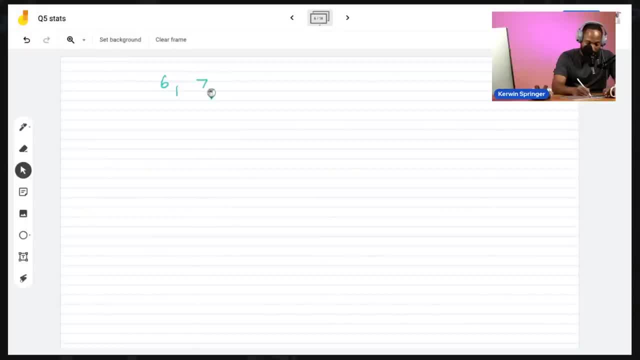 right, and i see one is six, one is seven, one is a seven, again one is eight, one is true 13. i want to go in order. one is 15 um one, two, three million um. one is 17. uh, one is 20 or something like that. one, two. 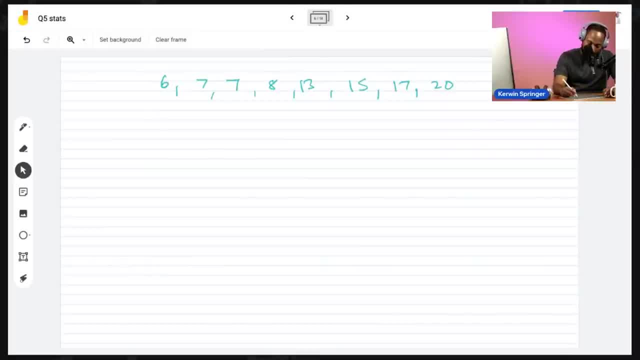 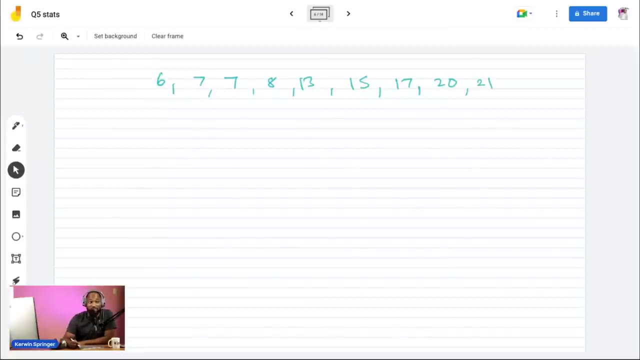 three, four, five, six, seven, eight, um, to make it nine, let's see it's 21.. okay, what's the middle value here? are they saying 21? normal are blocking? ah, are they serious? nice, nice estimation would be. so was he was the middle, was the middle the middle value? what? what is q1, q2 and q3? and thing really. 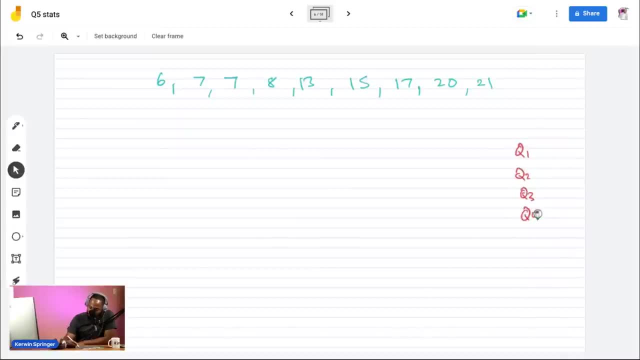 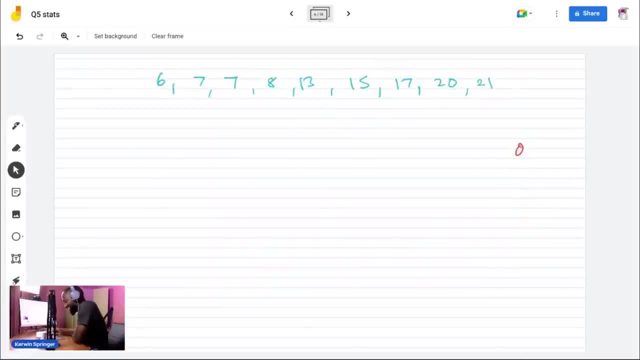 what are we saying? what we're seeing is that the middle value can be found using this formula. you could call it q2. that's the, that's the middle right, and you know this q2 will get a little more explanation just now by adding up how many values we have: one, two, three, four, five, six. 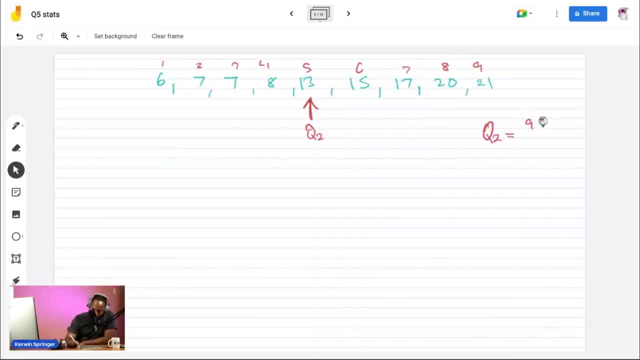 seven, eight, nine and say nine plus one divided by two. so it's ten divided by two. it's on the fifth term. ah, you seen it now. you've seen it now. this is the fifth term. the middle value is found at the fifth term. this formula works now. 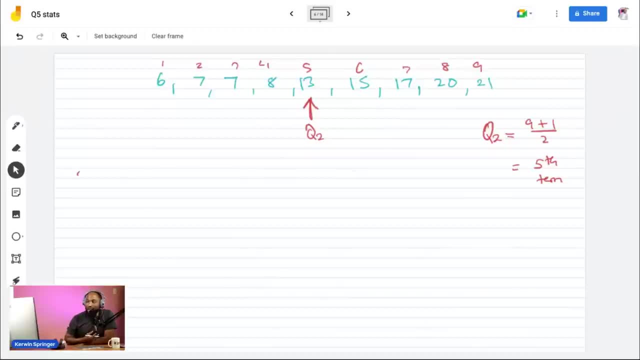 we add in one, because if you don't add one, you'll just end up dividing the thing by two. you wouldn't find the middle. find him. finding the middle of a set of items is different than dividing by two in it. let me show you what i mean. let's think about this like if i say two, four, six, what's the middle? 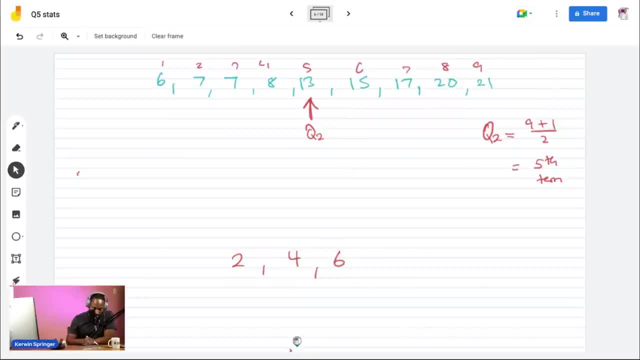 what's the middle number? the middle number is four, but if i say, divide the number of items you have here by two, you know where you're going to get. this is one, two, three, four, five, six, seven, eight. this is one, two, three, four, five, six, seven, eight. you know what you're going to get. this is one, two. 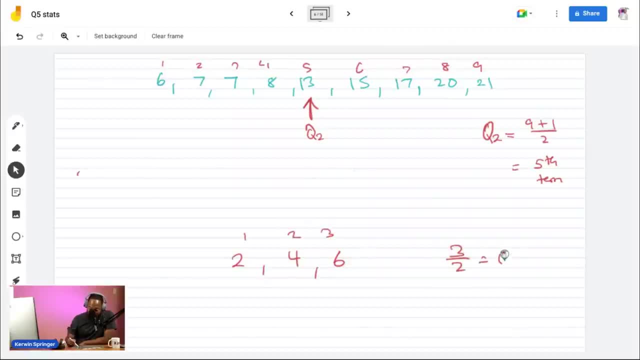 three items. three divided by two is 1.5, but the middle term is not. 1.5 is here. that's between these two. so you catch why we need to add the one in the formula. someone they probably never know why we add in one all the time. it's just how these things set up. fine, in the middle is not the same. 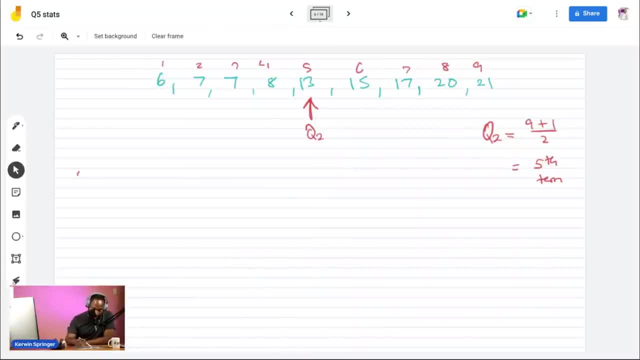 as dividing by half. so the middle term is there. you see, the step foot are we going to take is finding middle of the middle, the middle of the middle, if you're sitting a little better, if i don't put nine teams, like if i put 11. 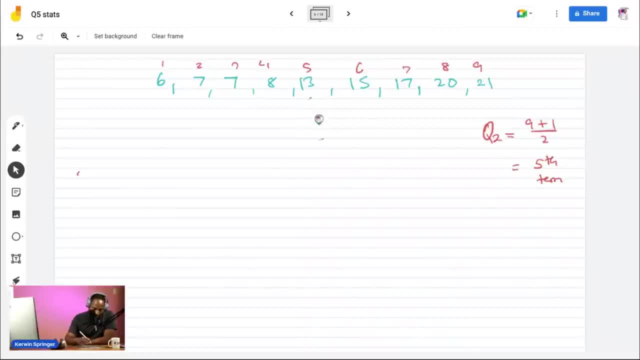 terms, you'll see it a little better, so let me bring them in two more terms here, all the way to 10, 11.. i don't want to get fractions in the example 24 and 30, right? so what's the middle term now? what's the middle term now? 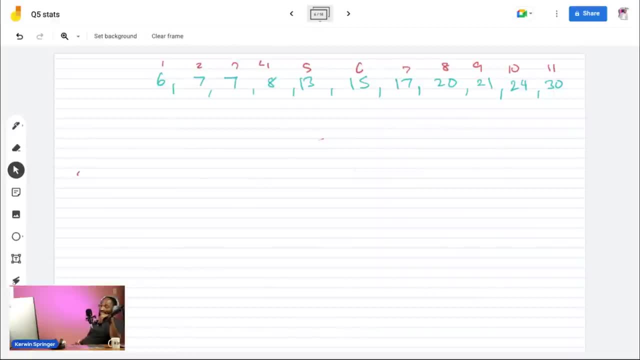 i'll hurry up, because this not suppose to last so long. what's the middle term now, if it's even numbers? Don't worry about it, Jonathan. Just follow these formulas. still, You will still get your decimal, but don't worry about it. 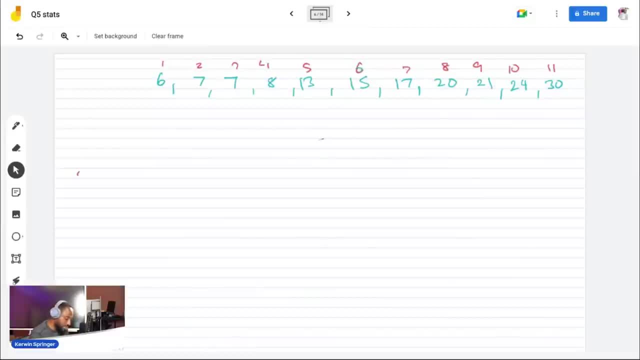 It's fine, I'll show you what to do. So the middle term is actually 15.. And if you cross, cross, cross, or if you say 11 plus 1 divided by 2,, you still get the sixth term. 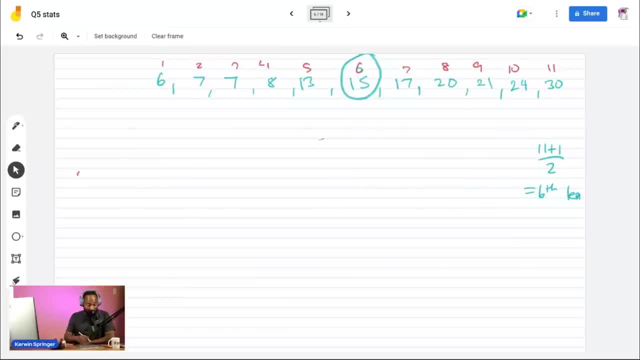 Six is not the answer. Six is where the middle term resides. It resides on the sixth term. That's very important to understand that little discrepancy there. So this is Q2, but if we divide this and you find the middle of the top half. 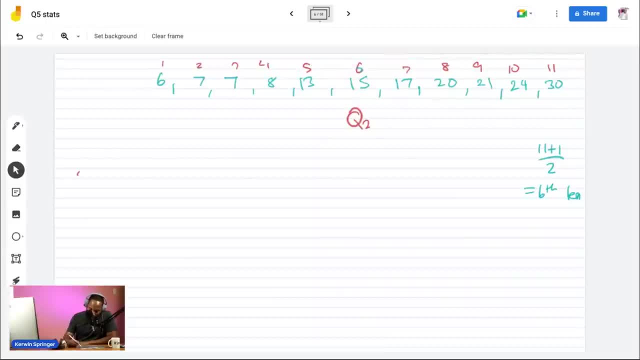 and then the middle of the bottom half, you'll realize that Q, this is Q2, right? Q2 is N plus 1 divided by 2, halfway through all the items, Q1 is a quarter way of the N plus 1, or N plus 1 divided by 4,. 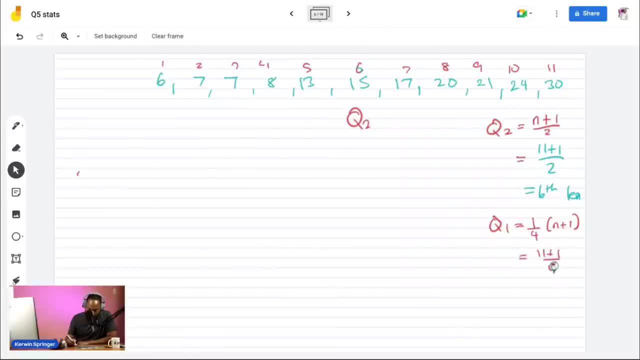 so, which is same 11 plus 1 divided by 4.. It's found in the third term, So you'll see that Q1 is Over here class. ladies and gentlemen, Q1 is that guy It's like. if you found this. remaining items here exclude Q2, you found. 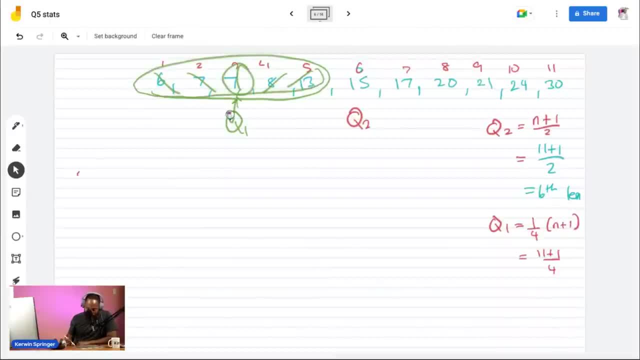 and you cross, cross, cross, cross. It's the median of the lower half of the data. So because- excuse me, because it's actually splitting the data into four parts, We call it quartile. This is the first quartile. 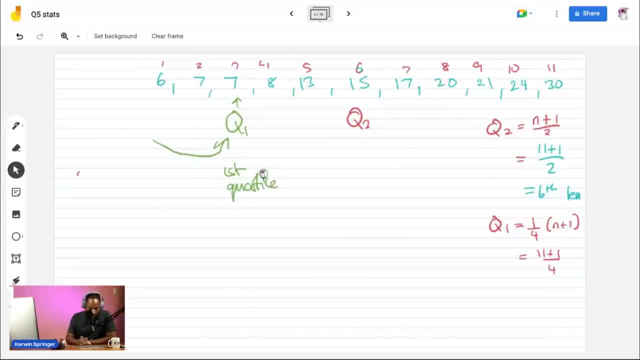 I see name out. This is the name in the arm. This is the name on his birth certificate- First quartile, But we call it Q1, outer road. Q2 is called the second quartile- That's the name on the birth certificate, but we call it the median right. 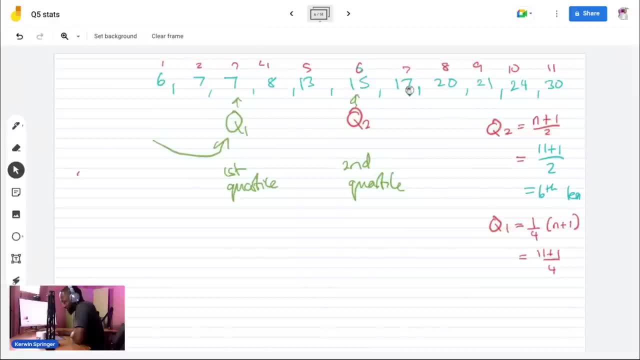 We call this the median, the middle, And then Q3 is. we'll get out. Q3 is this one, And the formula for Q3 is three quarter way of the data, N plus 1.. Oh, Oh, So now you know. 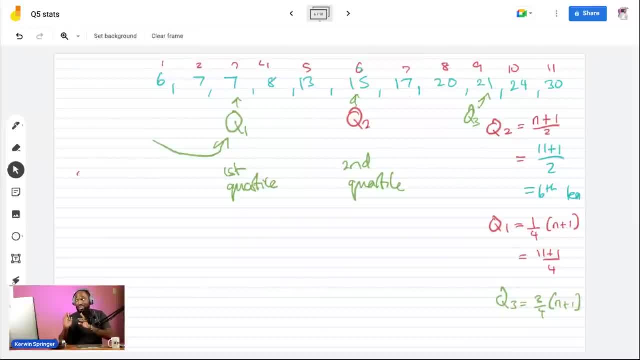 Now you know That's a quick little look into it, but you still need to practice it. It might feel like you know everything now, but you still need to practice it to get out the little rough edges. So the question was asking us: let's go back to slide four. 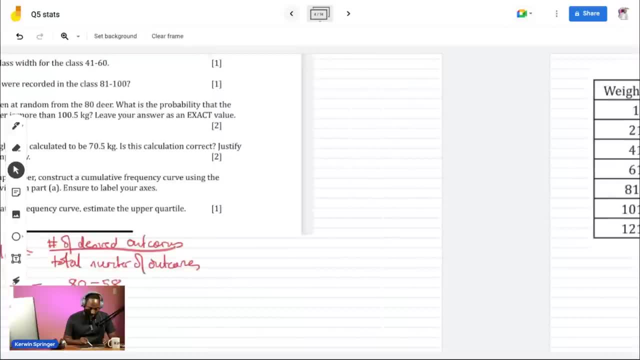 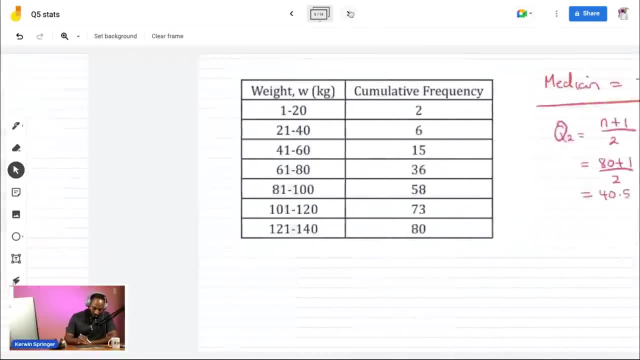 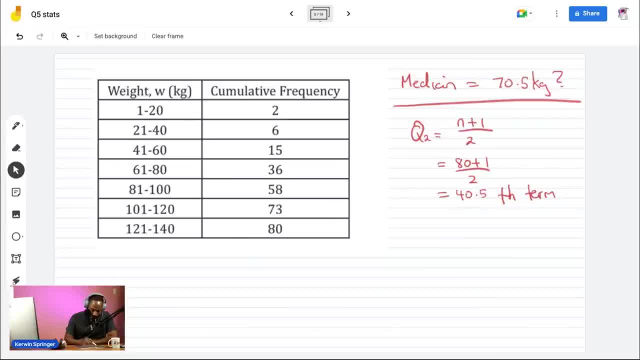 40.5.. 40.5.. 40.5.. Right about this. Righty, The upper class boundary of this guy. 40.5.. No, sorry, This is weak 40.5.. Where is that? 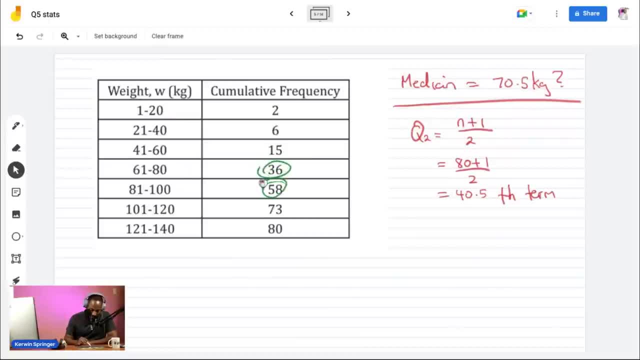 That's somewhere between this and that, Somewhere between here and there. You understand what I'm saying. This is the number of items going down. We have 80 items. By the time we reach here, we're going to have 80 items. 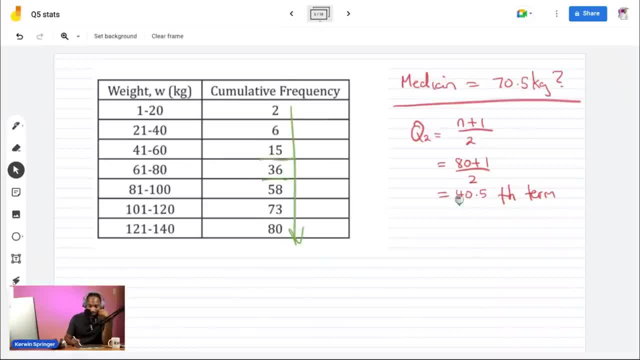 By the time we reach here, we have 15.. By the time we reach here, we have 36 items. I need to reach to the 40.5th item, The 40th term, And that's somewhere inside here bro. 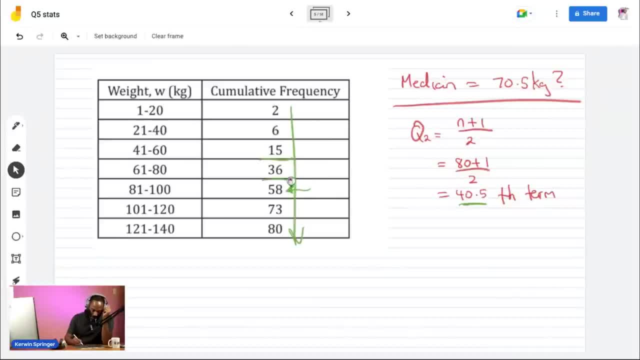 That's where that will come. So that means the median can be found in which class interval? It's found in the 81 to 100 class interval. Therefore, 70.5 kilograms cannot be the median. How would that be the median? 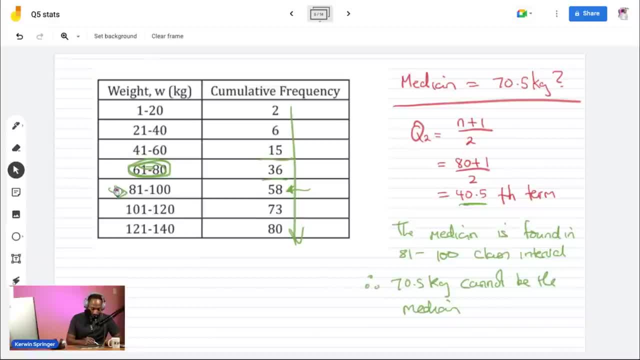 70.5. inside here The median ought to be a number between 81 to 100. And that's how you would call that. So they asked this really recently And they asked this like about two, three years ago, And they keep asking this every four or five years to look out. 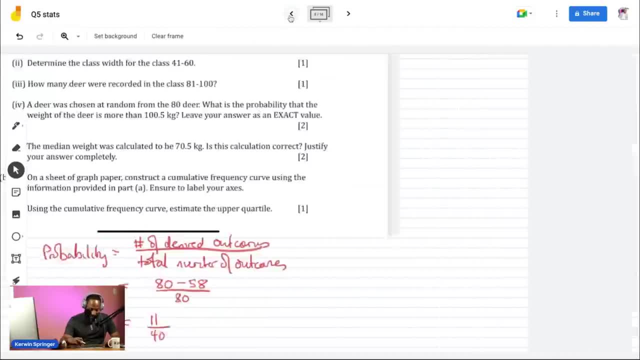 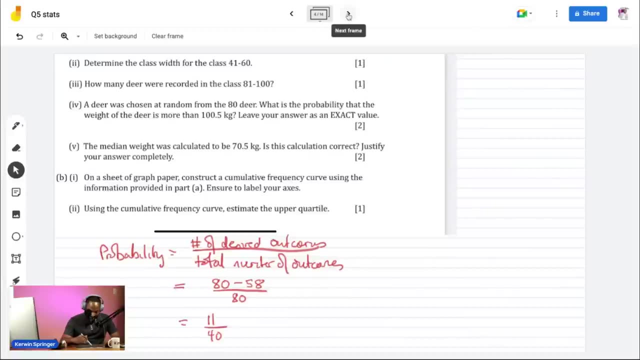 This question is taking real long to finish for you, Joseph, On a sheet. And now I need to go and Construct a commutator frequency. Go, use any information provided. Ensure to label your axis. Liza holds it at max. 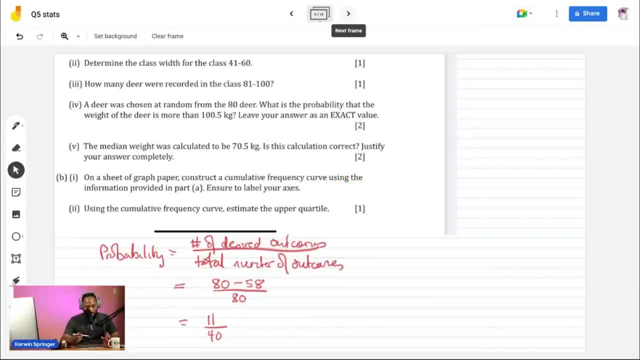 But this is not the way. question five comes right now. It only comes for nine max, But they could still ask you to draw the curve. Use the commutator frequency curve to estimate the upper quartile. So I want to take this table on page five. 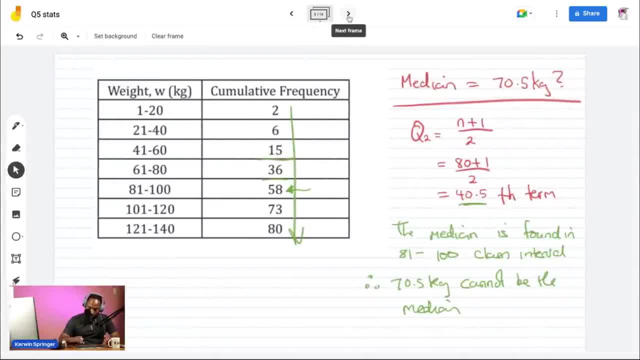 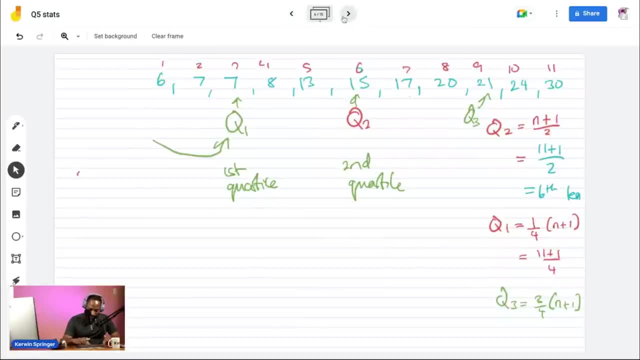 and draw a commutator frequency curve. So I'm going to copy back the table. Let me see if I can do that. I want to copy back the table. Yet another slide. I'll stick in by six there And see if you can find a background that have a graph on it. 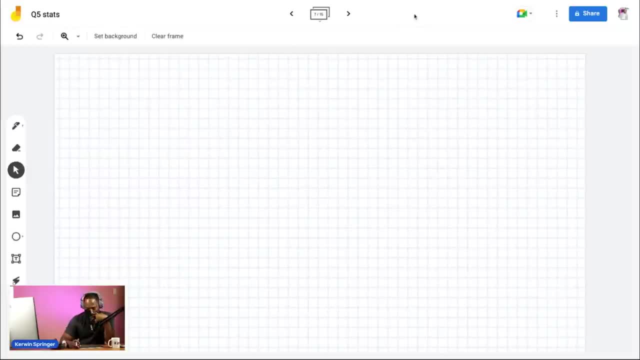 Is that one And right Graph paper. Now I'll put this here. I just want to give you all an idea of how it works, How to construct. This is not how the CXE graph paper looks, So that's a little unfortunate. 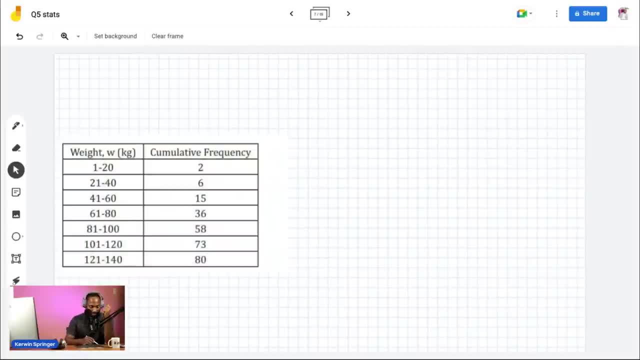 But we can still, We can still fight. You see, CXE graph paper has like five and ten. It's like a block of five and then a block of ten. So but you'll catch the idea. So we want it to go up to. 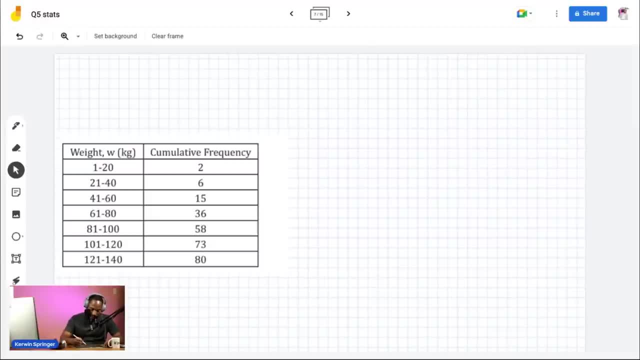 We want it to go up to 80.. So this is on this side, on the y axis side, And I want to try again with the ruler, the long ruler. So The y axis needs to go up to 60 and the x axis needs to go up to how much? 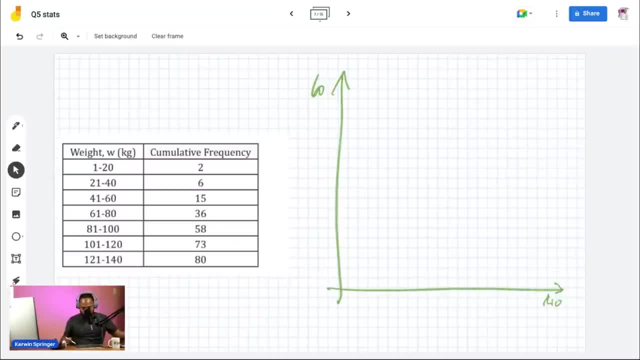 One hundred and forty. So I divide my stuff accordingly and I will see. I'll see. So somehow, when I draw any ruler digitally, it still come out Ben, I don't know what is that. Oh, this time it come out straight. 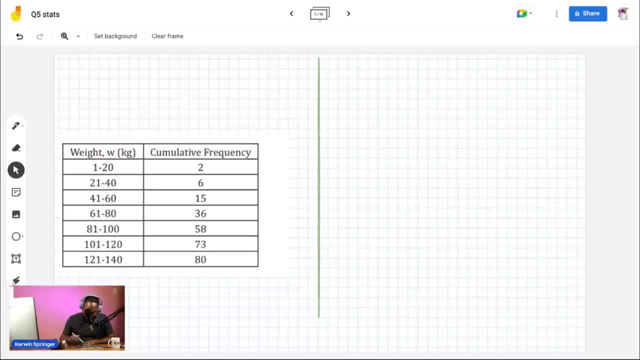 And then Let's stay by and watch me do this. If I take my time to do this, I will do this video And then, OK, so let me see 10, 20,, 30,, 40,, 50,, 60,, 70,, 80,, 100, 90,. 10,, 20,, 30,, 40,, 50,, 60,, 70,, 80,, 90,, 100. 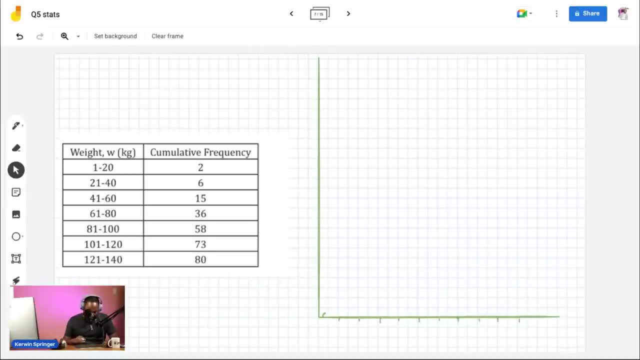 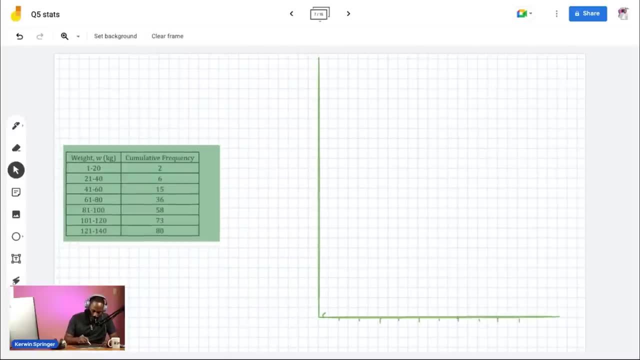 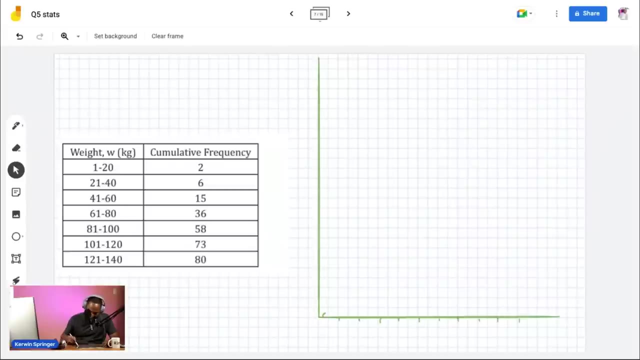 Can I make one hundred and forty? Huh, I really want to make one hundred and forty. So I'm going to do Pull this back like this And hopefully what I'm about to try here would work. I'm about to. 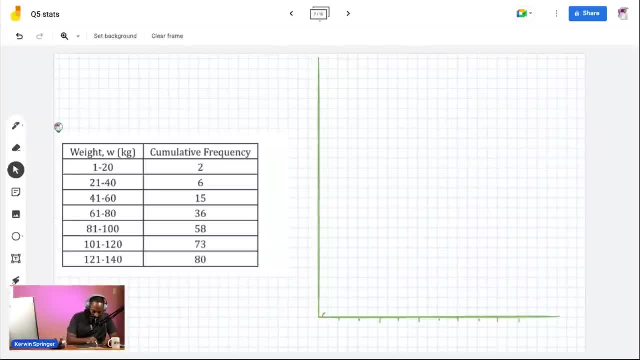 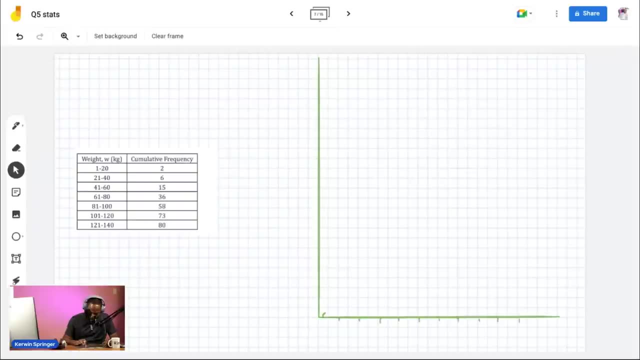 Try and then move, move, move a ring. Let's make this smaller And let's select this And move it. The stress is alive on this boy, Ray, So move that in. You come back. Yeah, Yeah, Yeah. 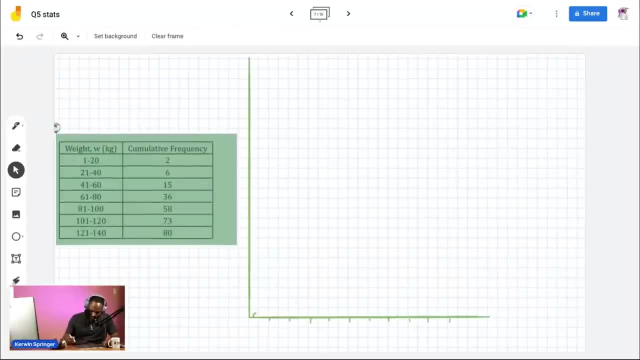 Yeah, All the scenery Nice. So now they want to double up. I didn't want to double up, I'll. you can do them thing. I can move the graph and you can. you could try it on your paper and think when you draw the graph: 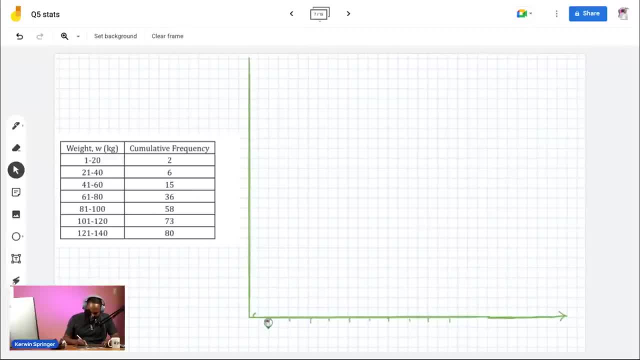 If you could pinch, zoom it, and So 10,, 20,, 30.. So make sure you plan ahead 40,, 50,, 60,, 70,, 80,, 90,, 100,, 110,, 120,, 130 and 140. 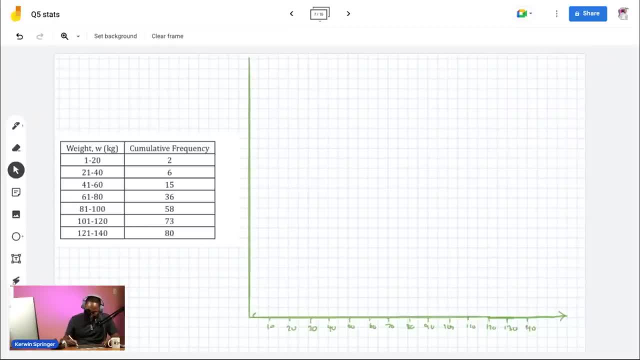 Looking good. so you write your thing one time. this is your weight in kg and this is your cumulative frequency. here you write out fully cumulative frequency, then you write number of days or something. you just want to have a label for everything, and this needs to go all the way. 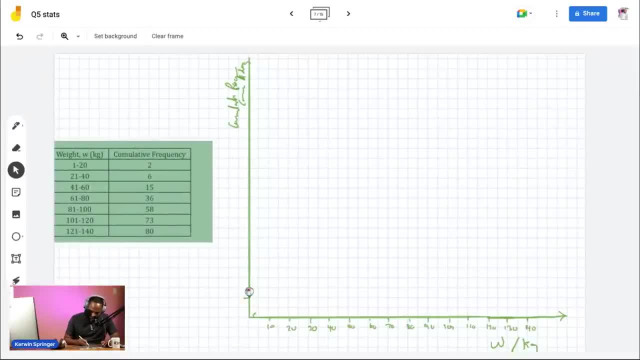 up to 80. i feel like i do the same 10 20 thing, 10, 20, 30, 40, 50, 60, 70, 80. so what you'll do here is write your scale and you write like one centimeter is equal to. in this case, let me. 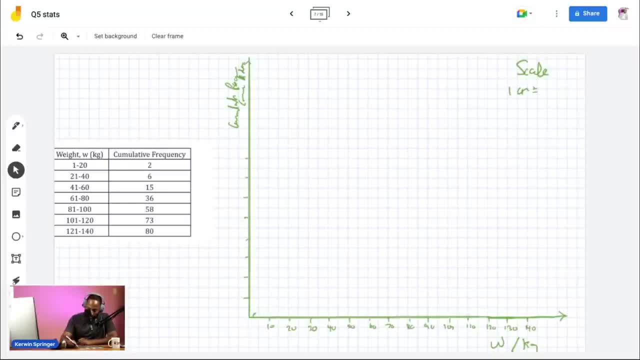 suppose this was one centimeter. so one centimeter is equal to 10 kg. and you put x axis- why isn't you understand how you do the scale? and i put y axis. um same thing for one centimeter equal 10 days. so that's how you secure the bag. that's how you secure the bag, all these little. 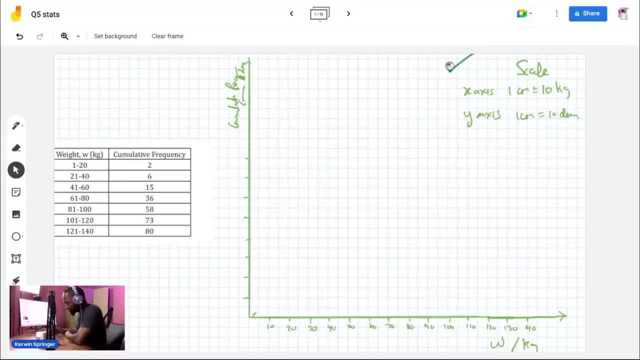 these little tricks and things showing on here. so what's the next thing i'm missing for this graph? so the scale usually goes up top there, but i'm putting it a little on this side here because i feel like my graph might end up in that zone. oh no, it could, it could, it could be actually. 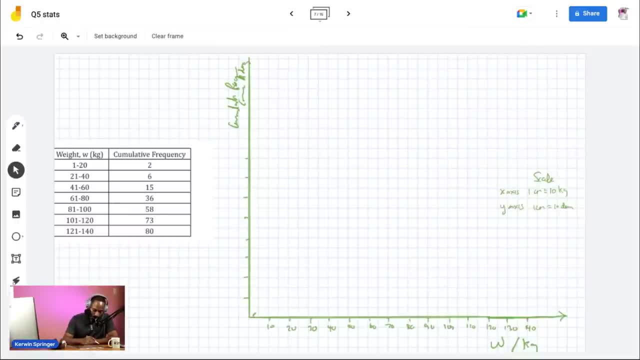 it could be. the next thing you usually put is the title. so you have a little title, title, the right title, right, some people, let's be taking four minutes something to figure out what to try to write for the title. just write graph of cumulative frequency versus weight and you're right. you. 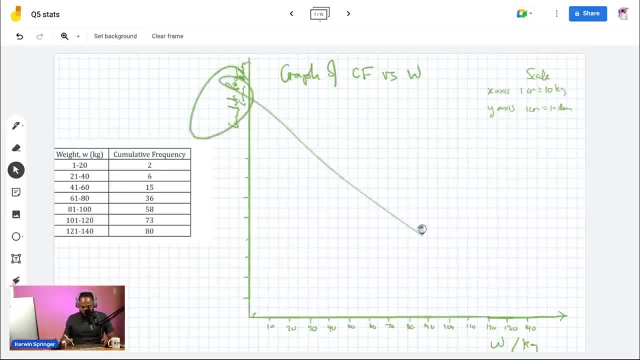 spell out those words: graph of this versus that. that's what you do for everything: physics, maths, add maths anytime you need to get the title of a graph. don't overthink it now, man: 10, 20, 30, 40, 50, 60, 70, 80.. so so far, so good. so far, so good. and then um time to plot. time to plot with a little. 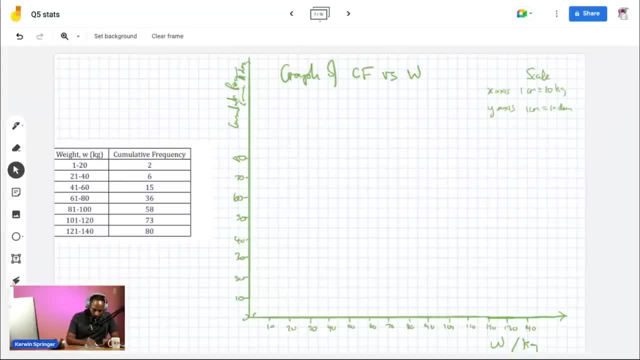 cumulative frequency. now, when you're plotting cumulative frequency, you don't plot no 20, you actually need to plot the upper class bound. you say plotting 20.5, so it's actually 20.52, so 20 is here. 20.5 will be a little smudging off, so it's kind of a seat in the graph is going to make. 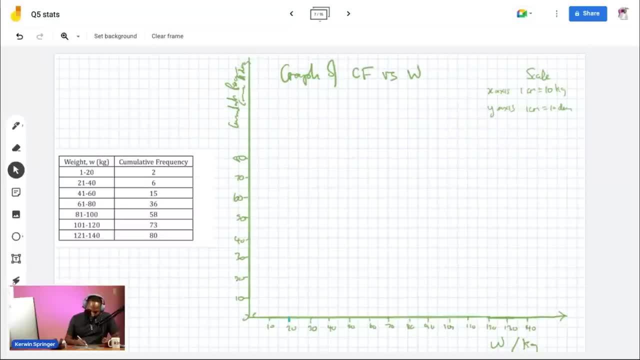 it going right a little bit off. some teachers just make you put 10.5, 20.5 here. i'm not about a life, i find that kind of clumsy. i would just move the point a little bit. and two, two is like real low down. so the first point is valentine's and purposes we can put him like about this one. 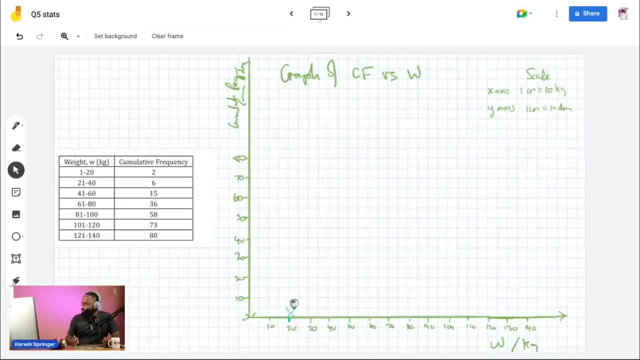 earlier about this. one, yeah, and 40.5. you understand what i'm doing right is 40.5 and 60 and 60.5 and 15, so i'll already do the 20.5 and two- it's hard for me to write a point on this- 40.5 and six, why these things are a bit scraping the. 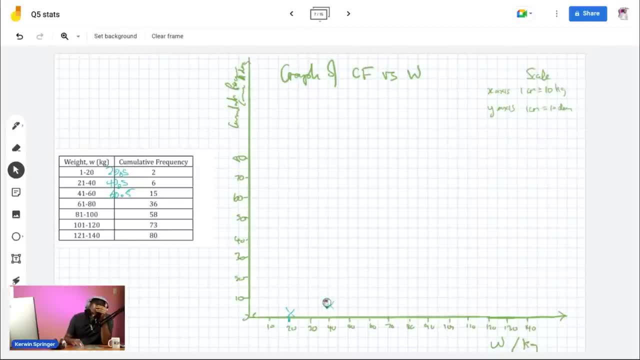 bottom of the barrel, so by 40.5 and six. so that usually happens in a cumulative frequency. it starts out slow and then all of a sudden it's scoot up like this: what's your legacy? 60.5, 15, 15, non-starting to 60.5 done, starting to feel like you want to. you know, experiment um. 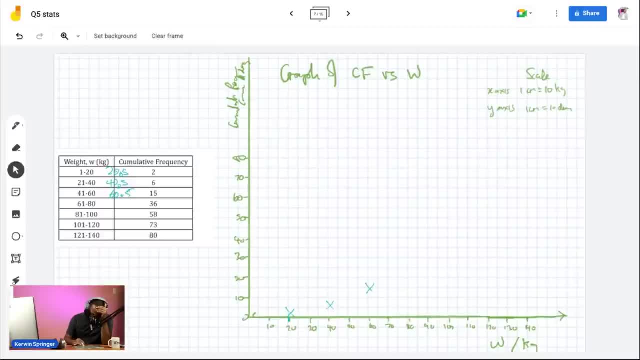 1x. oh, 80.5, 36, 80.5, 36, 80.5, 36. there we go, there we go, we make expansion: 80.5, 36 somewhere around there. so 100.5, 58, 100.5. oh, that 80.5 in the wrong spot. 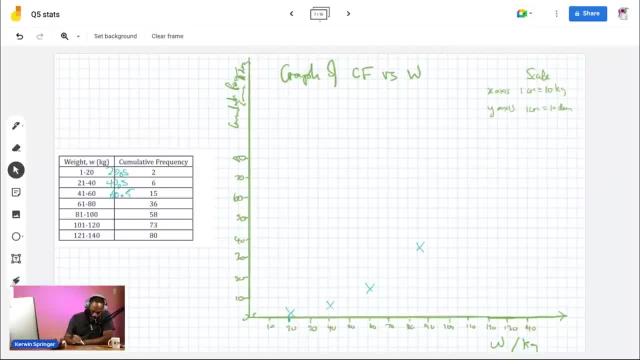 fortunately, i could just select it and drag it across. so come across. so there, bro, like that fine. and then 100.5 36, 100.5 58- i read this exam in 2005 and i really do not need to be doing this- and then 120.5 73, 120.5 73. 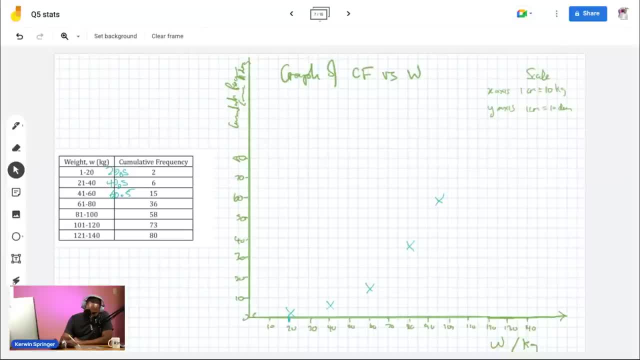 must be around this. so and then you had a finish off strong, it's good off my pen too enough. how long this battery looking to die waiting diet every time when you come in this class. so they must pray this man battery don't die. so if i go in straw and then 80, 140.5, and then you connect, then you connect. 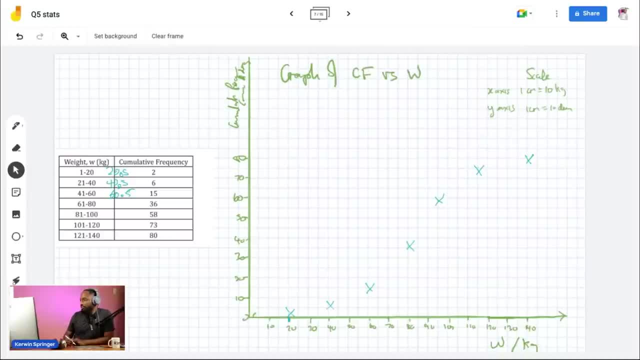 how are you looking? it's actually looking pretty good. on my screen. all you find out: looking pretty good, looking pretty good. so then we are a little so so, but it can't be so, it can't be so. it can't be so shaky. i need to be smooth, but it kinda. 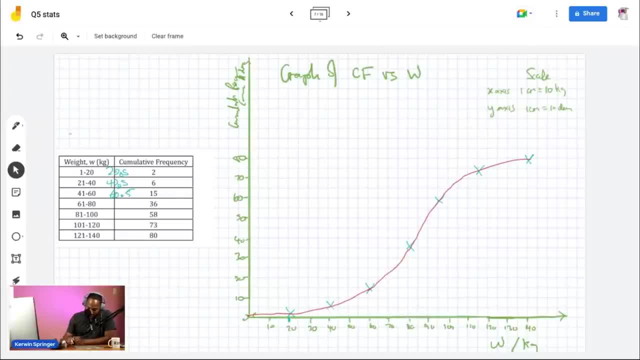 hard to do on an ipad. and that is you day graph of thing against thing. blah, blah, blah, blah, blah. every everything look like your expertise and i wanted you to use the graph to figure out um, estimate the upper quartile. this is what you're looking at, and then you're 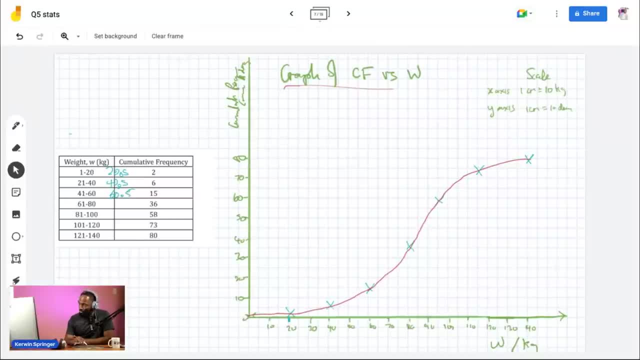 do to estimate the upper quarter? to estimate the upper quarter, they go back to the graph and they do the same thing. q3- remember the formula i gave you- is three quarter of n plus one. that's the upper quartile. three quarter of n plus one: a three quarter of 81, 80. 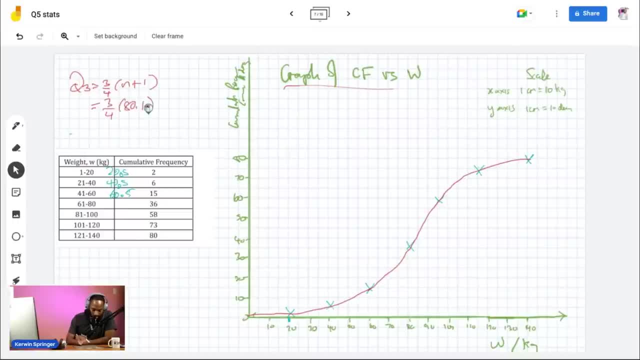 plus one. at the end of the day, you know some kind of 60, 60.75 something, so. so what you're gonna do is take your ruler and come across from the 60 just a little above 60, because it's like 60.5- do a little dashes thing, touch the, touch the grass, hold on. i didn't show up in this, just. 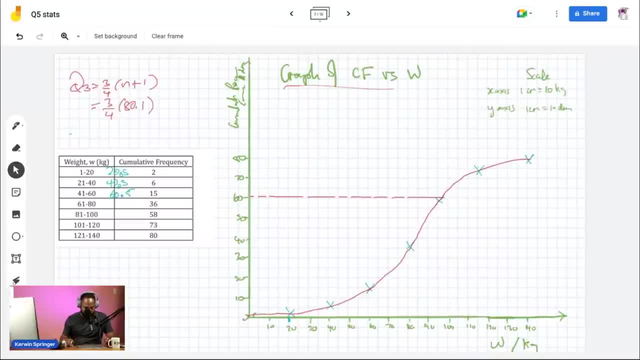 now i'm gonna make sure the estimate, the upper quarter, yeah, yeah, 60.5 on the cumulative frequency that is. and then you come back down here like this: on the, once you touch the graph you're bringing background bang. you could even battle r if you were and you read over there. 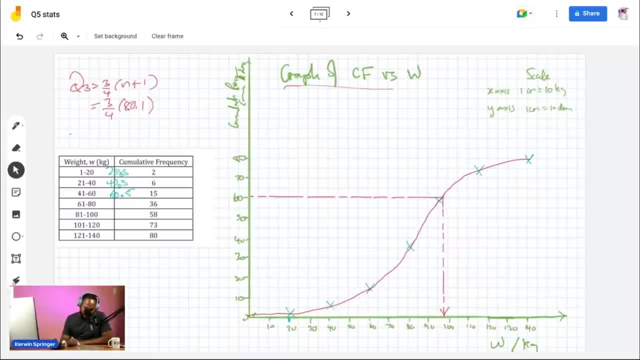 how it looking. nah boy, all you can see: 100.5. they're looking like 97. so the upper quartile, therefore q3, is equal to 97 kg. now hold up, you see. all right, this here i should put equal to the 60.75 or something like that too did i put 80.1. sorry, my body should be 81.. 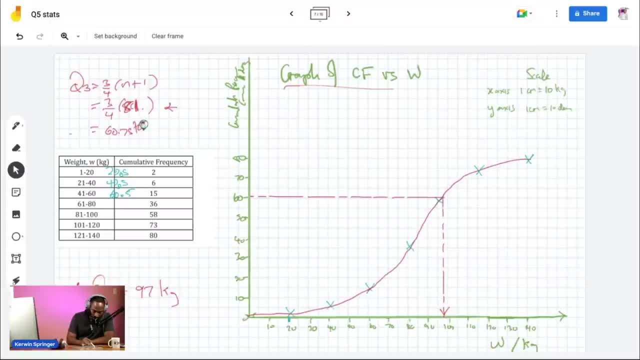 and this is the 7.60.752. and then you have per q on like this: 120 was wrong, i fed upon. now, if all you want to see the accurate diagram for coming later. if you're frequency, go and switch up coins, bring a community frequency. but to be honest, 120, 120 or 120.5. 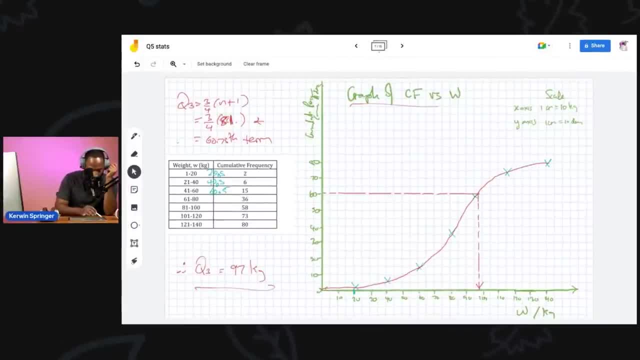 in the wrong spot, he correct. oh boy, let me just sort that out for the perfectionist and them how i'm missing it so by earlier. it's just how i had to zoom in. let me zoom. i'm so sad about missing this. both of these wrong. 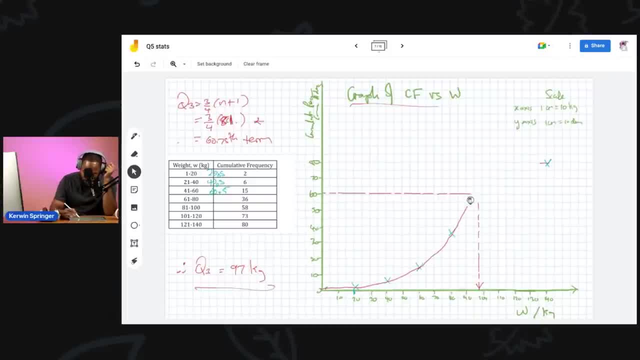 so what we're seeing is this man put the wrong graph here, boy. so it was. it was 100.5 58, 100.5 58. drawing it, 100.5 58 is about here. so 120.5 seven 123, 123, 120.5 73. 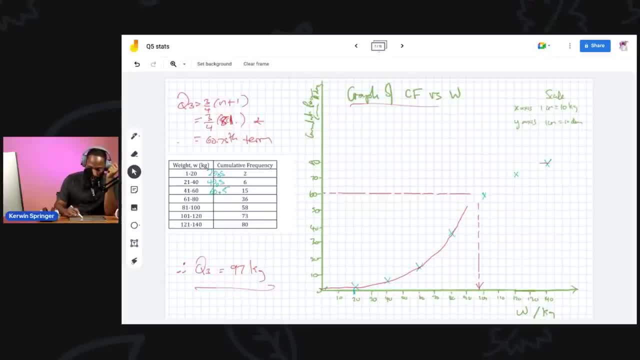 yes, check that now. so what happened is that i'll have seen my whole screen. but i have seen my whole screen, so i started watch the access and then follow it back up, so something might get lost when i'm doing that, like i'll fall into the next line that way. um, so this: 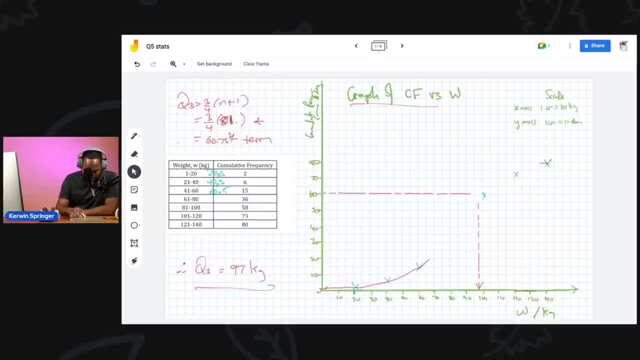 was 80 point. the next one was 80.5, 36.. five thirty six like this. so let me just accurate this graph a little more. fix the accuracy on this graph. it will actually change my answer for this, for this, for this thing here. sixty. 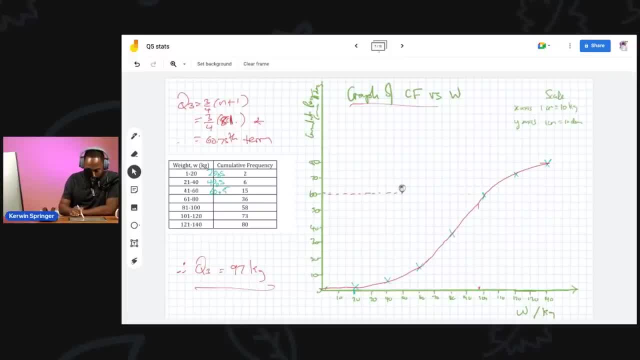 point five would have come almost like this. sixty point seven five touch the streets day and come down like this. so the person who say a hundred and about 105- that was that was actually correct. it's like 103, all right, so why is that one? you can't get fed up, so 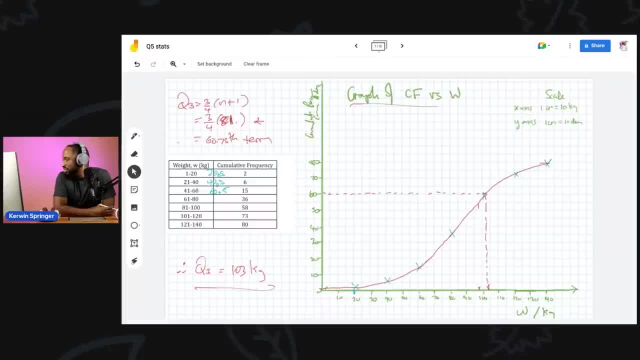 you put it. that's where i think you come in with the frequencies, right? yeah, um, this is another question. is that quest? so let me just state over what was the issue so that everybody will be clear about it. see if i could get a highlighter here. the issue is that the, the cumulative, 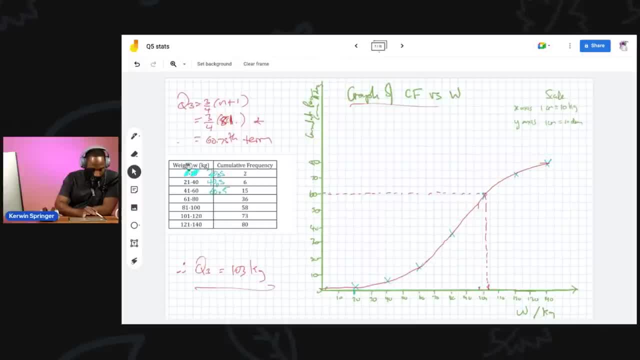 frequency doesn't plot with the 20 or with the one or with the middle. it plots with the upper class boundary. so i need to plot 20.5 on the x-axis with two. so 20.5 with two, then 40.5 with six- see now- then 60.5. with what? if i plot with, then 80.5? 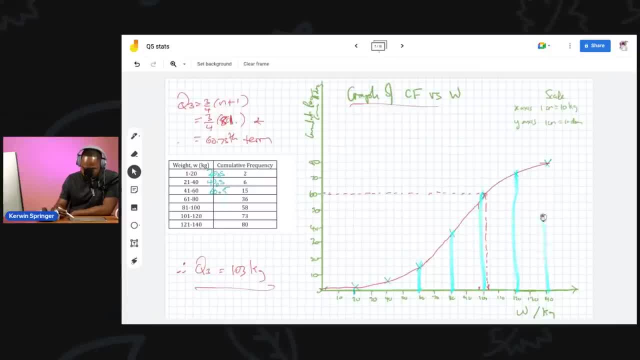 take one hundred point five, then 120.5, then 140.5 and you plot it really corresponding y value from that class interval that it represent and it will get this kinda s looking curve right out of 10. how much you understand this. just look up k overstring our cumulative frequency. 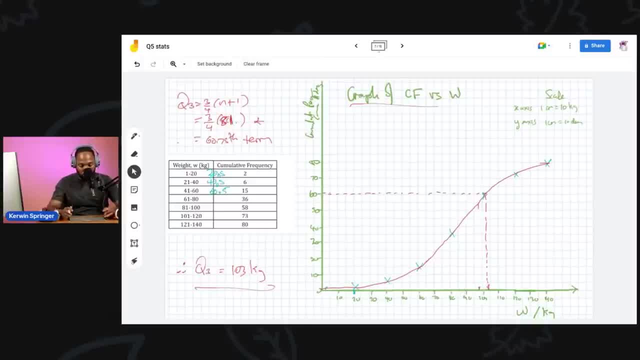 for a full nice in depth left lesson on it and you'll get to see me drop the graph hunting again. so the next community frequency curve graph. i have either recent retreats or might skip it, right, because you see, take something i'm saying somewhat different, right maybe? i'm going to go with s, and that's my thing, because i'm prepared for this problem. but looking for something is nothing. and have heard this. it literally comes up and just blurt th ExploGraph and once you leer gara nuevas tenguin naucen tube graph and the 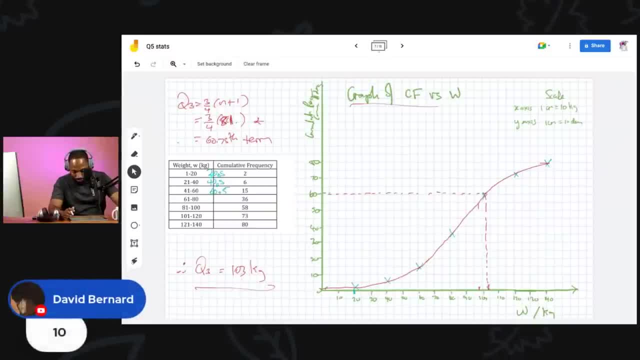 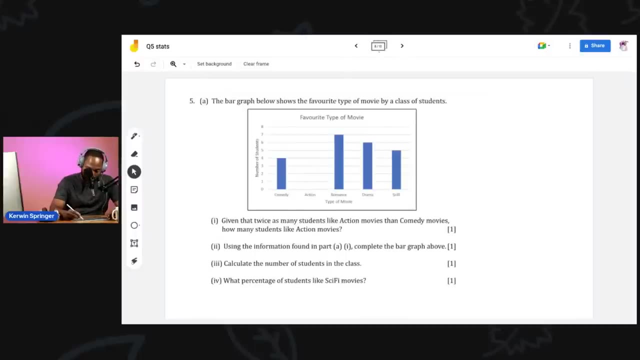 time. all right, new number five. the bar graph below shows the favorite type of movie by a class of students. given that twice as many students like action movie, non-community movie movies, how many like action movies? so how many end for the action way? can i write really highlighter? 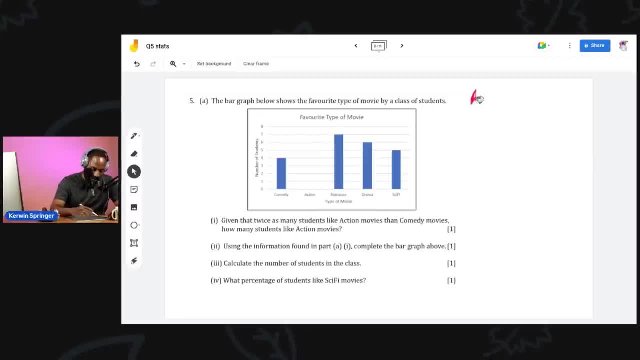 so you need to read off. i love when they bring bar graphs. i like free max. so action movies would have to be two times four, which is eight. students, how come i didn't answer this one yet? students, so you have a little issue with these kind of questions sometimes. on this they might. 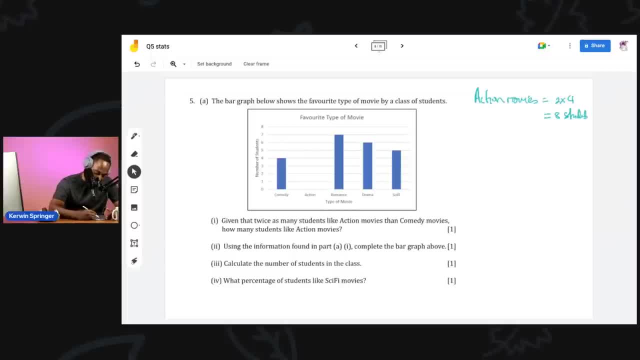 have number of students and these people will put in a little sneaky little brackets here: hundred of students. so you think you could just write four. this time you had to write 400 or 800, okay, so So action is twice comedy. so that's what i know is eight. it really need to go up like this touch. 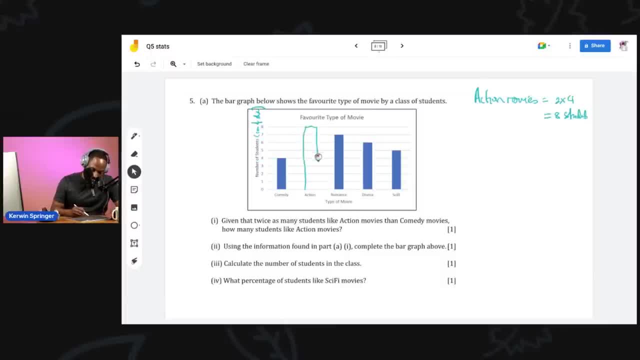 it. get a little bar and come back up using the information from my path a1, complete the bar graph. we did that. you're supposed to use a ruler and thingy and if you had a shade hatch, um, calculate the number of students in the class. number of students in the class, total number of. 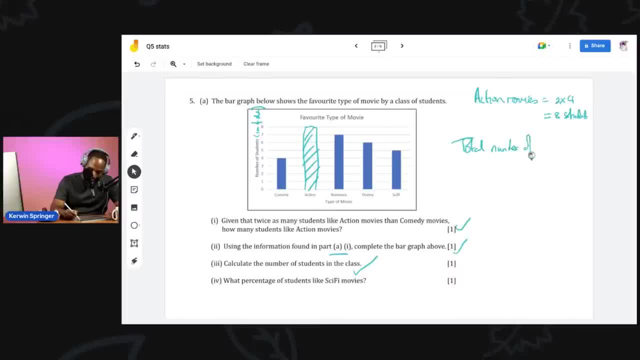 students. so what i do is i usually come out with pencil and just write the number of students in the class, number of students in the class. then i'll select this circle over here and i'm gonna tell the answer, and we're going to have to try and get it right. just write four, eight. 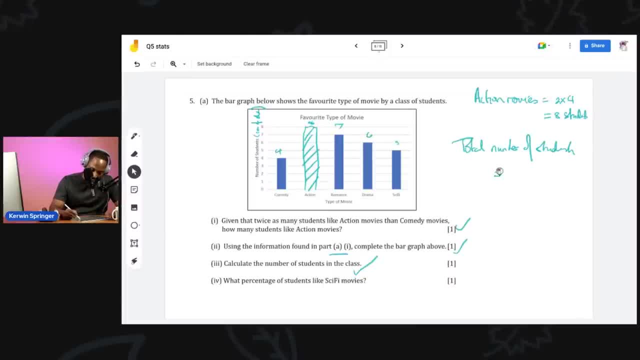 seven, six, five, just to make sure. so four plus eight is 12 plus seven is 19 plus 6 is 25 plus five is 20 students and what percentages are students like? i wish this question come earlier. i'll pray for this for their boy. so percentage? 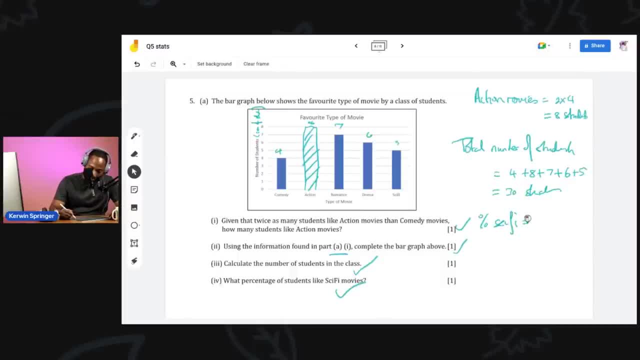 Syfy wтом 30 students would have to be 5 over 33. I'm sorry, but geez, wow, god. he cost me whatever for hours. that's all I can afford. I'm fucking. And the rest of them are people that are assuming to use hate than for the other two. Heritage member. 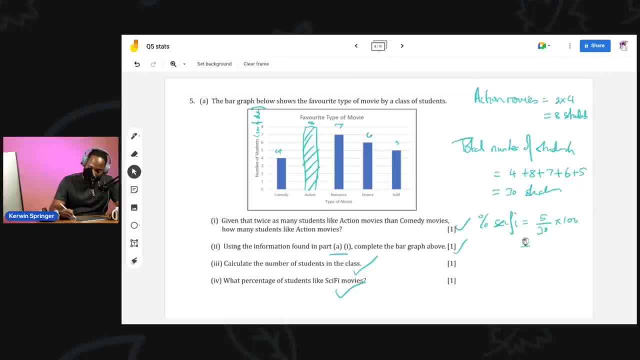 guys more money, but i guess, uh, oh no, Lemme, just kinda take each other's third bet job, multiply by 100 over 1.. If this company is like this, it's like freeness, of freeness- How much times 6 could go into 100?? 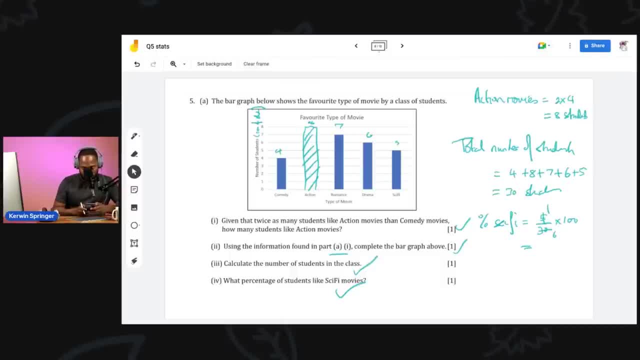 12 point something. 100 divided by 6 is 16.2%. 8 could go into 100, 12 point something. So what percentage of students is that? And we got to go there A class Soon as 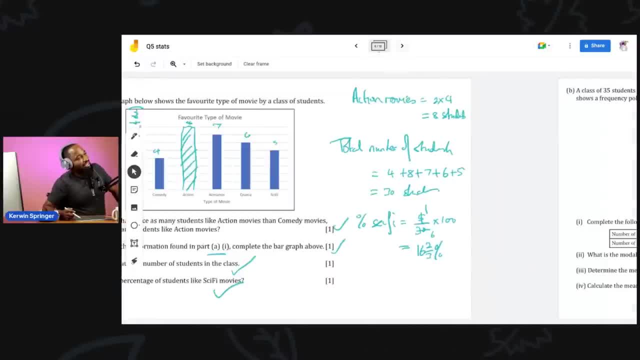 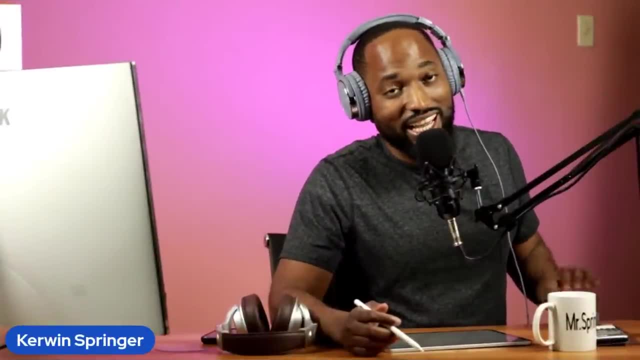 you see question 5 in the in the exam when it's only 17,. that's right around the corner. any next 10 days or whatever Soon, as you see question 5 in your paper, scan it through and see if you see draw. 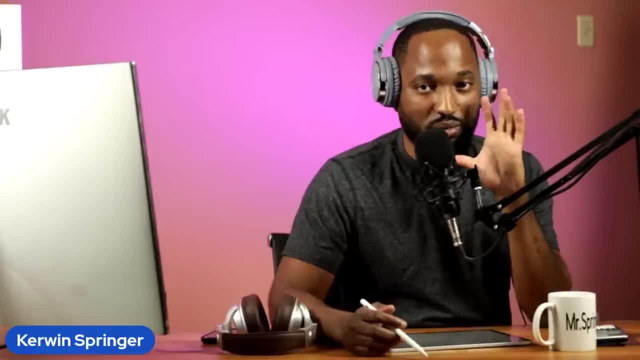 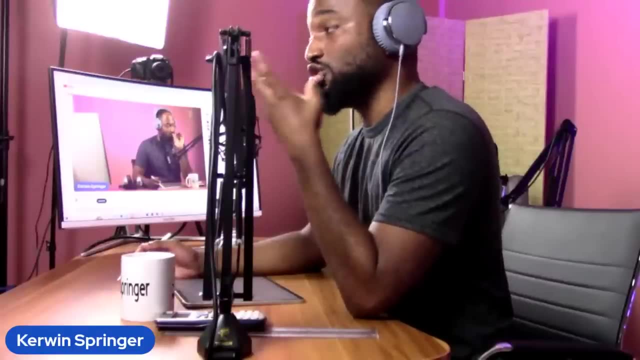 If you see, draw, set aside some time to draw, either community frequency, Instagram, whatever it is. you had to draw, So don't waste no time, Because you see how time consuming sometimes it is to draw. something could take right A class of 35 students. 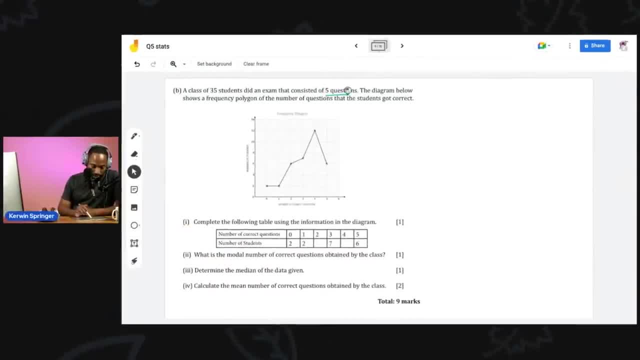 did an exam that consisted of 5 questions. The diagram below shows a frequency polygon, So you notice how they didn't close up the frequency polygon. Sometimes in CXC they insist that you must close the frequency polygon and then, when they give you a question, 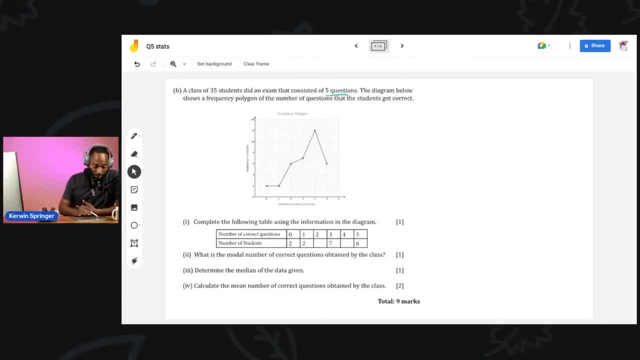 they may close the frequency polygon, So their frequency was that, their frequency something It make a polygon, but they didn't really close up the form into a polygon, right, However, we're not fighting it Completely. following table using the information in the diagram. 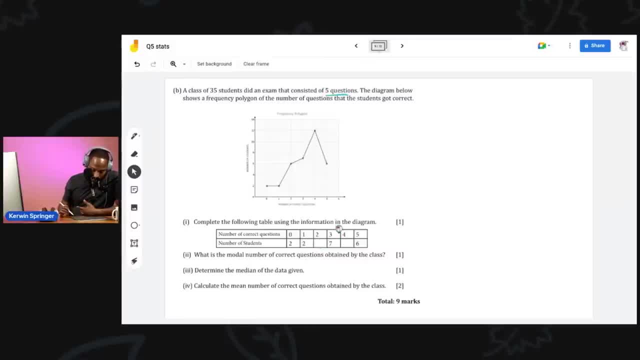 Oh, something's missing here there. Let's go get it. Let's go get it. So two needs to map to six. Number of correct questions. I don't know if all you're seeing it. It's a little kind of zoomed out Let. 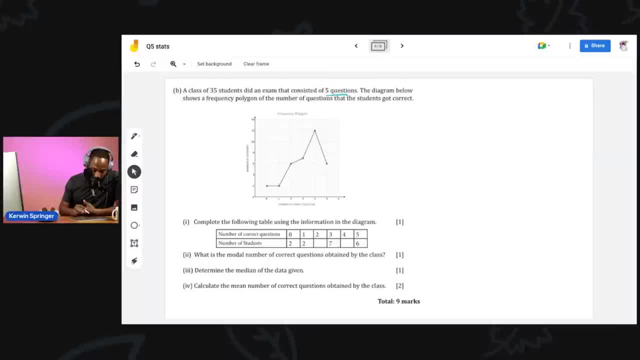 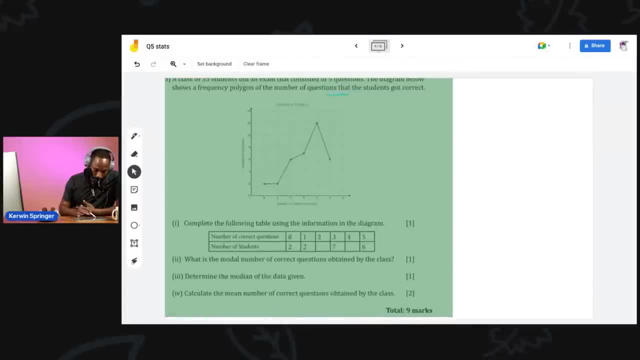 me get a little zoom in there So you're seeing number of correct questions and number of students: Nice. So therefore, the two here maps out for the sixth day, Nice, The four actually maps out for the 12th And the five maps with the six again. Well, they do that. 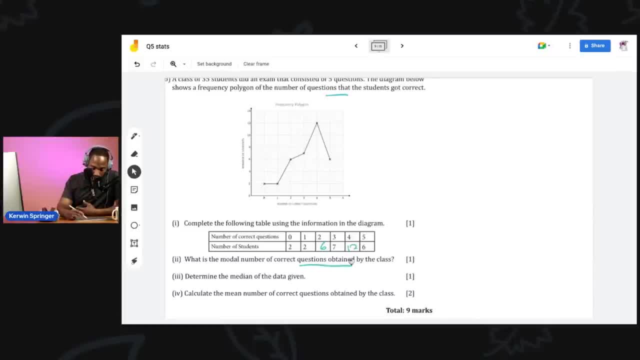 What is the modal number of correct questions obtained by the class? So modal means most frequent. So the modal number of correct questions is what? The modal number of correct questions is not two, although you're seeing this number most repeated because there's number of students. 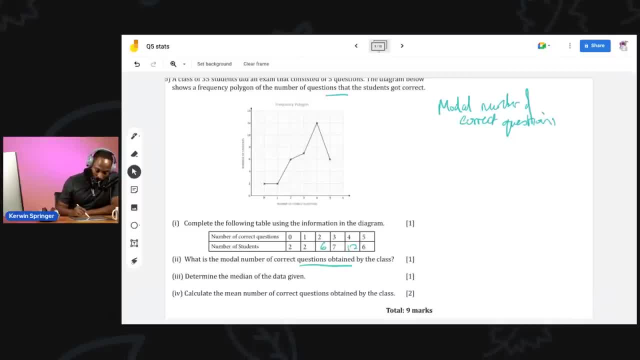 The modal number of correct questions is not 12, although you're seeing that is the highest frequency. The frequency is not the answer unless you specify what: the highest frequency, the modal frequency, The frequency is not the answer. This just indicates which one is the answer. So the modal number of correct questions is four. Right Four is. 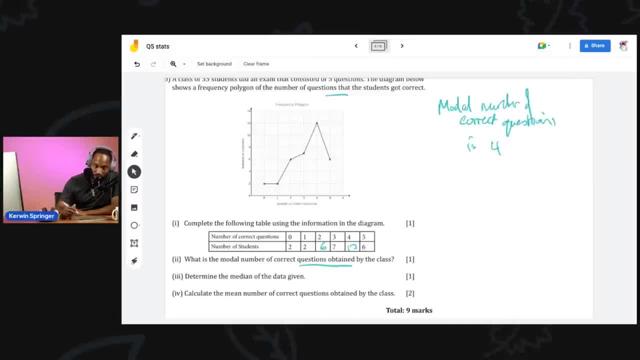 the answer. Number of exclamation mark there four, factorial means something else. So the modal number of correct questions is four. If you're not seeing it, if you're zooming in, really good, there it's four And you could actually zoom in on YouTube videos now. 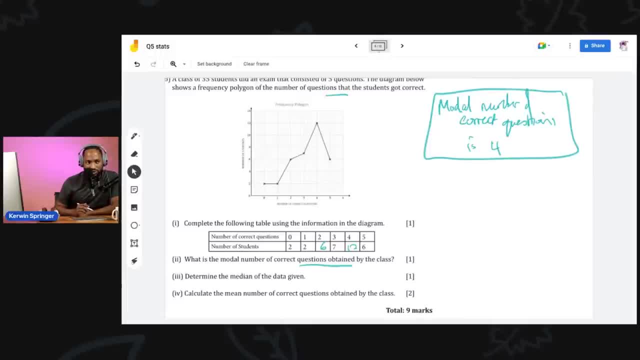 Did you know that? I don't know if you could zoom in on live YouTube videos, though I'll let you check and see if I can zoom in on this video here. Determine the median of the data given You can zoom in. Yeah, The median of the data given. What? The median of the? 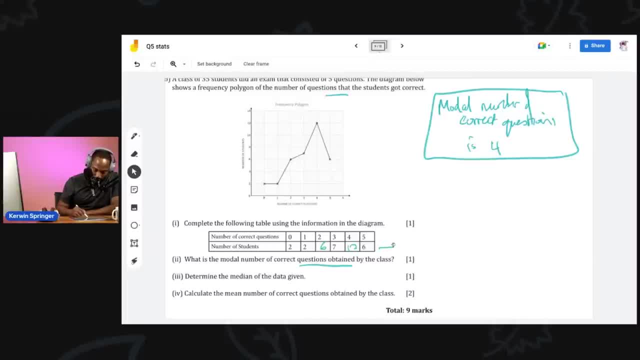 data. Oh well, you need to watch your frequency. There are a few things we could do. How many seconds? How many students again? They're actually there already. How many students All of this eight up here? I don't know if all you can see. Thirty-five students, Yeah, Thirty-five. 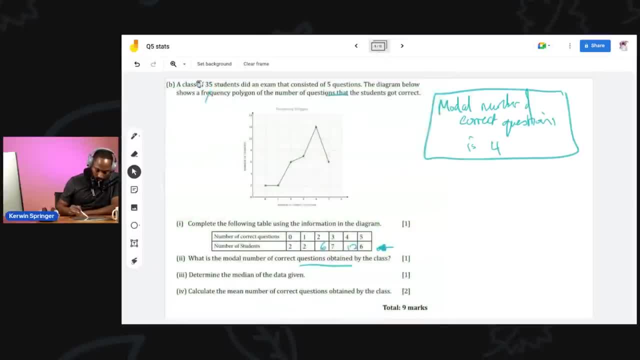 students, Right? So we have thirty-five students. So what should I go in and do If you have thirty-five students? how are you finding median again, Median is Q2.. The second quartile is the birth certificate name for median: Q2.. Quartile two: And you find it by saying: 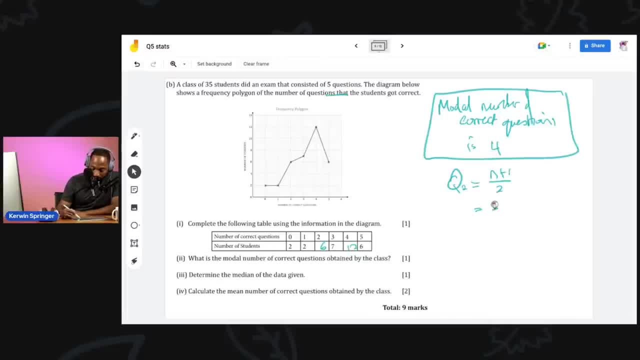 N plus one over two, Half of N plus one And N is thirty-five. N plus one over two, So that's thirty-six over two, So that's 18th student. So it's the 18th student when you line them up in order. So we can go from top or we can go. 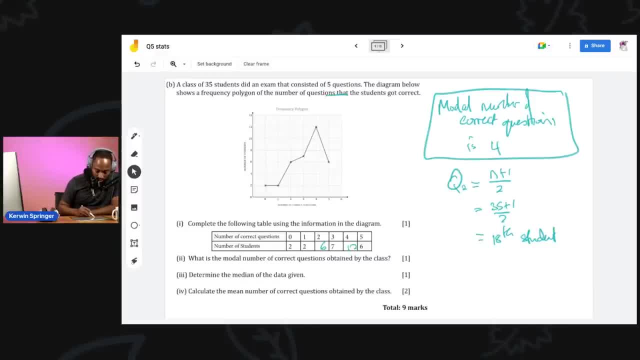 from here And we cross And ultimately we reach 18.. Two and two is four and six is ten and seven is seventeen. The 18th student is found in four, So the median is four And this is the median which I said is one side of the 18th step. So 32 words Now we should. 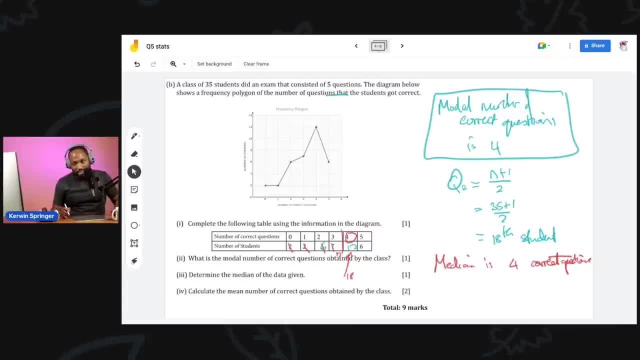 have this one over here, because we have these two, And this is not exactly solid. This is not exactly half half of a golden rule. Instead, this is half a double root. So anything important. So we will be 𝐯-𝐡-𝐤-𝐉-𝐡-𝐟. 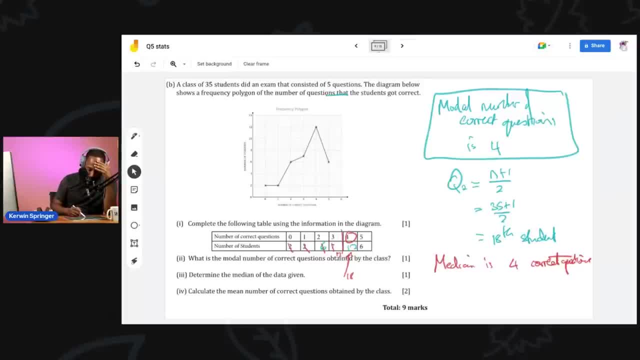 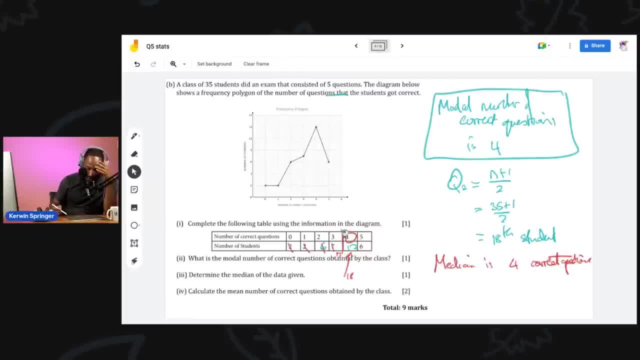 I think it's somewhere here, but it's actually here Because most of these students- right, most of them- get between three or four or five correct. I'm calculating the mean number of correct questions obtained. Ah, see the comment mean now. 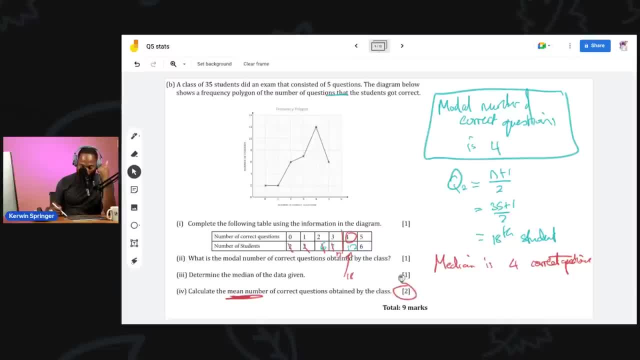 So how do we find mean It's two marks this time? How do we find mean I need to go to a separate page for this boy? Why all these statistics, questions, taking up all this page? Just give me a little page. 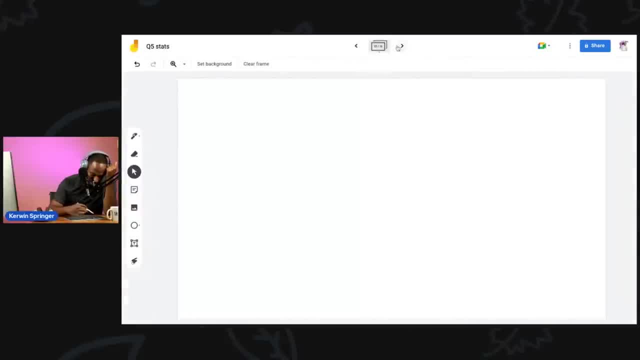 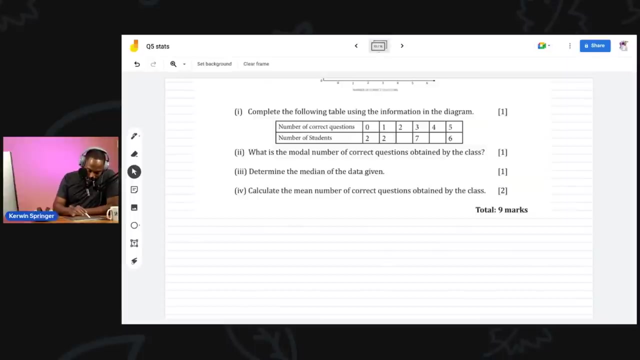 Somebody. maybe page 10, and maybe I can just sneak in this statistics class taking a real long boy. Don't worry, we finish it now. Yes, so this is the formula, This is the special formula. now, Now wait, as we get there, we get some kind of four, six, some kind of six something. 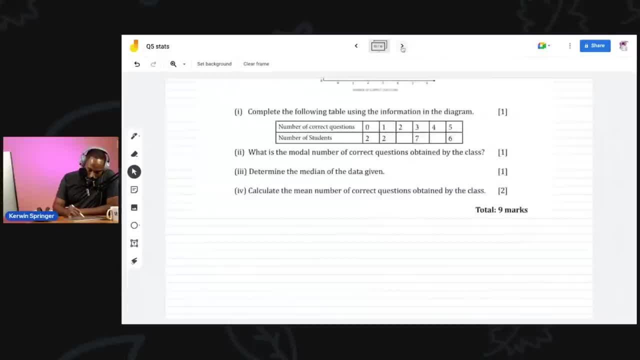 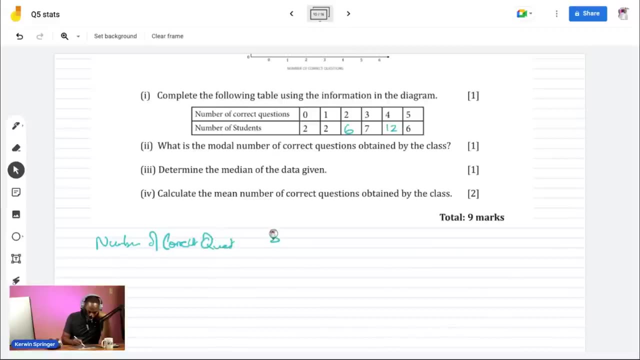 Six twelve- Let me just fill back in this spot here: Six twelve. So it's like if I create a table and I want to write a table like this so you can see number of correct questions, Then I have student number or number of students. 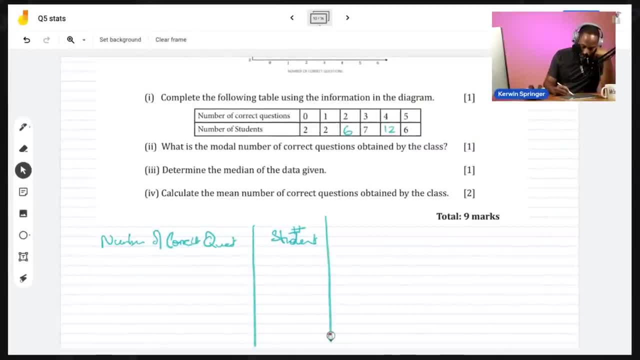 Then I have: okay, let's do this first. So let's say I have zero, Zero, two students got zero, two students got one, six students got two, seven students got three, twelve students got four and six students got five. 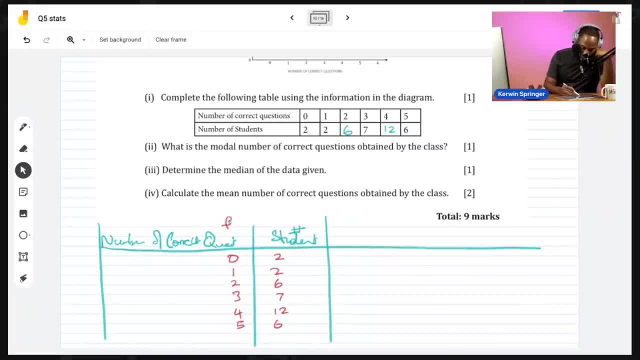 So this is the frequency and this is, like your individual teams, frequency on your individual teams. Is that good? No, This is the frequency and this is the individual, the number of questions, correct? So your frequency is the number of students. 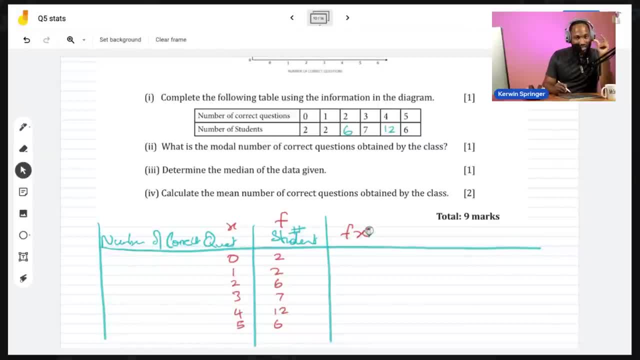 All right, we're ready now. So the next thing I need to do is get f of x, like how much students get each part correct. So zero students. sorry, two students got zero, So I can put two by zero is zero. 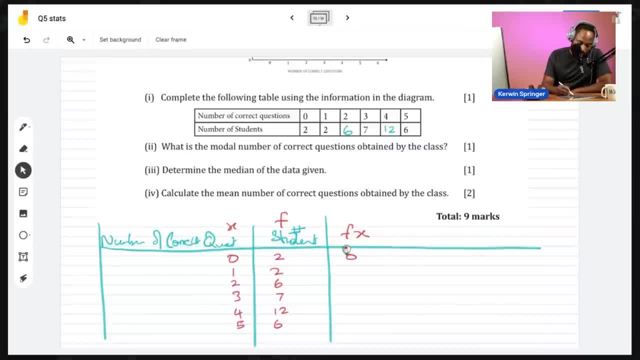 It has a reason for the madness. And two by one is two, Six by two is twelve, seven by three is twenty-one. four twelves are forty-eight, five, sixes are thirty, And then you add it up So it's like you're working out all the students, because, remember, it's like twelve students. 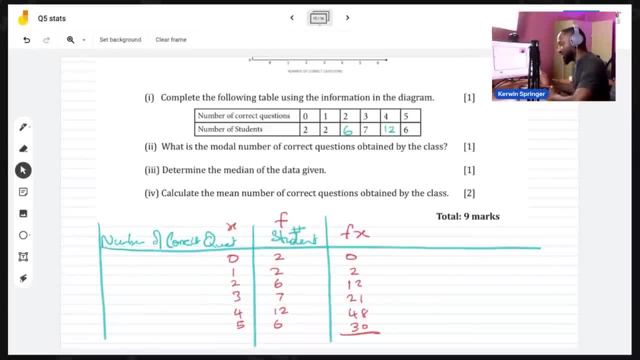 get four. So in all their points will add up to forty-eight, so you get the sum of all the points. So the sum- and that's the symbol there- of f x is equal to somebody tell me how much is the sum of f? x? 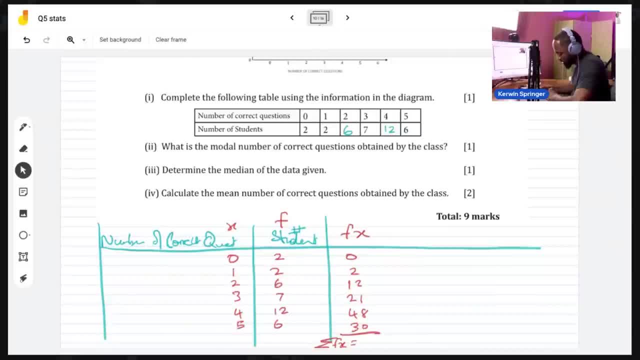 You also need to know the sum of f. So the sum of f is just the sum of the frequency, which we already have been told is thirty-five, So the sum of f is thirty-five. the sum of f- x is one hundred and thirteen. 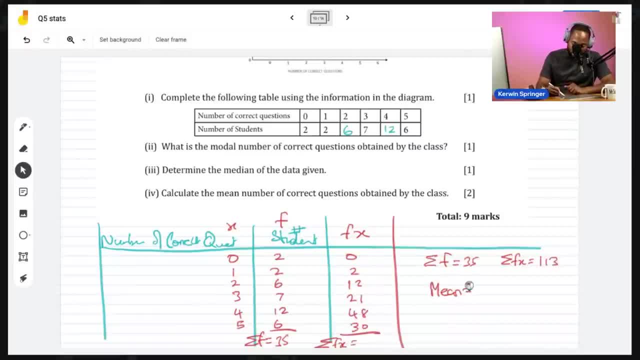 So that's how you find the mean of grouped data like this. So the mean is the sum of f? x, not the sum of f of x. f of x is function f x, just meaning the frequency by the individual scores Divided by the sum of f. 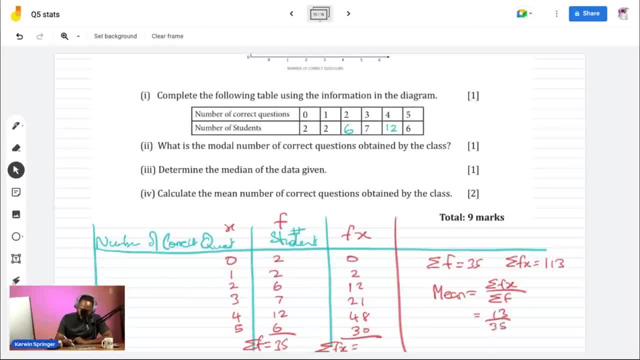 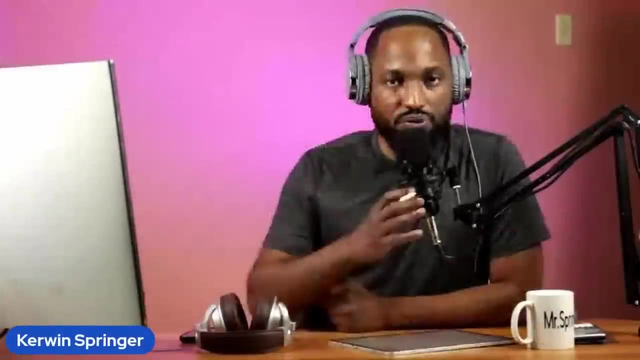 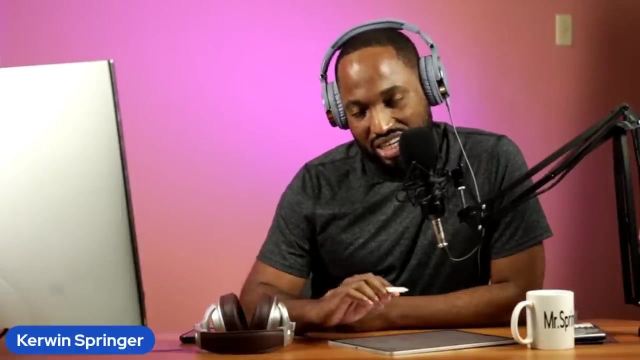 Thirty. Thirteen divided by thirty-five, one hundred and thirteen divided by thirty-five is three point two, nine. Three point two, nine questions, correct? So if I would add in, if this is equal to three, to the nearest question. so yeah, really. 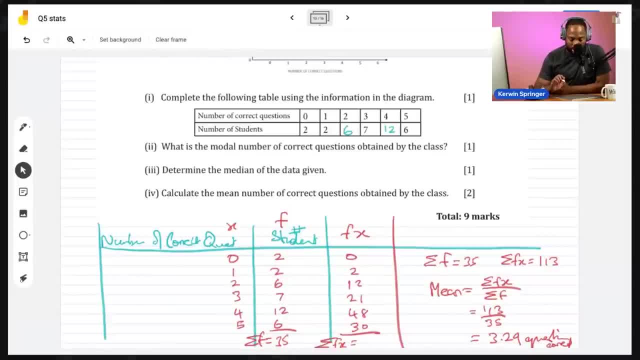 maybe they're not giving that kind of point. two, nine marks here, So I'll put this first, Okay, And then say three to the nearest question right, Number five. Well, all of these are number fives, but let's do one more. 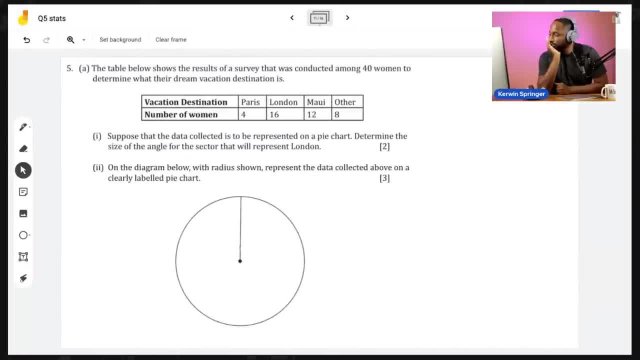 I think we have it in me to do one more. boy, I feel it's just one more. How much you pull it up in this life? Two, seventy-three, Two, seventy-three, One more people. I'll let you do the two more. 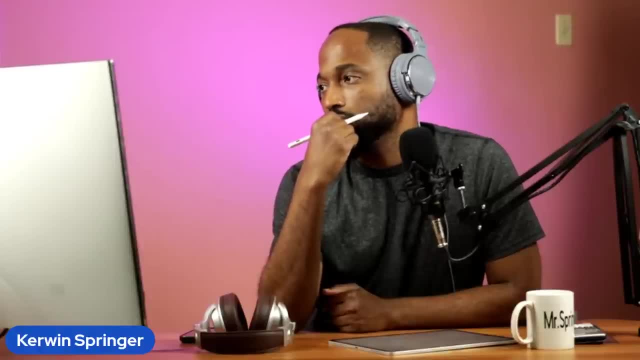 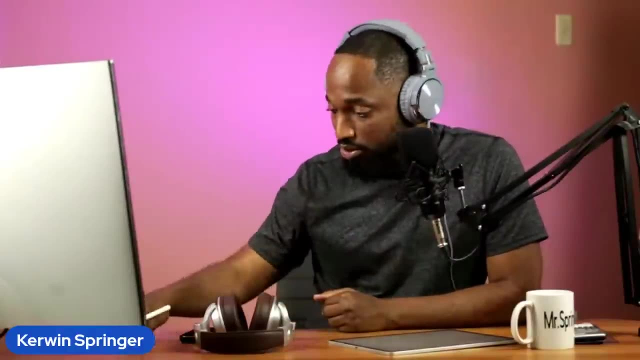 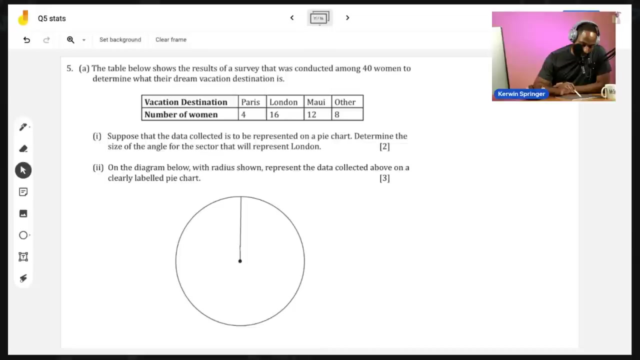 I'll try for the one more first and you'll see the energy for the two more. Oh gosh, I pie chart Remember. Okay, Okay, I'll try. The table below shows the result of a survey that was conducted among 40 women to determine. 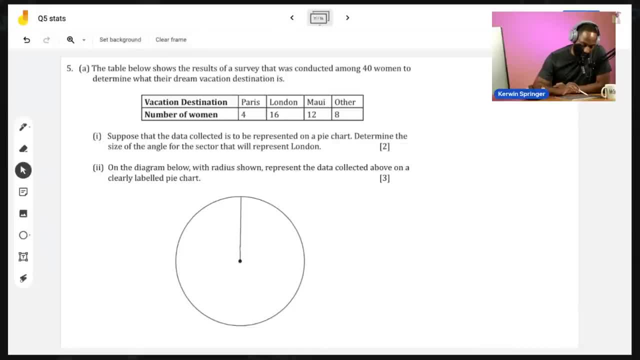 what their dream vacation destination is: Paris, London, Maui, Maui, Maui, Maui. I pronounced it out for a minute: Maui, Maui, Maui. Anybody from high know how to properly pronounce that And other places. This is how I do it. 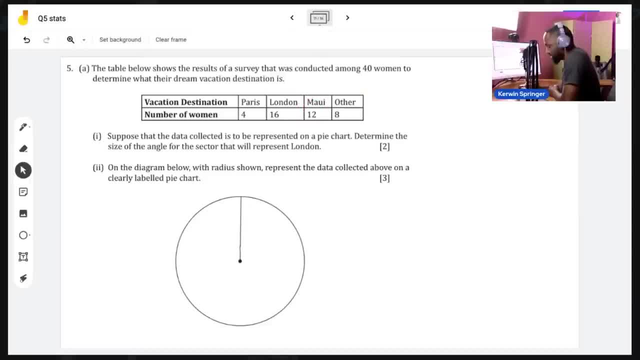 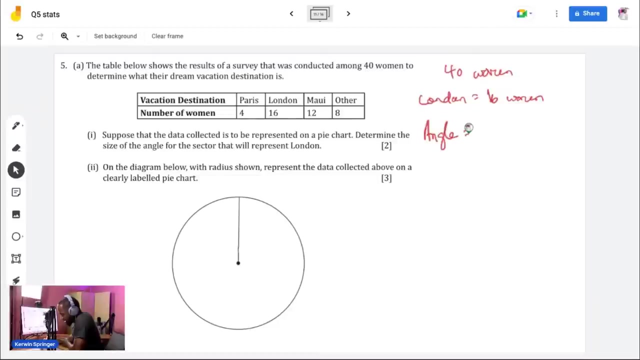 Oh, okay, And then okay, suppose the data collected is to be represented by the pie chart determining the size of the angle. I represent London In London, all right. so 40 women, London is equal to 16 women. So the angle, not a percentage. the angle has to be a fraction: 16 out of 40, multiplied by the full angles in a circle 360.. 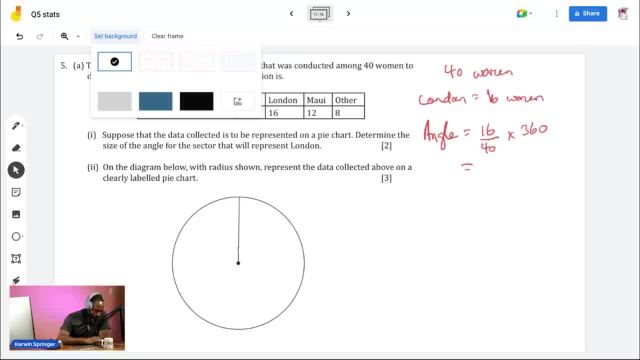 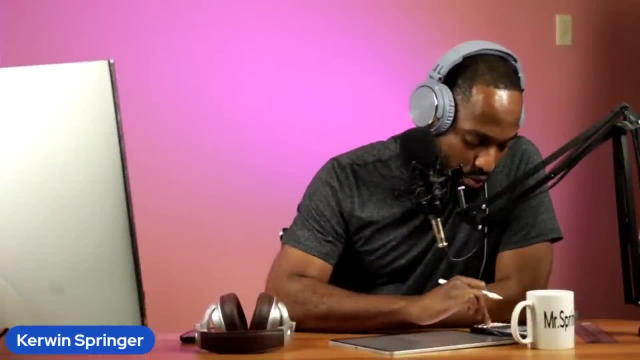 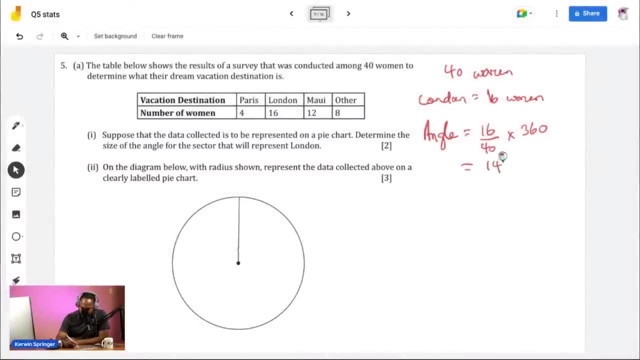 And I'm going to show you how it is. The truth, The trophy, the winning, the first place, the success belongs to the persons who are able to continue where the energy is low. When you are able to sacrifice now for a better future, that's when you're winning. 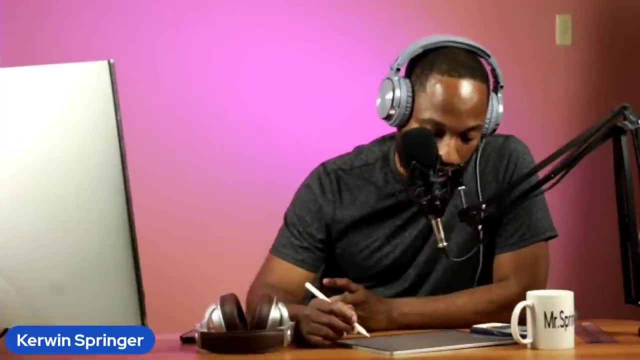 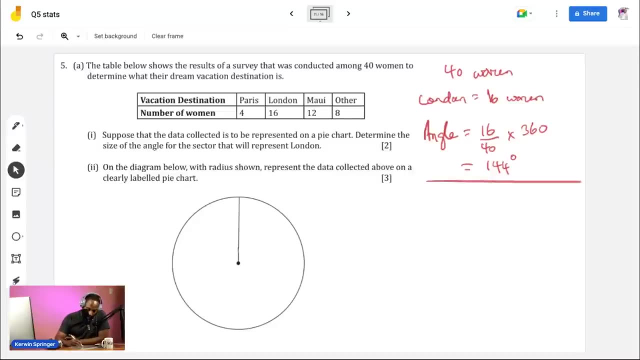 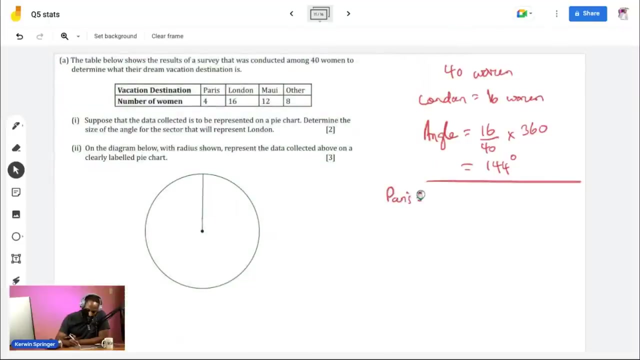 That's when you're winning 144.. And now we need to find the others, because we need to draw, We hold, So that's just London. They find Paris, Paris, Paris is four out of 40, multiplied by 360.. 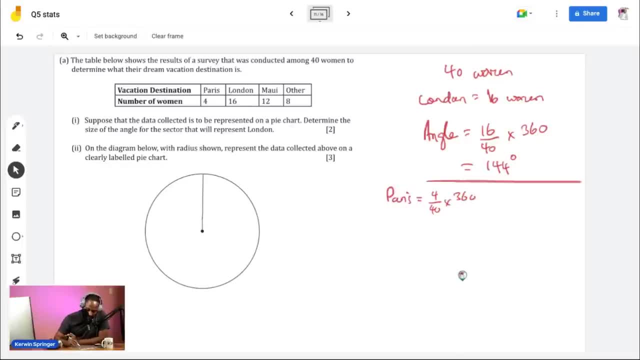 Tell me I 36. now I smell in a 360.. 360 degrees. Wow, He is 12 out of 40.. Multiply by. So I will use it: Multiply by 360.. How much would I get for that one? 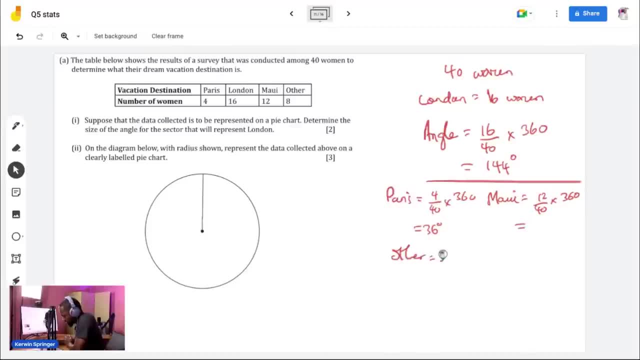 And other, It's out of 40.. Multiply 360 by 72 degrees, Wanna run eight degrees, So we have them all. We collect them all, Like Thanos on the rings. We can draw a graph diagram below with radius shown, representing data collected. but clearly i kind of needed. 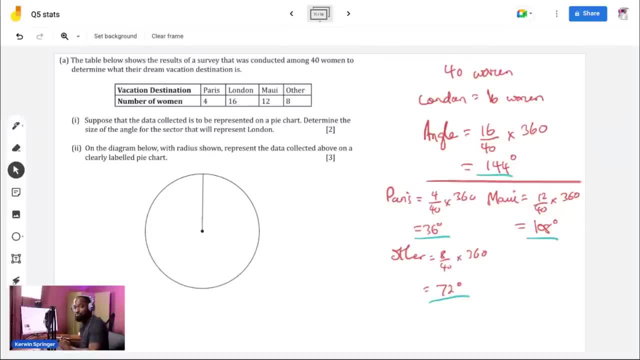 the overhead camera for this one. but oh, what we can do, what we can do, um. so i wanted to show you all how i'm gonna line up the angle on this. so maybe, maybe, just set the set the camera. i'm watching my id to the whole screen and you can lift that. 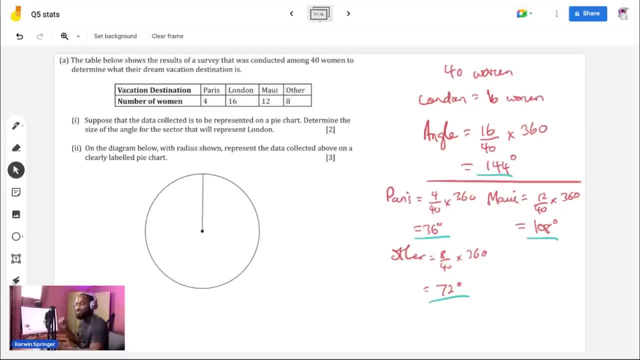 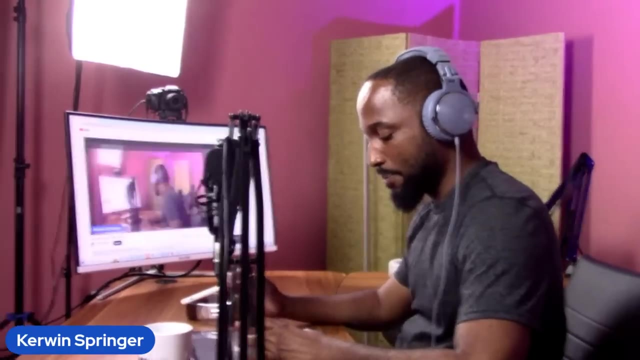 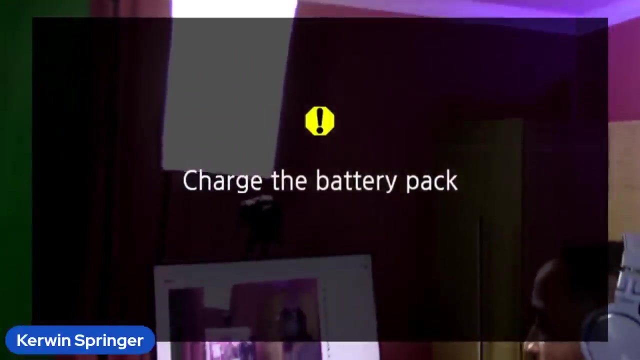 camera and just point it per second, so, but set the whole screen to this. so, yeah, all the way, standby for action, standby for action. so we full screen, right, right. so let's see if i can bring it, have it. have this battery going and dying? oh okay, check the batch, okay. 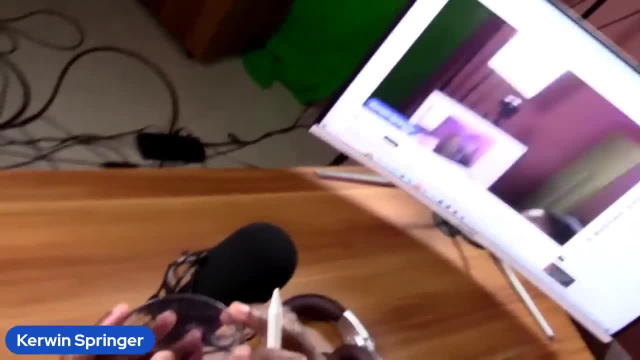 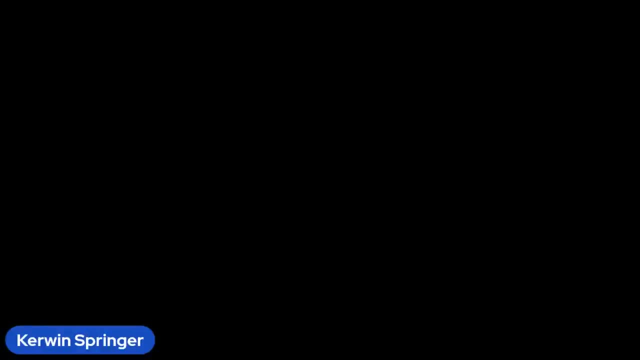 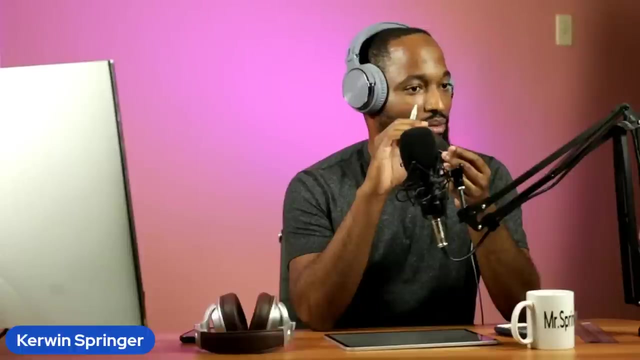 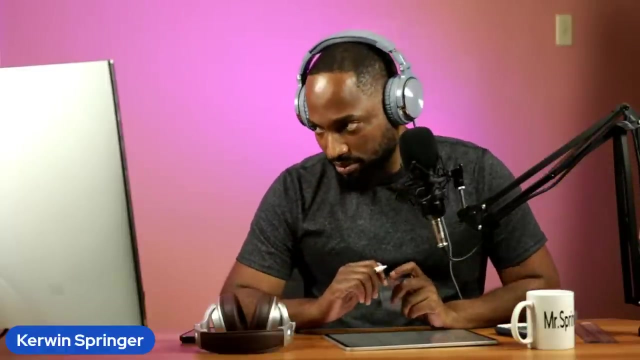 so what i would do? you have more uh task in progress. do not be. i think it cut off. i think it got off. this is working earlier. i'll use the imagination, just plug it back. let's plug back in this one, thank you. so use the imagination, use the imagination. 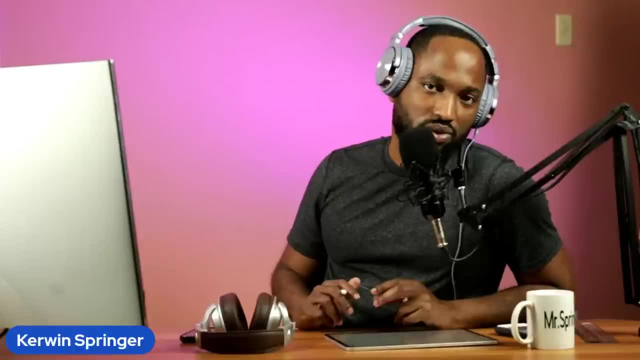 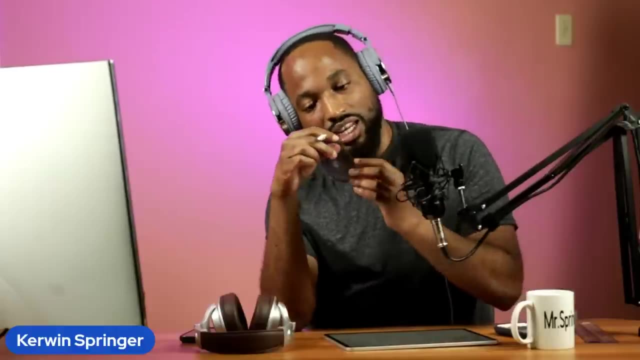 i'll actually show you all how to do this on one of new statistics video so, as i said, you could go out and look it up on youtube. convinced by chat, you want a line of the base light of the projector with the given line, and these days, when they're 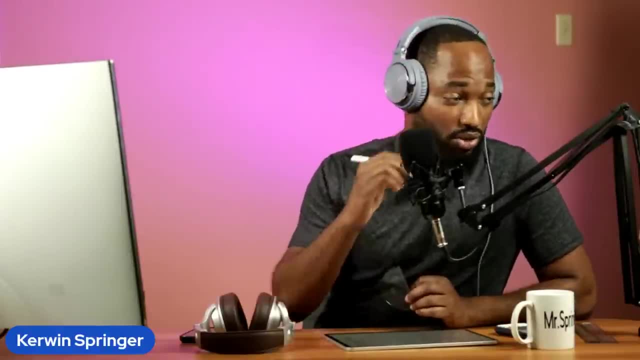 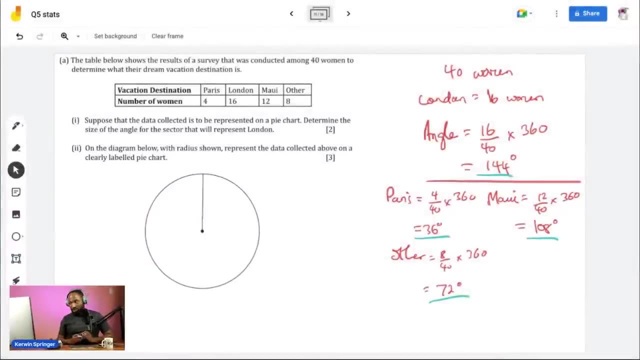 giving you zero pie chart. they start in the hospital line. let's bring back up the screen. they start in your office. that line right there. and number one, vimos касcdamn. normally we had an overhead camera here, but i thought i would not need it, but actually i do. 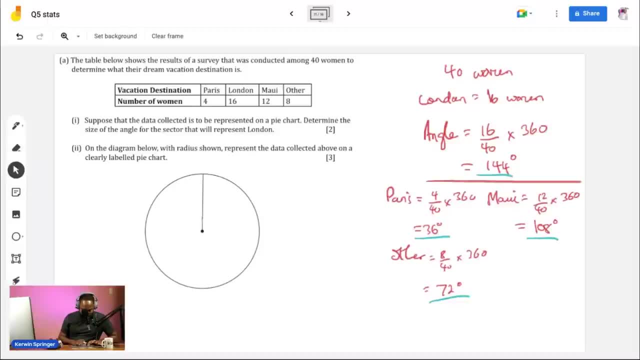 so, um, so you line it up and then the, the center point of the, the projector that goes on the center of the circle, and your, your mark off your angles. so the first angle is 144.. so i can put here about this, so so you know to see. but because how how do you protect us saying don't like this and mom? 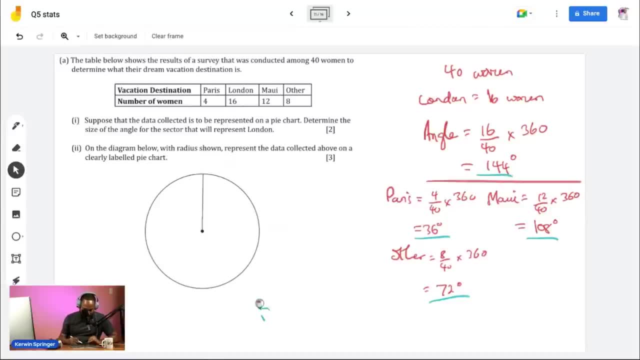 thing because of how big the projector is the angle here? so actually the committer ruler now and join it up. why is any chat if you know how to do this and join it up like that? so and then easy thing. well, some people struggle with it. so then you have 36 to do. 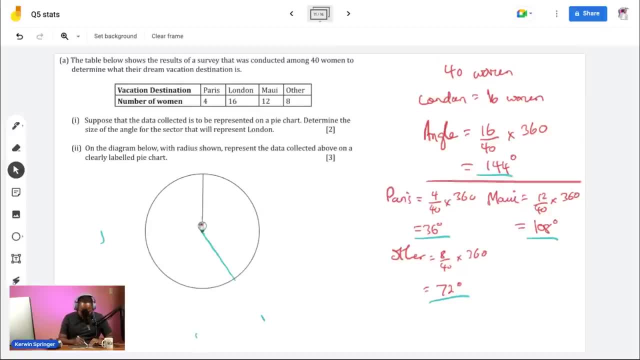 he's like: how are they? so i think i see a little random smudges come across on my screen there because my finger touching it. and then 108, who's the 108's way? 108, 108. he goes about there. so, and then 72 will be the remaining. 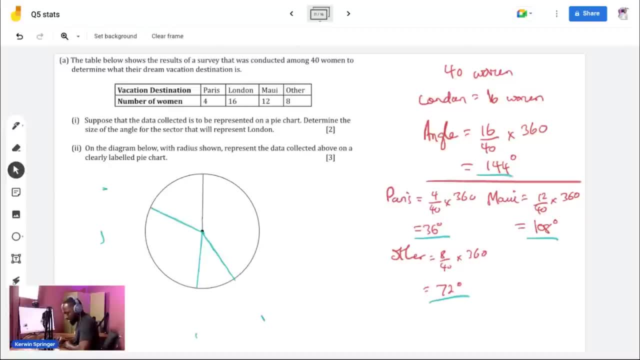 the remainders. so i feel like that was good, i feel like i could figure that out, so, and then we're going to put it in. we'll label up, however, i feel. in the label listing london, it's 144 degrees, this one as well. paris, this was 36 degrees, and this isn't maui: this is 108 degrees. 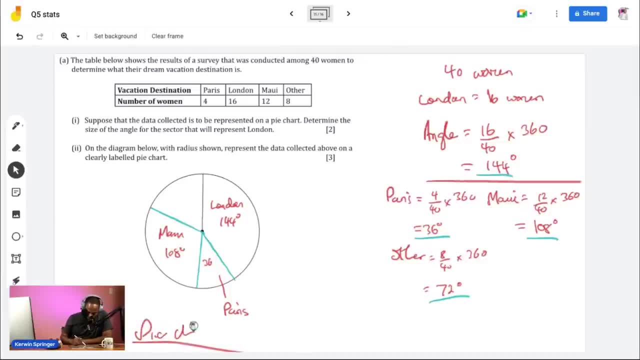 and this is pie chart of favorite or desired destiny nation. we have our hammer label day and this is other. this is 72 degrees and one degree is- you don't need to put this. one degree is 360 divided by 40. yeah, pointer 26. hold on, I have this back the front. one person is that amount of degrees, yeah, one. 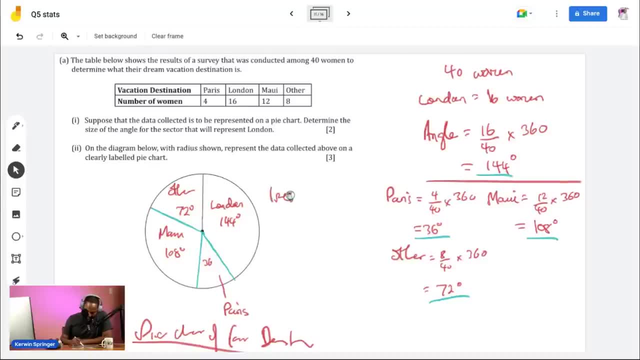 person is. she was a. she wanted- now I talking to myself, I talking to myself- one business: she's 60: 40, which is nine degrees, all right, so you don't really need to put the scale. I just was being a little extra here, remember? I can't draw dots on this, this, this thing, so that's. 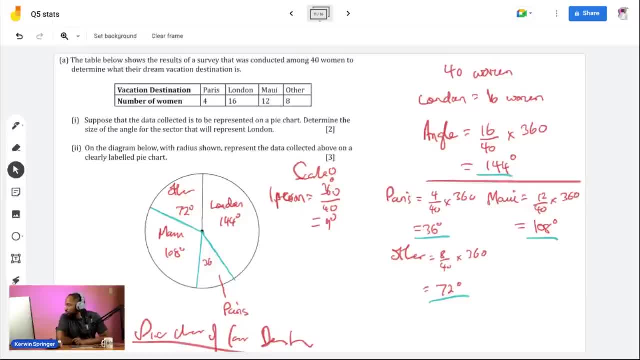 how we collect the marks in the pie chart. yeah, so when I'm doing a new angle, I move to the, I move to the new line. easy. I've seen some people saying easy and some people people saying they're very negative. so we done. the one more part b. let me see if I draw anything. doesn't look so. so therefore, 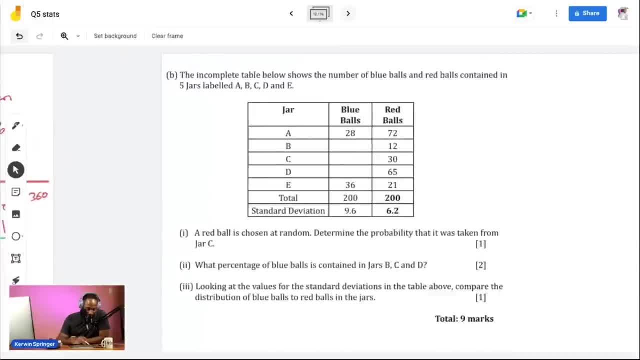 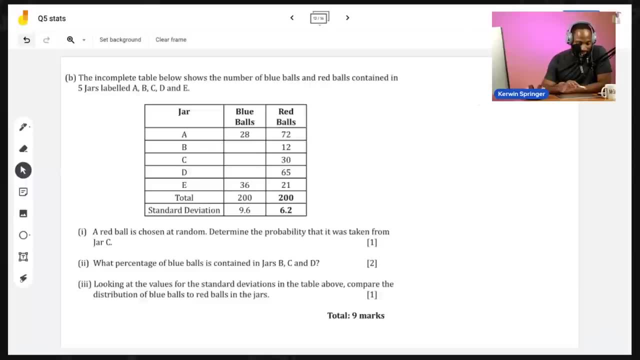 we shall do this, then. the incomplete table below shows the number of blue balls and red balls contained in five jars labeled a, b, c, d and e. the makers of these questions is not what they're doing, so all right, a red ball is chosen at random. determine the. 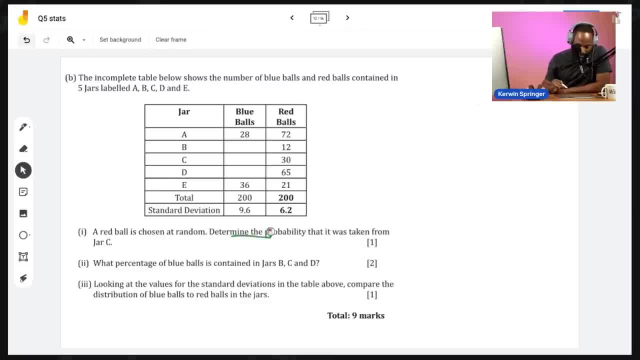 probability that it's taken from jassi a c red chosen at random. hold on, I don't really know what going on in this question. it had 200 of them in total: 200, 200 blue ball, 200 red walls and containing five jars. okay, and we choose a red one by random. we actually 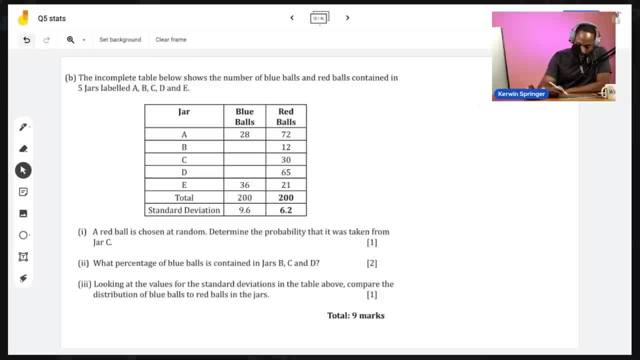 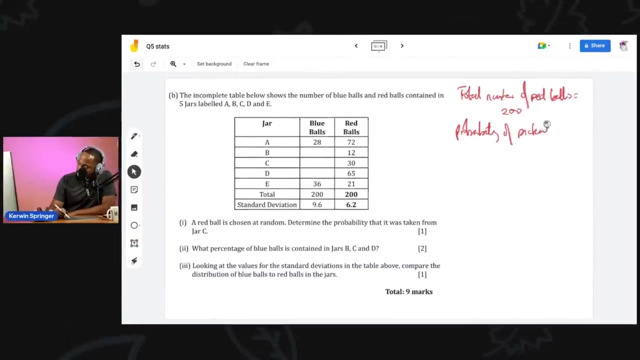 pick a red one, right? so if we choose a red one, total we're taking a red ball and a blue. number of red balls is 200. So the probability of picking from JRC has to be the number of desired outcomes over the total number of outcomes. 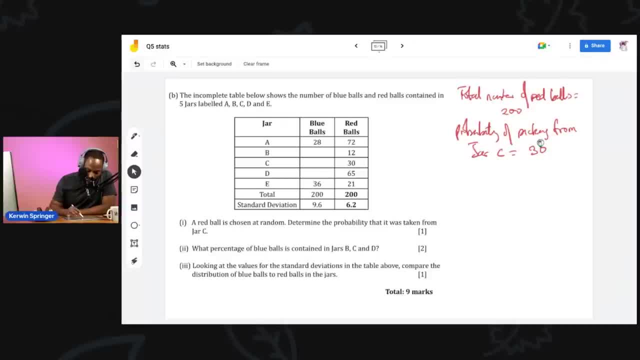 which is 30 divided by, because JRC is just 30, right, JRC 30 out of 200,. so three-twentieths is the correct answer. What percentage of blue balls is contained in JRC B, C and D? 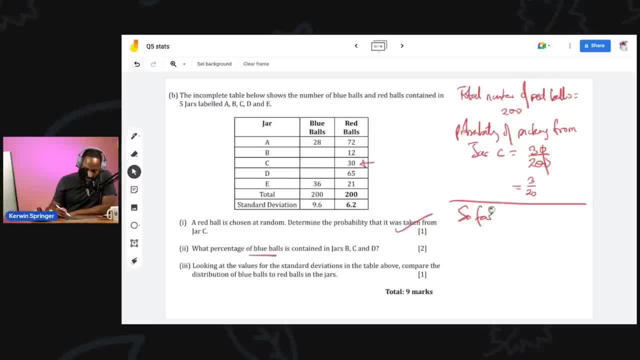 Well, so far- and when I say so far I mean A and E- we have 28 plus 36.. And 28 plus 36 is 64. So far, we have 64 of these fellas, 64 balls. 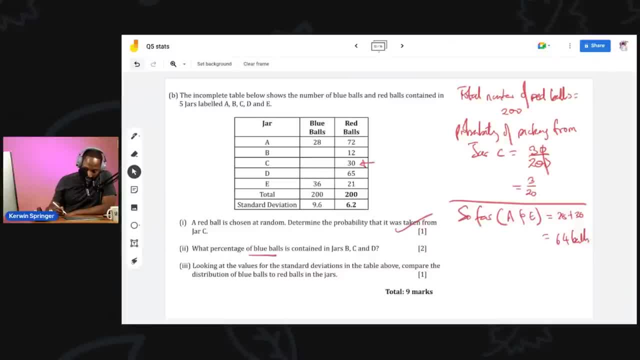 So what percentage is missed out? So missing is 200 minus 64, which is 136.. So percentage is has to be percentage. missing would be one, or in those jars, 136 divided by 200, multiplied by 100, cross, cross, cross cross. 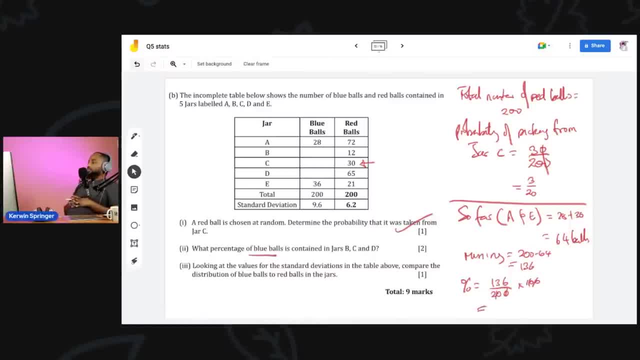 How much y'all get for that. Oh yes, 68% is only real nice. to me, 68% is good things. Looking at the values for the standard deviations in the table, compare the distribution of blue balls to the red balls. 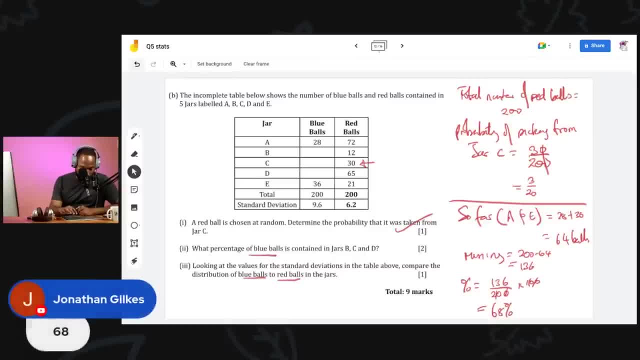 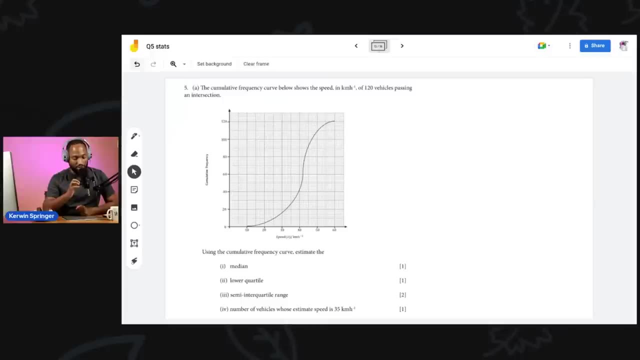 So listen to my talk through this one. There's one more question. No, there's two more questions. I will ask you all, when you finish this question, if all you want to do anymore, if you had enough and you want to just go and study for yourself. 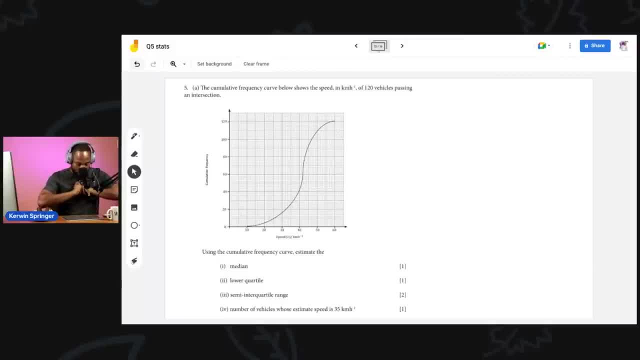 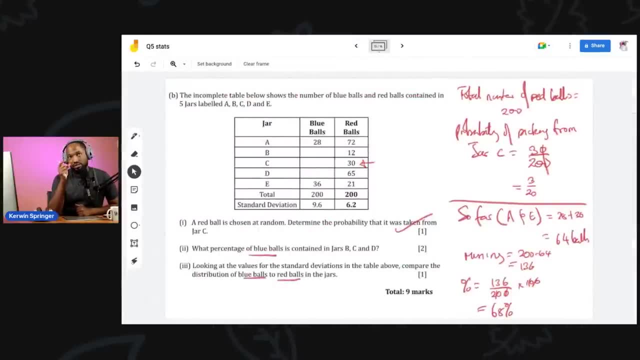 But let me know. So, looking at the values for the standard deviation in the table above, compare the distribution of. So this is the kind of way, This is the way they're asking. standard deviation over the last six years: four years, four, six years. 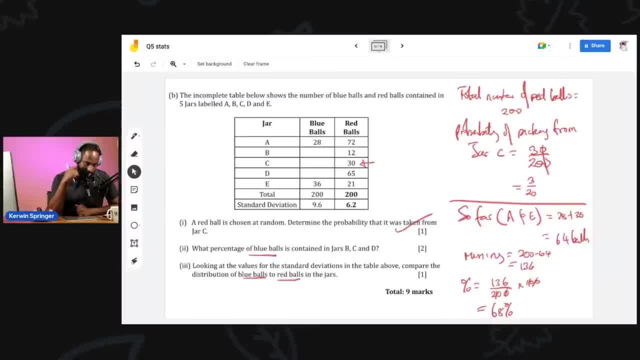 This is how they're asking standard deviation of five years in new examples in 2018.. So how are they asking it? to describe it? So you see, this one has the highest standard deviation. Here's the words, the keywords you want to use. 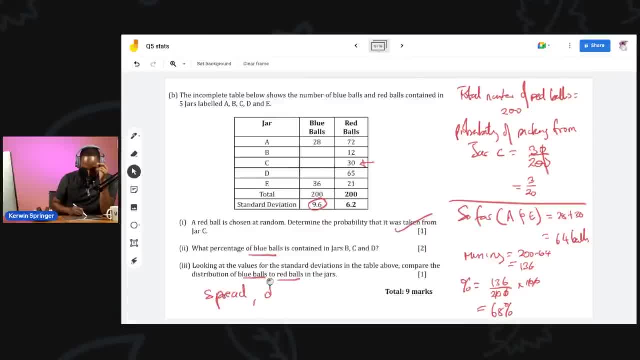 You want to use the word spread and you want to use the word deviate- Spread or deviate- and you want to talk about further from the mean. Once you start to talk about them things you start to hey, I feel like I'm 10,, 9, for real this time. 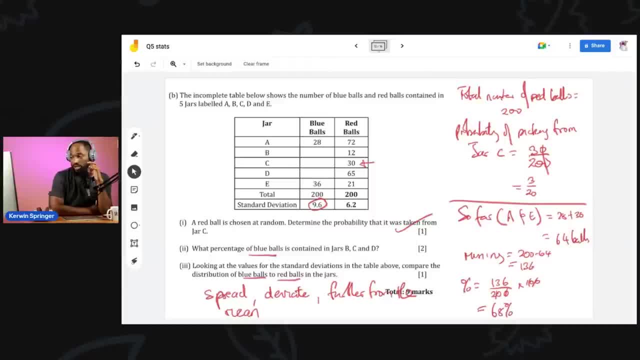 Once you start to talk about them things, you're good to go. So here's what I mean: Let's just do a quick idea of standard deviation so you can collect this one mark when it comes in the exam, right, It will only take three minutes, so let's do it now. 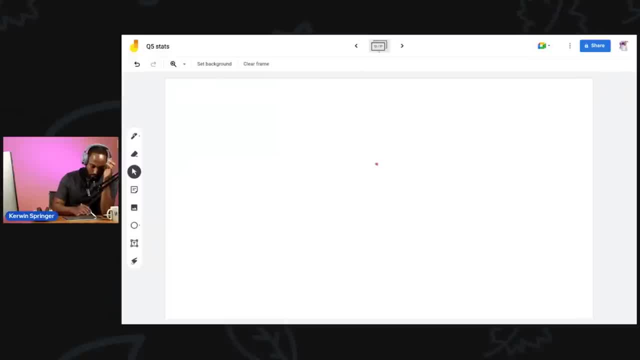 If you go in a town close up, If you go in a town there, you go and you walk in a town right And then you watch all the buildings in the town looking like this, This height. so all the buildings in the town, like the streets there. 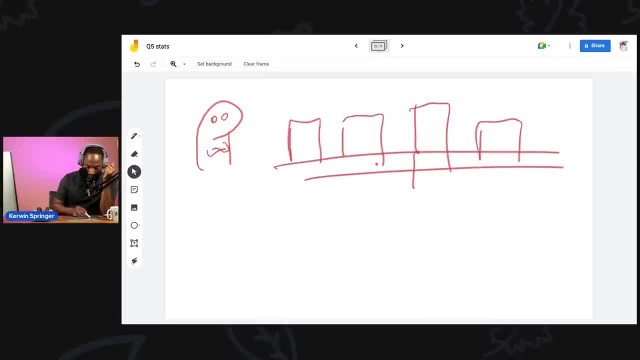 All the buildings in the town looking like that height. What's the average height? The average height is this blue line here, The average height of the buildings in the town, And you can see most of them really close to the average. These are the two furthest away. 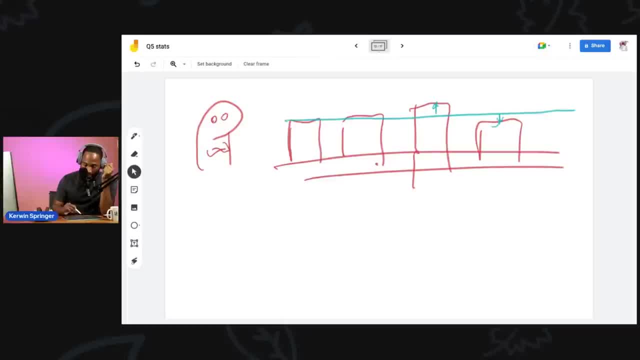 And now? now, If you decide, if you decided, to walk into another town, I'm going to draw you here. So there, you here, And you walk into this town And you see buildings looking like this: What's the average height of the buildings? 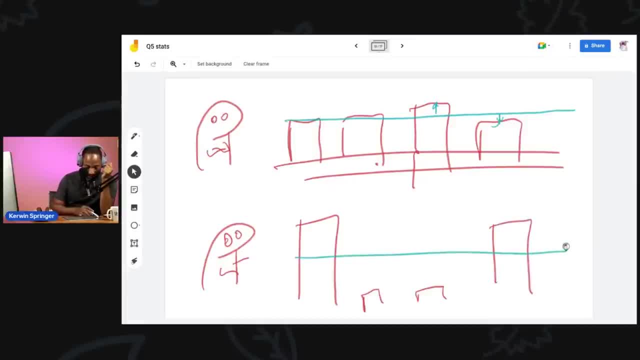 Now, the average height of the building might be the same as that town, But the idea is that they deviate way more, So the standard deviation of these buildings will be higher. So, like I said, the standard deviation of these buildings is like seven stories. 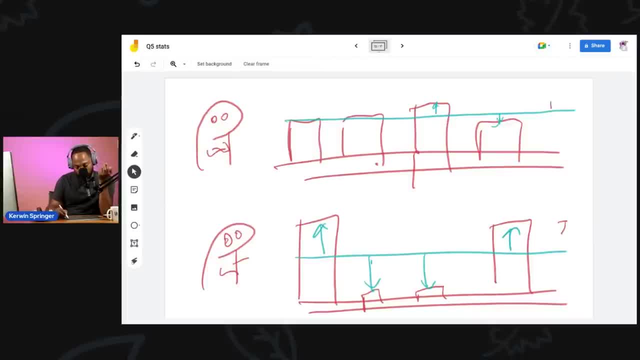 And this one is only like one story or half a story. It means if you're watching average height And if you know the average height, the building is not far away from the average height. And these ones, the buildings, spread or deviate. 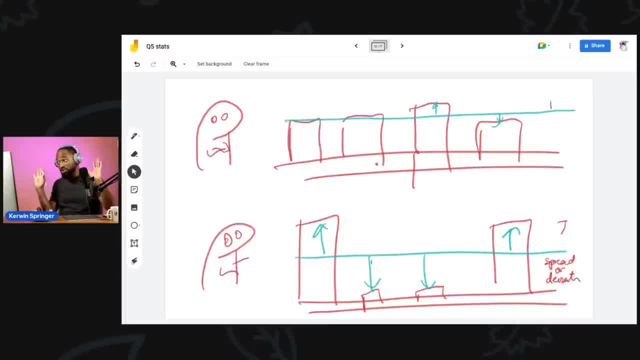 Why is it in each other? If you understand what I'm saying Further from the mean, That's all you need to know about standard deviation And you need to use them keywords, them trigger words to make the exact Examiner happy, and spread and tempting. 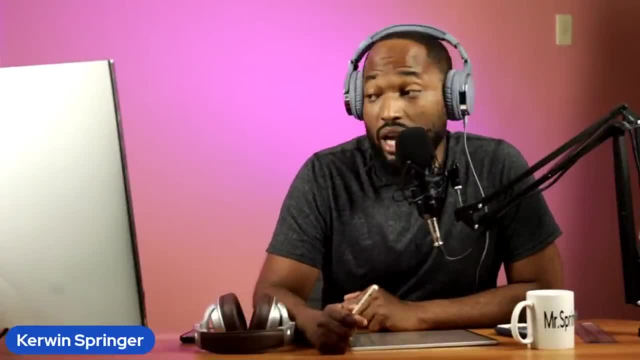 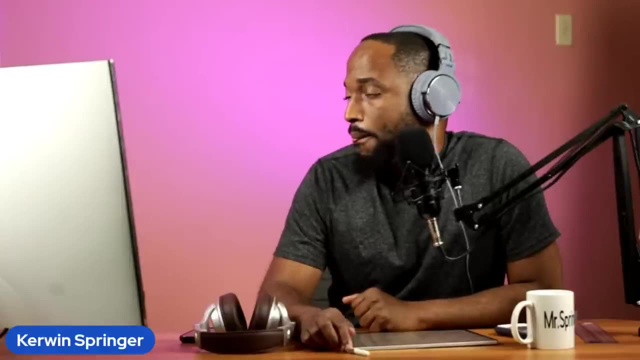 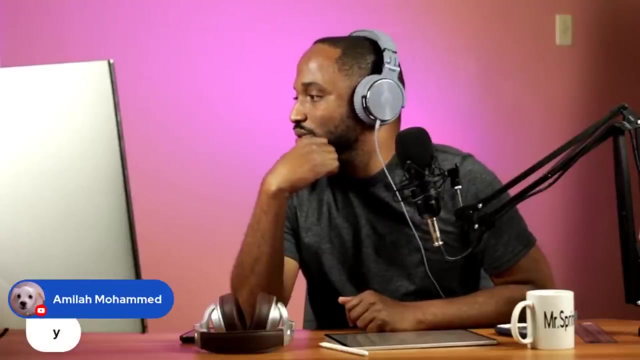 So much people. we have right now 290, 290 of y'all here, 297.. I only want to go for the next question. I'm waiting for the comments to come up here. First time, catching one of you lies on it. 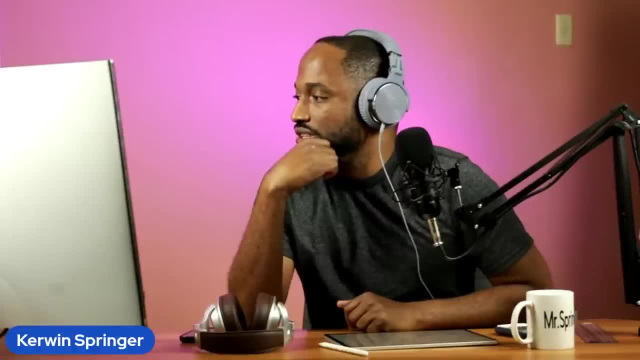 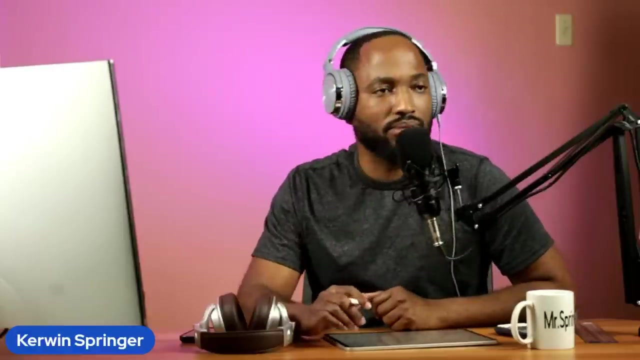 Actually live love from Jamaica. Shout out your country, Jamaica, in the house So everybody's saying yes. Next question: Yeah, let me go. Yeah, yes, yes, All right. So there you go. Thanks question: Was the time I have a whole class to teach? 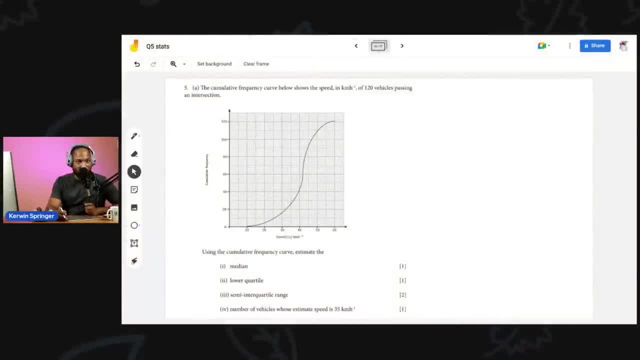 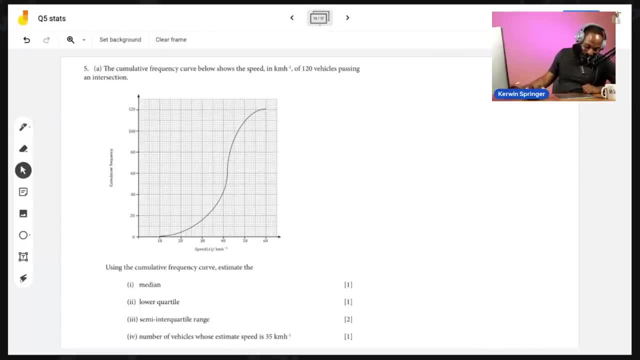 All right. So next question is another community frequency curve. Can you feel that? That's the immense joy I get every time I see one of these questions? So use the community frequency curve: estimated median: the median, the median You have to estimate. 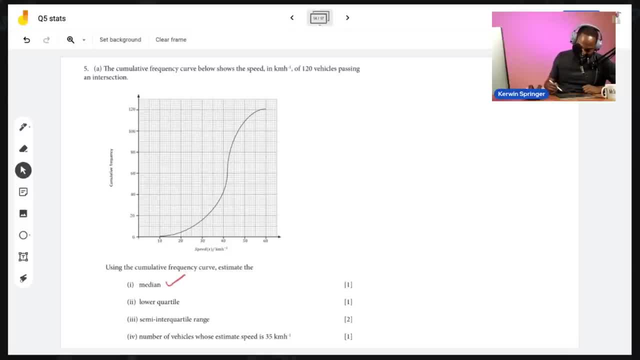 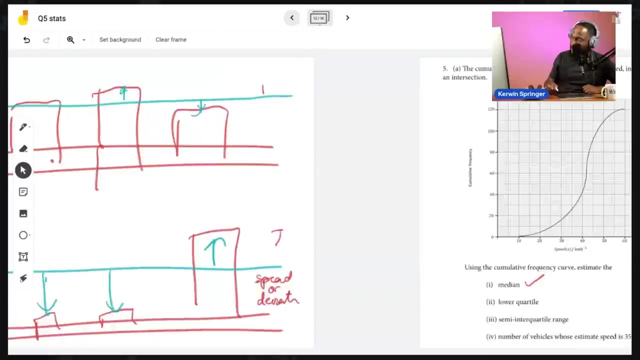 So I need to skip the local. Let me just see if I can sneak it into the next page again. Never I That fella from from yesterday. I seen him, Let's see him again. Go back to slide. one Ghosty pun. 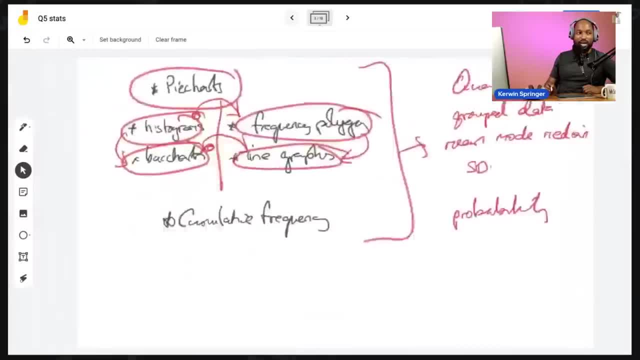 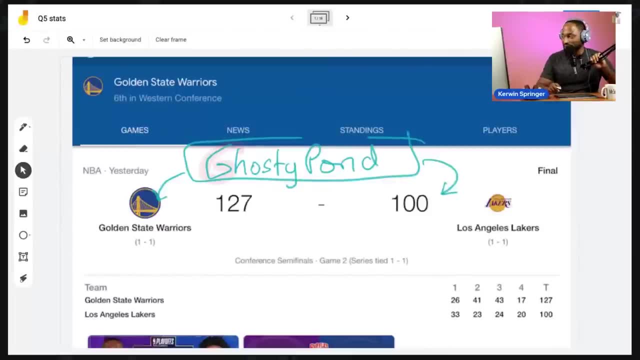 Ghosty pun here Who was getting my talks about? Um, It's ghosty pun in class. Ghosty pun, if you in class one sit down in the back, go to the principal office. Ghosty pun was saying Lakers going to beat Golden State. 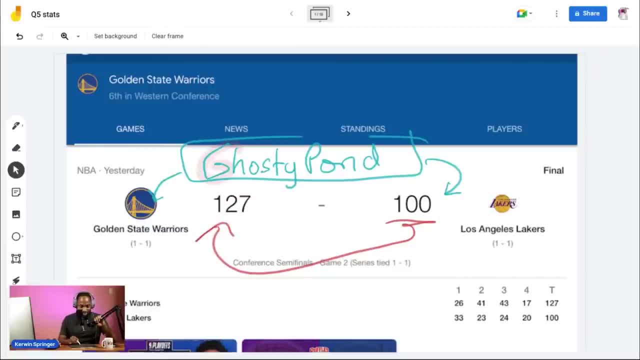 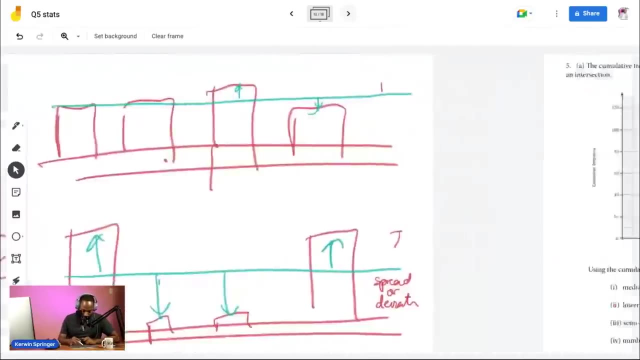 Um, did you watch the match, Ghosty pun? I hope you felt the immense pain of a 30 point defeat. Dylan Brooks kind of talking, All right, So let me go to the new question, Number of page 14.. So you need to determine the median. the median, page 50.. 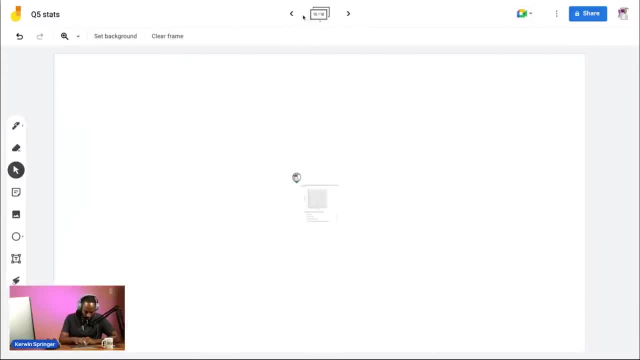 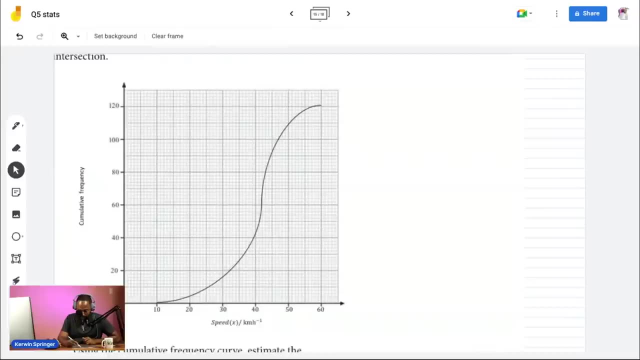 How do we get the median again? Page 15.. I'm not trying to make this big. We supposed to look at Q2 because the median code name in the streets is Q2.. I saw this call him and he heard Q2. and we supposed to say um, Q2 is equal to N plus one over two or half of N plus one. 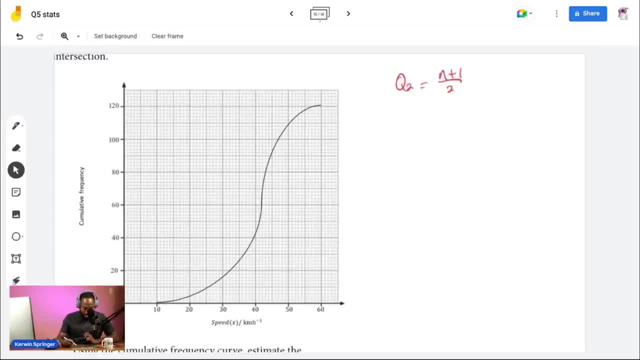 That's where Q2 is located, right, And we see, and now we have, We have 120 of these people involved, How much 120 vehicles involved. volume, So therefore, is 120 plus one over two for intense and purpose, This is basically 60, 60.5.. 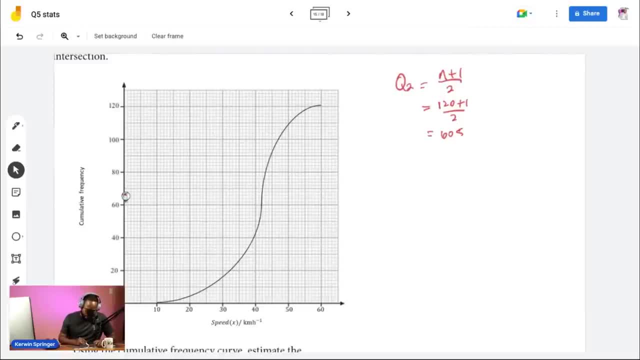 So we go down, look at 60,, bring him across. They had to see them dotted lines right. Just a little smooth job of 60,, 60.5.. And yes, we are touched there. And then you touch the road. 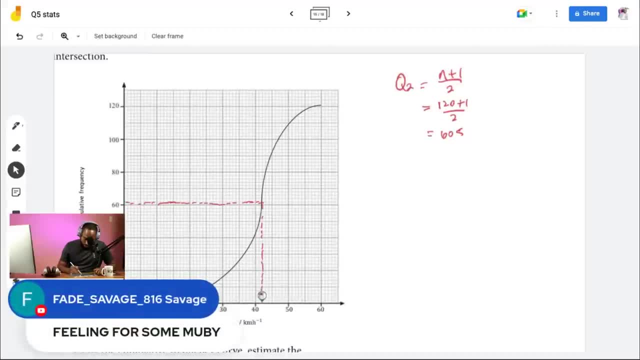 I, I, I tell my students always remember to touch the Road in these questions. You touch your road and then you come back down. So it's only 60.5 to more 60 points if value of 60.5.. 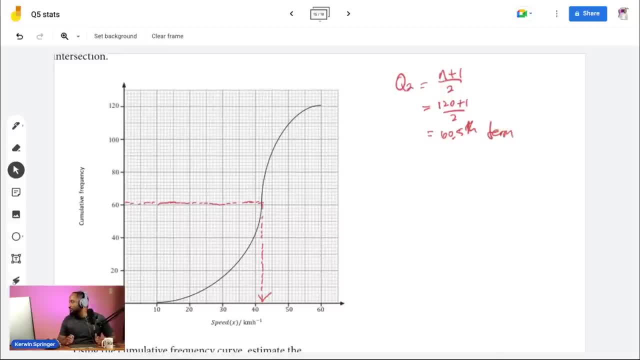 Please turn away by your way. I want to see. all the same, I'll see him. go, step on, Go, step on him. I want that talk yesterday. Go see if I know your quiet So I show you inside. Yeah, No. 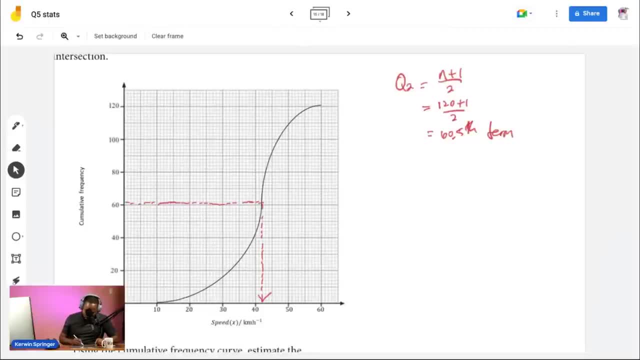 And then the speed is true. Do, do, do, do, do. How much are they getting there? 42. I get 42. So mean, under another screen, Yeah, Remember, you can pinch your zoom. 42 kilometers per hour is the median as a median. 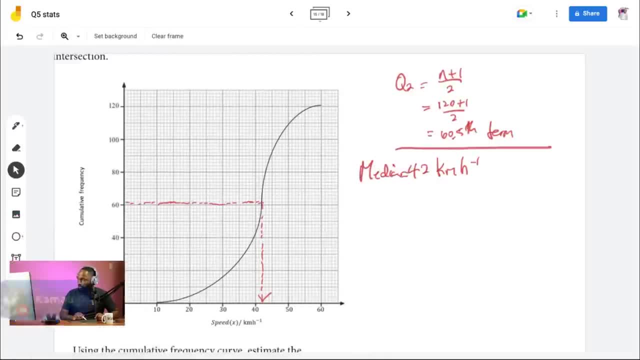 Don't forget the units when you're writing these Q2 things and them kind of thing. Yeah, Yeah, Come come out, come out, come out. It really looking like a 42, the lower quarter. that is code for Q1.. 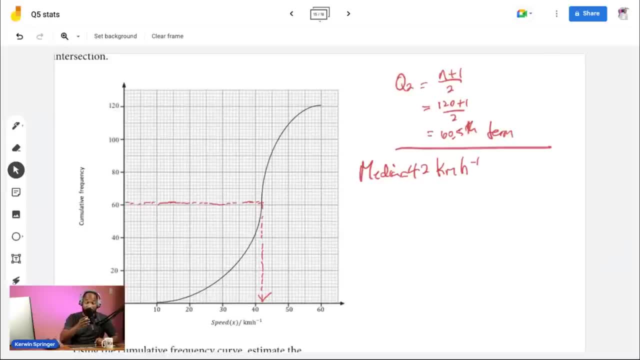 So this was Q2, Q1, and I just explained how we'd get these quarters things. I can look it up after this and most statistics, by the way, semi interquartile ranges: Q3 minus Q1.. Yeah, 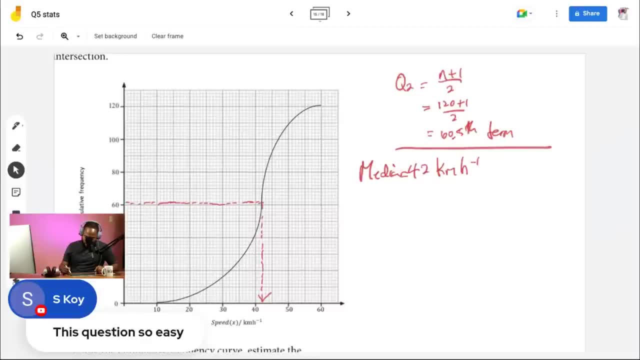 So let me go ahead and find Q1.. Now, Q1 is the same thing. You see, the hundred and 20, it's not, it's cracking my back- divided by um four this time, and you'll get 30.25, or something like that. 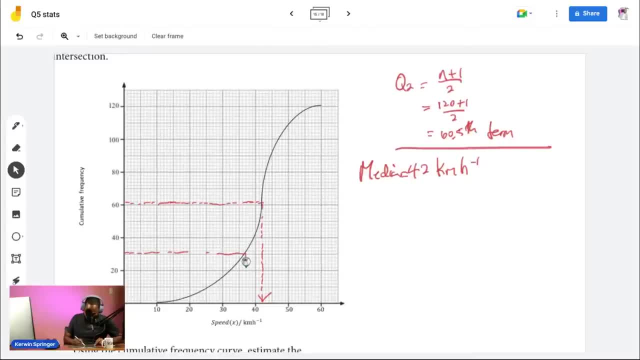 Then you swing across the touch. You would come down This actually looking like a 36, 1.5.. So Q1 to not to be 36.5 kilometers per hour. Same idea. I just kind of skip out some of the points. 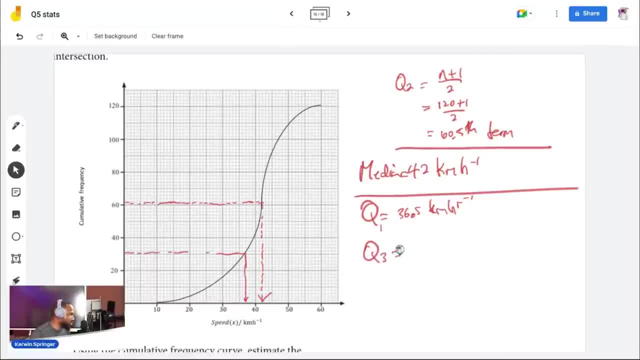 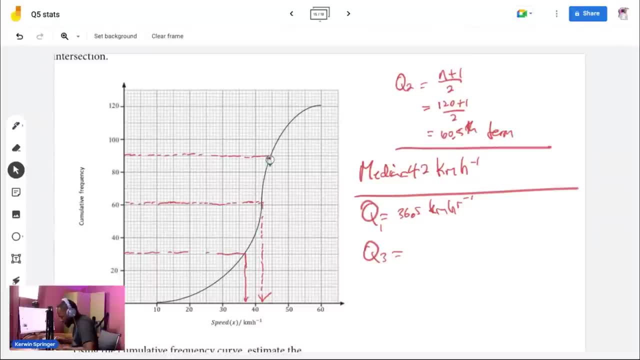 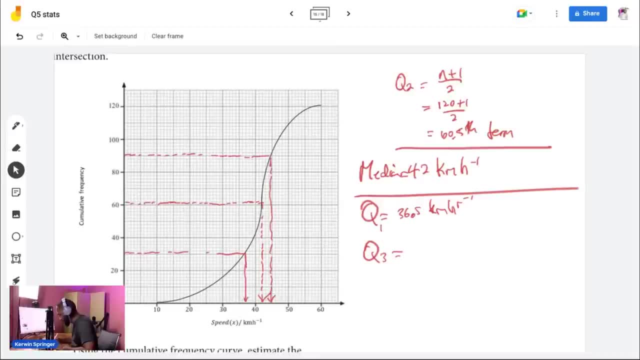 Just not interested in that. That's not what's coming to me. 44.5.. 44.5 kilometers per hour. Niceness, 300 people, We make our next 300.. So 44.5 kilometers. And now, if you want the interquartile range, 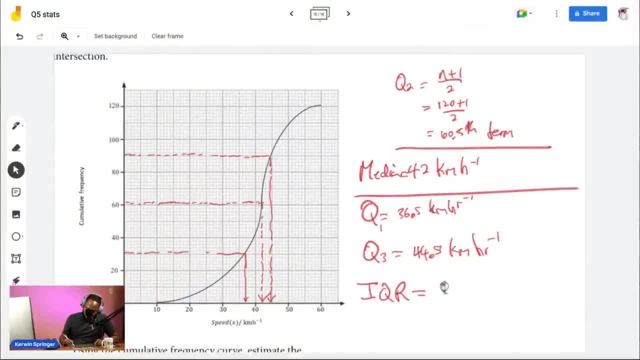 which is fondly known as IQR. you just say Q3 minus Q1.. So that's 44.5 minus 36.5.. Marissa, tell me what I see. Okay, some of the speedy people in this chat. 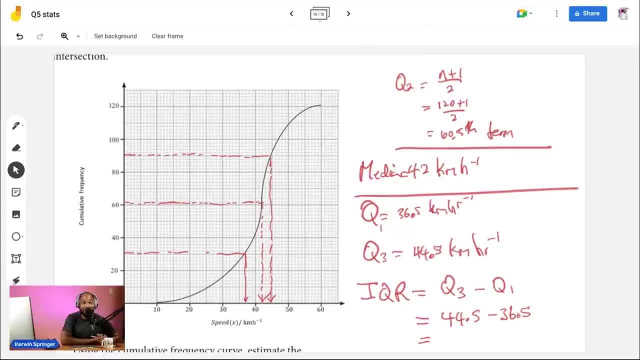 So will CXE release broad topics? If I had a million dollars every time somebody asked me that Cool Creaming. But no, No broad topics will be released. So check Q1.. Q1.. Did I make a mistake with Q1?? 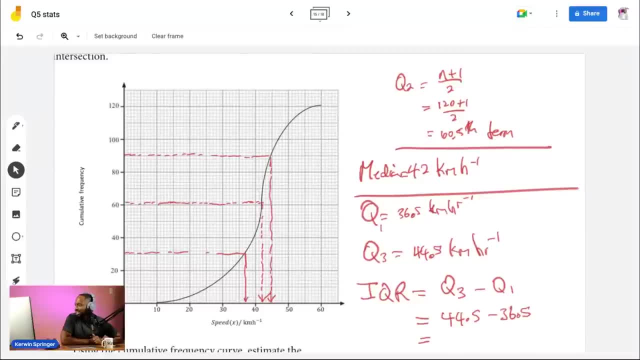 I'm going to check out for Q1.. I get to the 6.5.. It looks like to the 7.. Nah, but I know why. I see to the 6.5. So 8. 8 kilometers per hour. 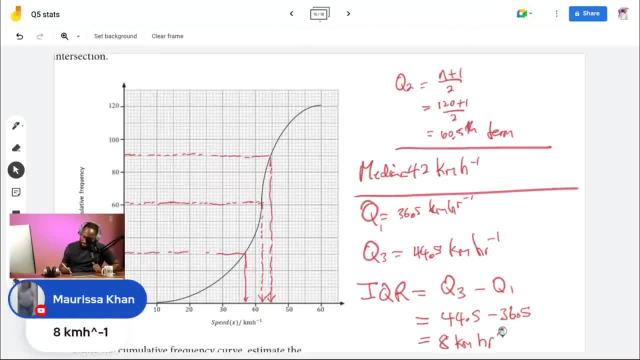 I'll stop writing things just so. now, boy, Pointing the units. now, Why do I need to ask for that again? I need to see again for the pointing units, boy. So what do we do? We do everything. The number of vehicles whose estimate speed is. 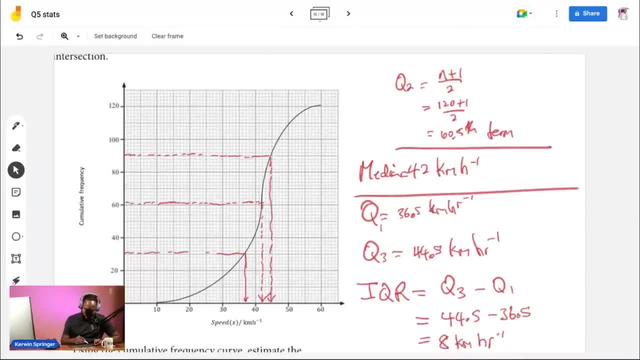 You see this. This question is incomplete, So let me just ignore it. There's something else to tell in here. For the last two it's in question four. So see if you can find it, If I can just show her something incomplete here. 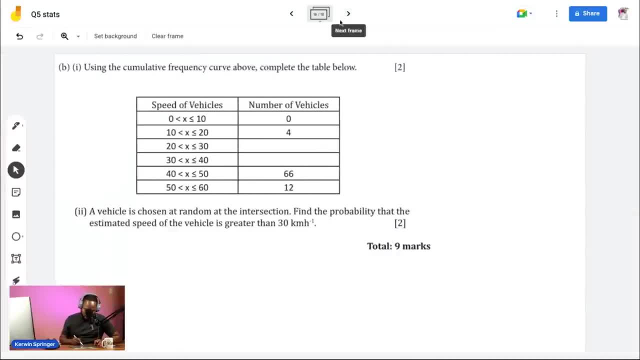 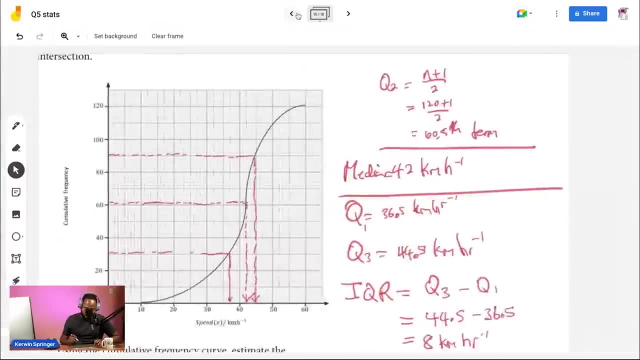 So what I'll do? The number of vehicles whose estimate speed is 35 kilometers per hour or less or more. That's the part missing out of that question. So you go 35. You hit the road And then you come across here. 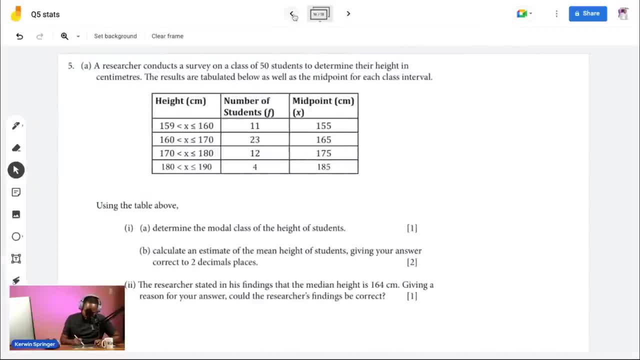 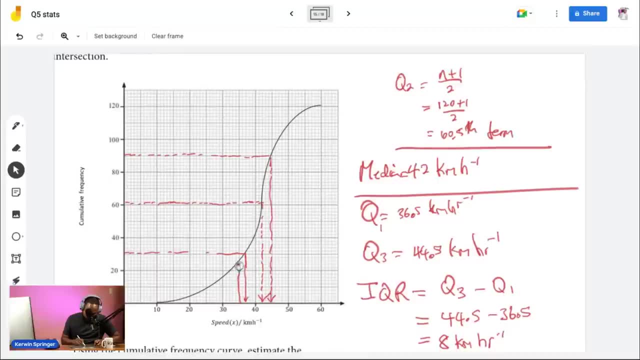 Let me do it on the more zoomed in diagram. So you come from 35. You hit the road again. That's the business line I draw for the series Boy. Hit the road again, Bang, And you come across Dotted lines. 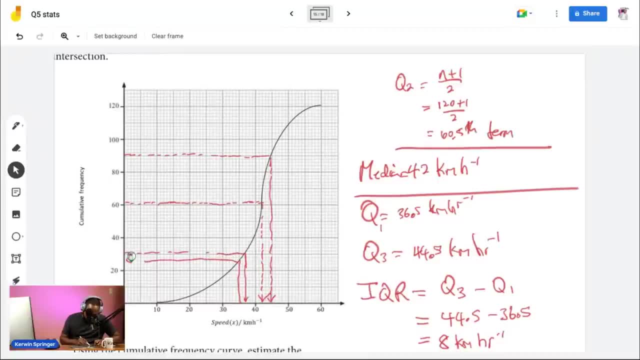 I'm just keeping it straight for 22,, 24,, 26. 26. Remember, you're counting in twos on this axis, So you get 26 students, So you see that number is 26.. So if there was number of vehicles whose estimate speed is 35 kilometers or less is 26.. 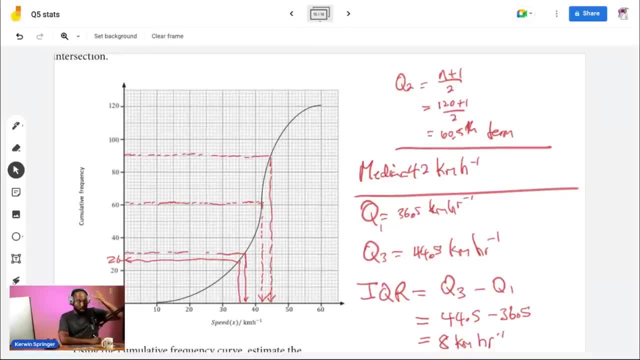 If it's 35 kilometers or more, you would say 120 minus the 26.. So you get rid of the 26. who's slow? And you read it more. Why is it in the chat, if you understand? Yeah, So they're not giving out any topics. 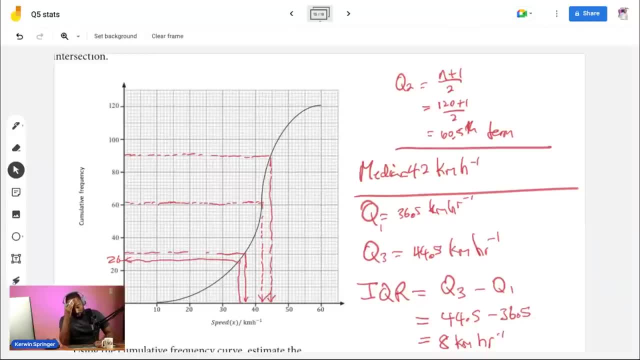 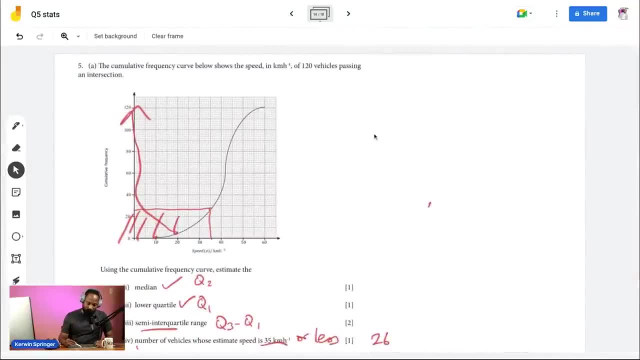 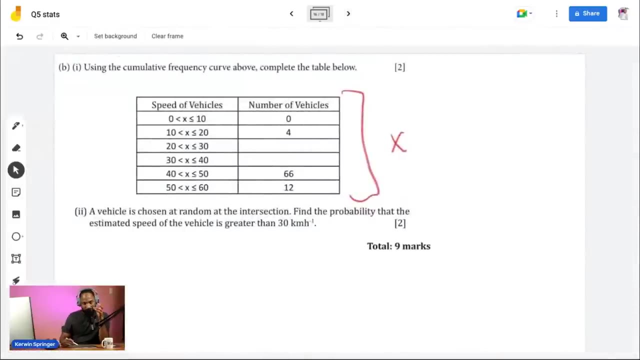 But I got to study everything Using the cumulative frequency curve above Complete the table. So I do this already And you all can check out cumulative frequency curve on my channel to see like the ideas of how to build it from scratch. Build it from scratch. 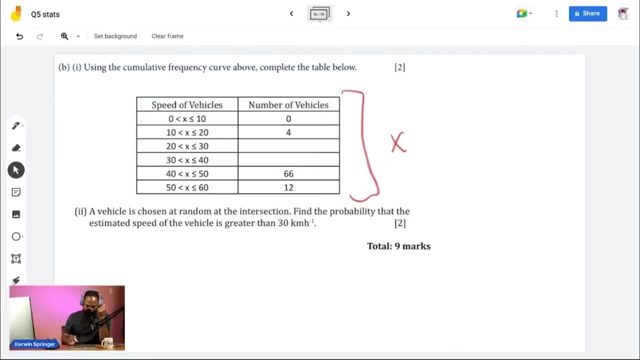 What you want to do is: Can I just do this quickly? There's a probability. I'll skip the probability, But let me just see if I could squeeze this in quickly to see that I do everything now by 20 to 30.. 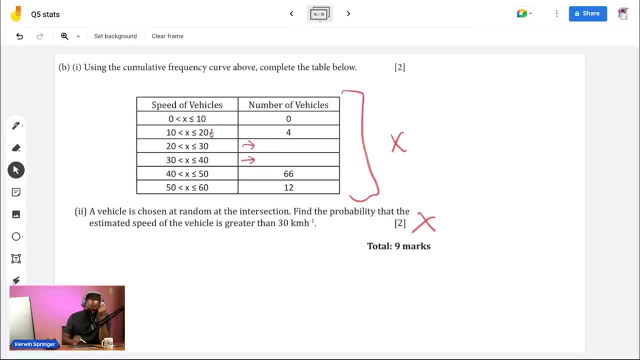 So you see, when it reached 20.5, it was on four. You see now Two, four. So who's the next one? 30.5.. I need to see where it was on 30.5.. So when I go to 30.5, it was on four less than 20.. 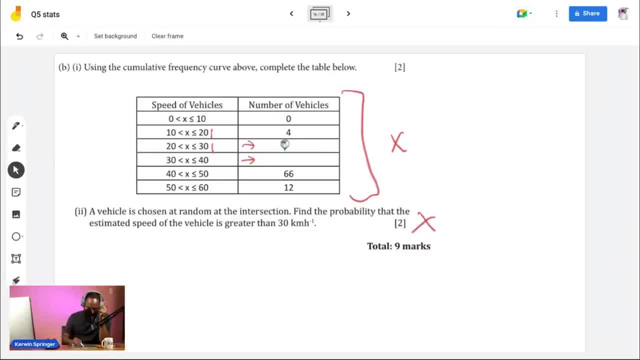 16. So it was on 16.. That don't mean to put 16 here. Come on, people, You have to take away what it had before, So you have to put 12 here. Ah, Because, remember, you add in. 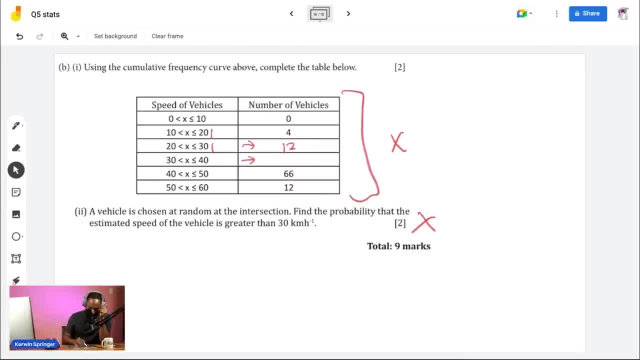 So this and this make 16.. I'm going to show you again. I'm going to do 40.5.. 40.5.. Let me go back. 40.5.. Run up that graph 40.5.. 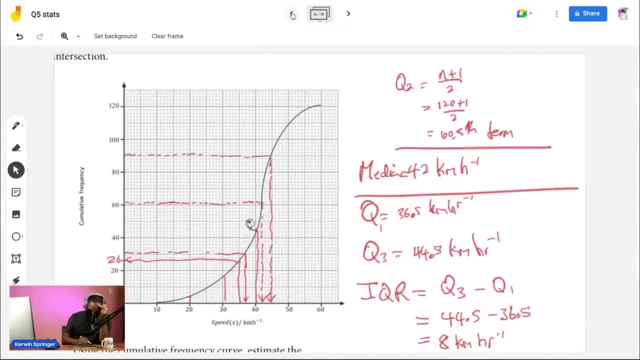 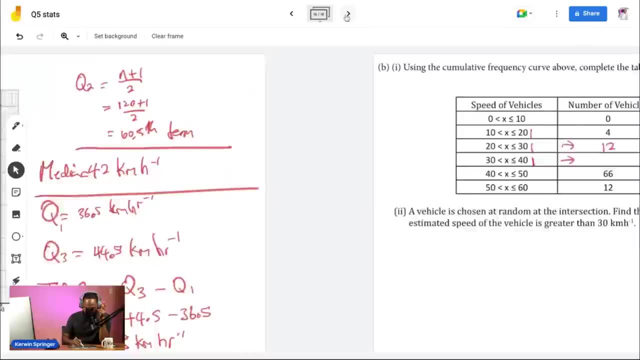 Hit the 40.5.. Looking like 44. And Yeah, Because remember you're counting in two, So there's 44. So let me go back to 16.. So that don't mean to put 44 over here. 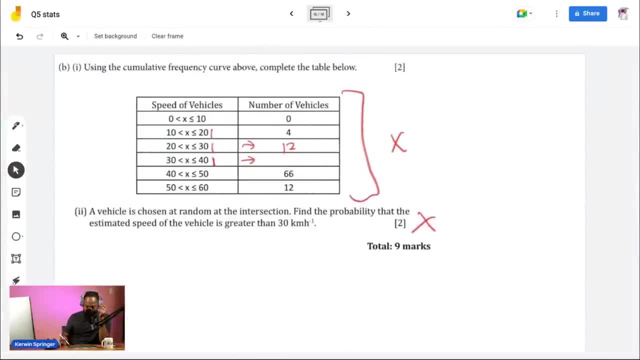 And slide 16.. You don't need to put 44 over there. You need to take away all them things from before too. So if I take away 44 minus 16, how much I'll get 28.. Now I just need to add up all of this. 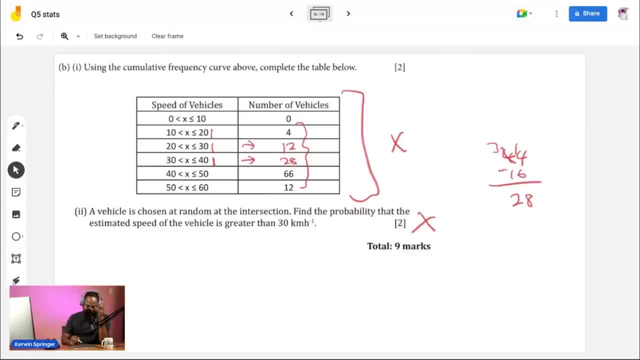 26, 28, to make sure you get the same, the total number of vehicles. So I can do it and double check. If you realize you're off by one or two, you could just tweak one of the numbers so that it could be exact. 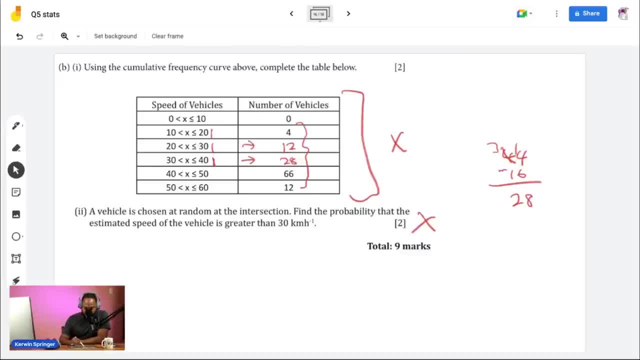 All right. It's hard for me to get say like: I totally confident in my numbers because I'm using a digital thing here. I can't see everything, So that's how you do cumulative frequency in reverse. Check my video to see how I did forward. 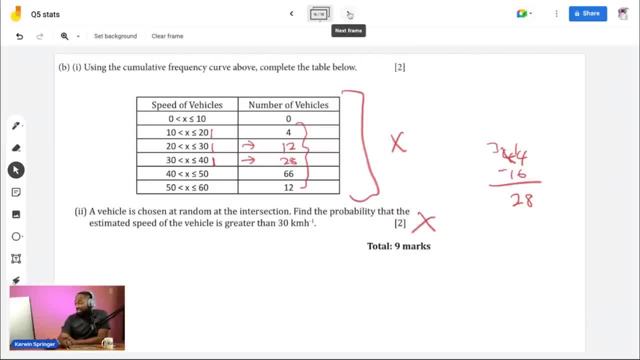 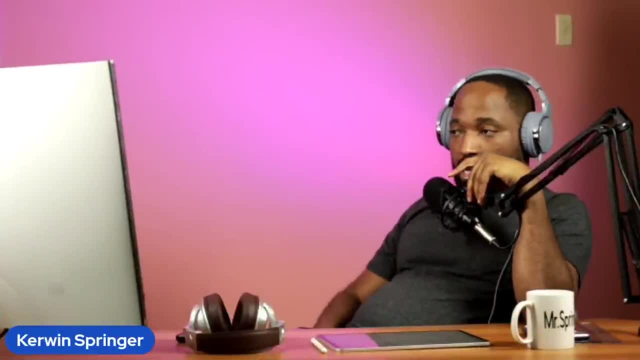 And then we'll move on to a last question, because I've spent that next five minutes here. Next question, Question five: boys. I'll leave you not a probability one, We do things like that. enough already. Another question five. I feel like we good day. 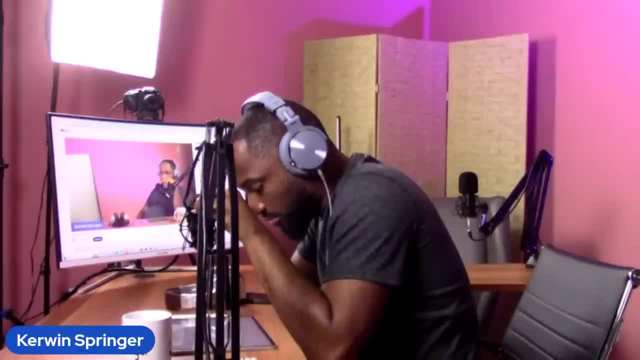 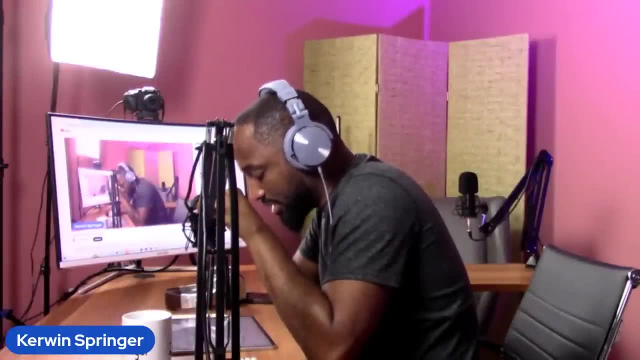 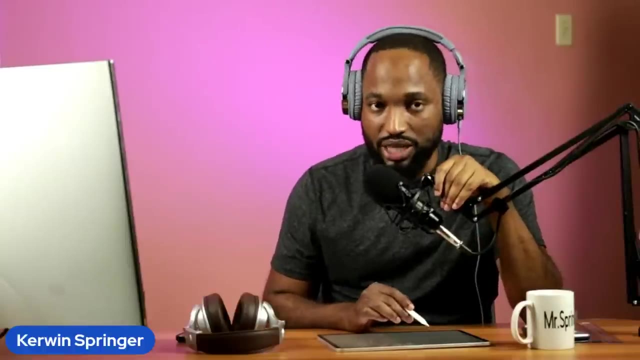 What is next? question five is about Model class Mean: Same thing, Same effects. So you see that model class talk. eh, It's the model class. Other people you can do this. Stick a screenshot and do it now and put the answers in the chat. 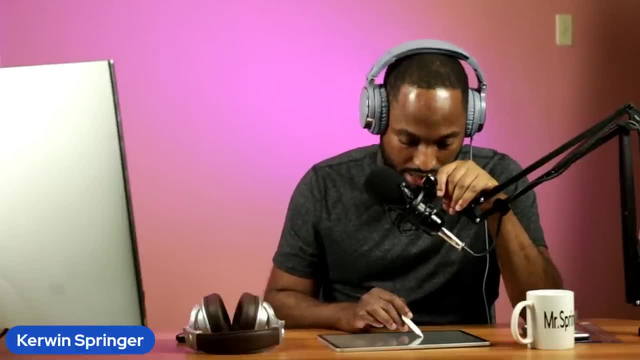 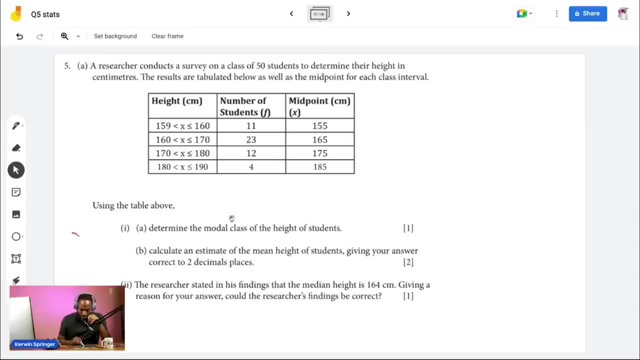 Modal class. Bring it up. Modal class. I'm not giving no hints. Modal means most frequent. I'll just give a hint: Calculated estimates of the mean height. I do this already. This is the sum of fx over the sum of f. 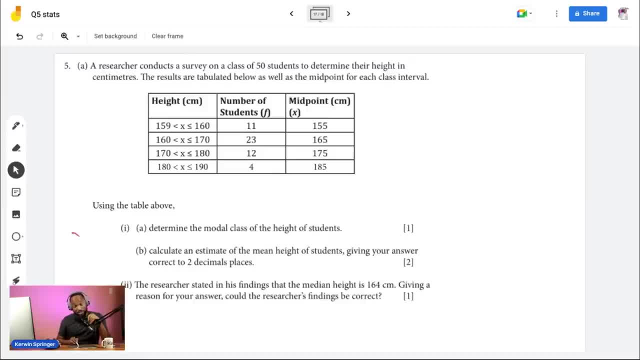 And you see, just seated inside, that the median height is 164.. And I just do this too. How do we prove if the median is correct? How do we prove if that median is correct? Give an answer, And then the next part on slide 18.. 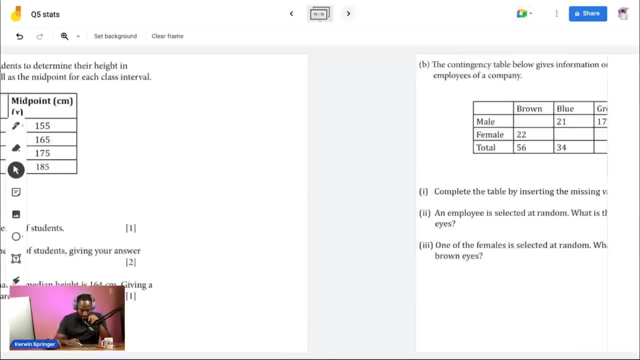 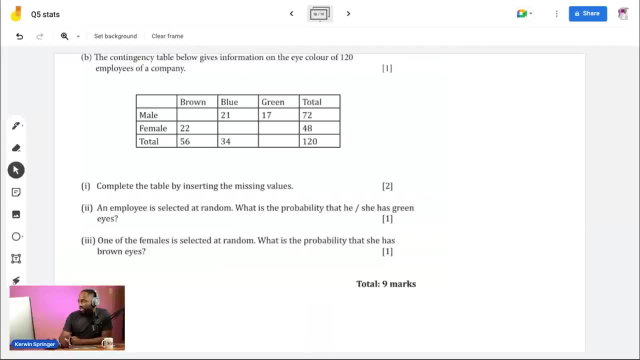 We are going to do slide 18 because it's kind of different to what we are accustomed to. This is like the deepest probabilities getting to the c-segment, So let me take a little dive on slide 18.. Last one: This is the finals here. 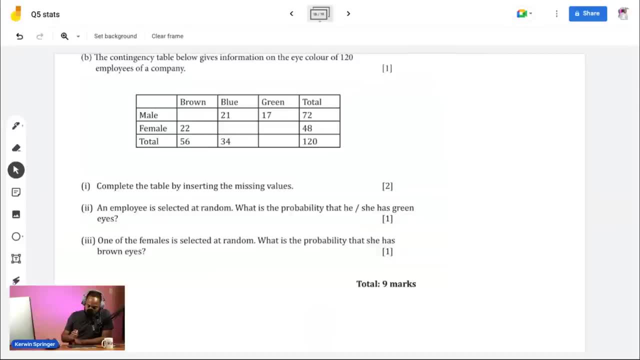 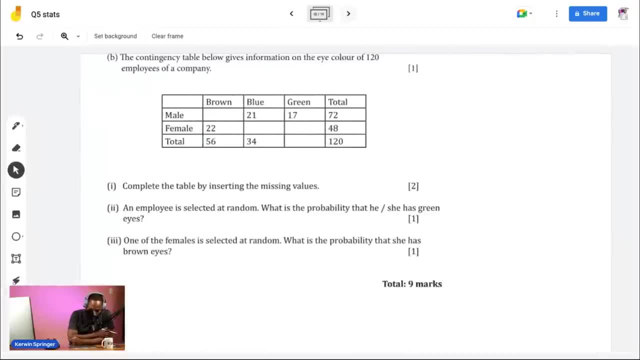 So I hope I'll take a screenshot of slide 17.. Let me just go back to it. Take a screenshot of that and see if you can do this slide 17.. All right, And let me go to slide 18 now. Okay, So complete the table by inserting the missing values. 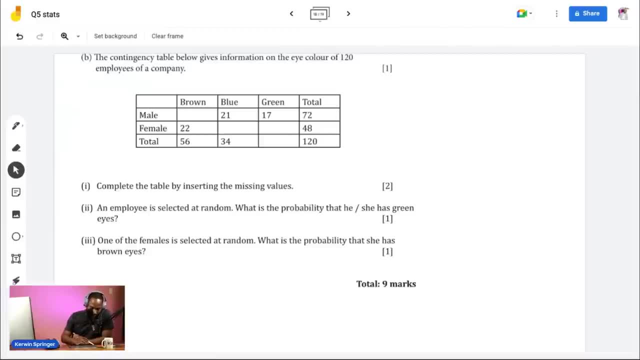 How are we figuring this out? Oh, it's a totals. Oh, it's a totals. There's a total line here and a total line there. So it's total on the left hand, total on the top. So if it has 72 here, it's like Sudoku. 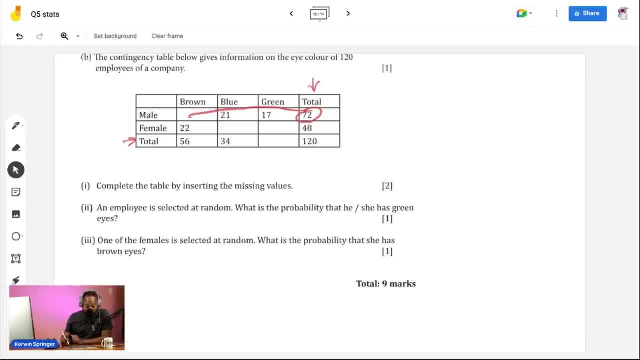 You're missing that number there. What could that number be, boy? It's so hard, It's so hard. All right, So 22 and 52.. You say, oh, they give you a real clue to this boy. 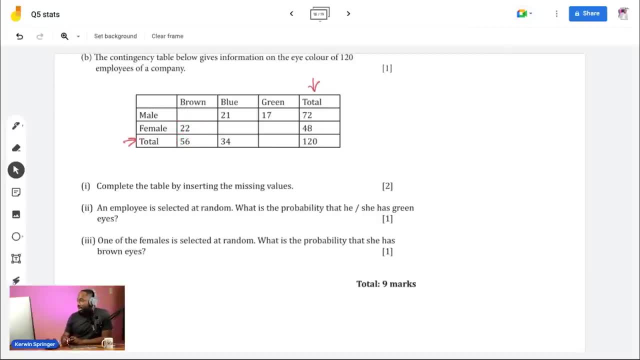 And what could that number possibly be? Class 34.. 24.. That number ought to be 34, boy, Yeah, 34.. So when I subtract this from that, I get 34.. If I subtract this from that, I get 34.. 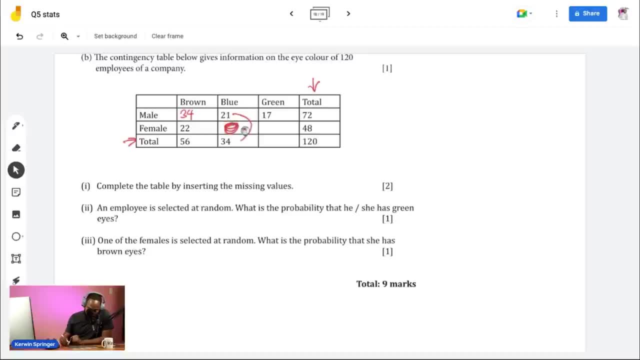 What about this? What can the number be here? Well, I have these two, So I just need- and you're surely working- 34 minus 21.. And you will get come on critical thinking skills. So after I get this one, I'll be able to figure out this one. 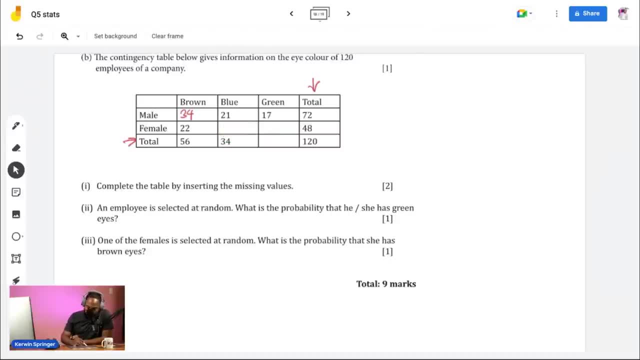 then this one, Niceness, niceness. So I got 13 here And this plus this I use in each other, this plus this subtracted from 48.. So I want 48 minus 35.. And that will give me my missing term there. 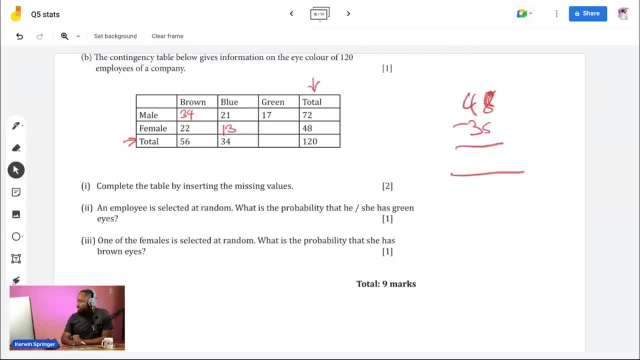 I get the 35,, 22 plus 13,, which is 13 again, And then finally I add these two together And I double check to make sure that all of these add up as well. They could have leave out more things. 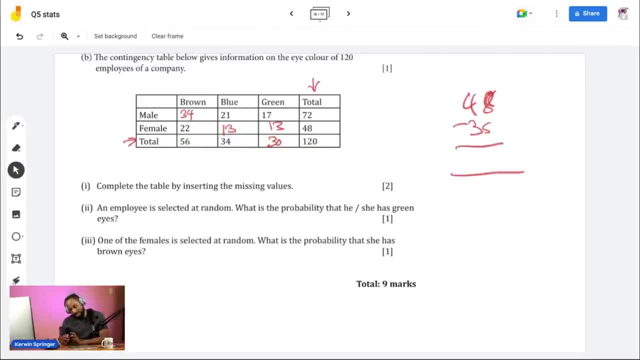 They could have leave out more things, because it was kind of easy, boy. They could have leave out a little more things to make it a little more challenging. An employee is selected at random. What is the probability that she has green eyes, That he or she has green eyes? 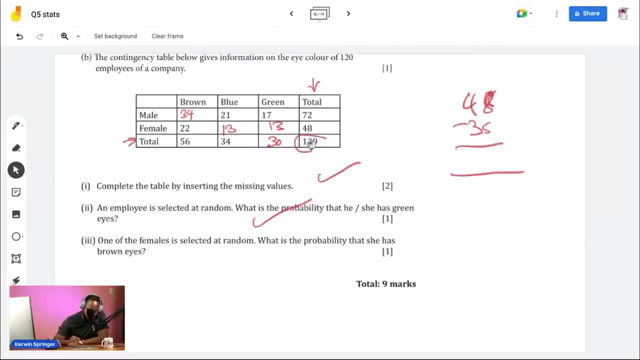 So they want the total employees. So you use this number: Total number of employees- right, Okay, Okay, So the probability that they have green is the number of desired outcomes. I fed up, right, this boy. I'm writing this again. 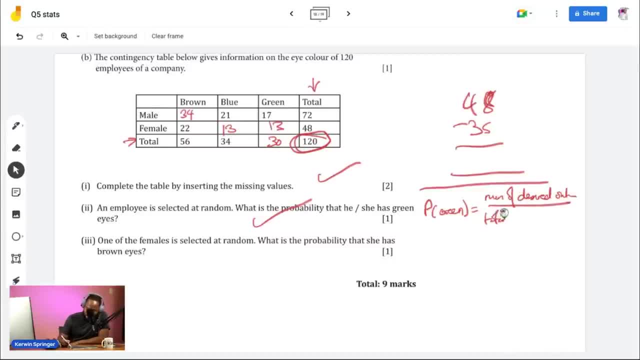 The number of desired outcomes is the total number of outcomes And the number of desired is 13.. Oh no, 30, 30.. 30 people have green eyes. That is a he or she And it's a 120.. 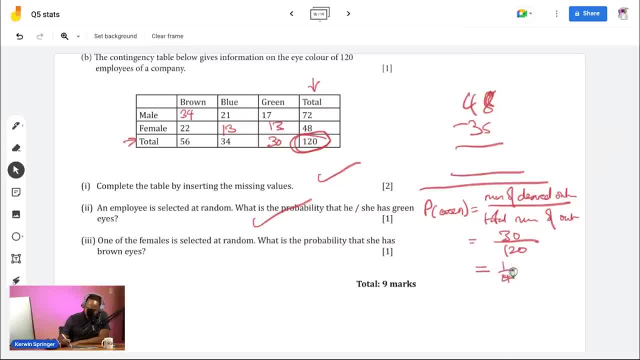 So this is a quarter, 25%, 0.25 probability. It can be expressed. It can be expressed as a percentage, a fraction or a decimal. One of the females is selected at random, So it's a female, And I waited some kind of cringe these days, boy. 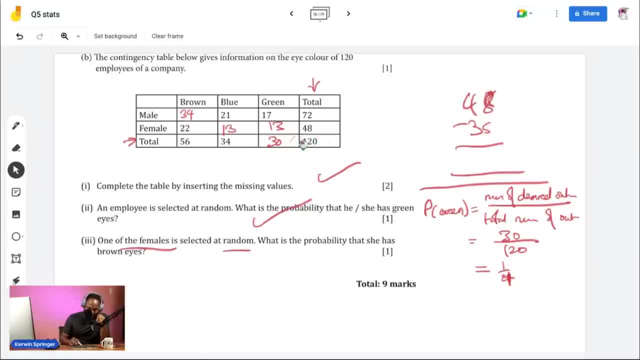 And you see it's a female. Okay. So all right, How much, how much? how much? ladies: 48.. 48 females. What is the probability that she has brown eyes? So you already select the female. So it's out of 48 now. 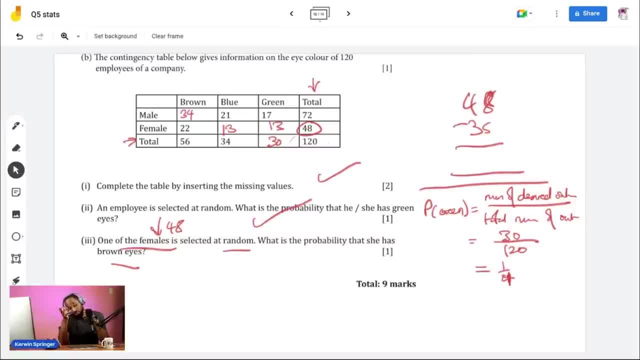 Why isn't it checked? if you understand, It's not out of 120. now You selected already. You already Selected a female And what is the probability that this female, given that you have already selected a female, has brown eyes? 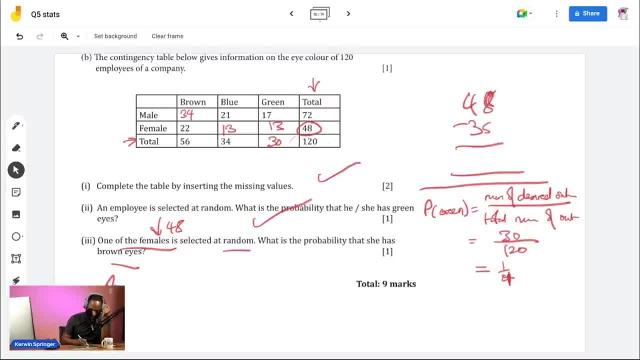 So this probability for brown has to be a 22 out of the 48,, which is 11 out of 24.. And we're cooking it Ramco gas there. So that's a little walk-in statistics. Notice, we just did some pie charts. 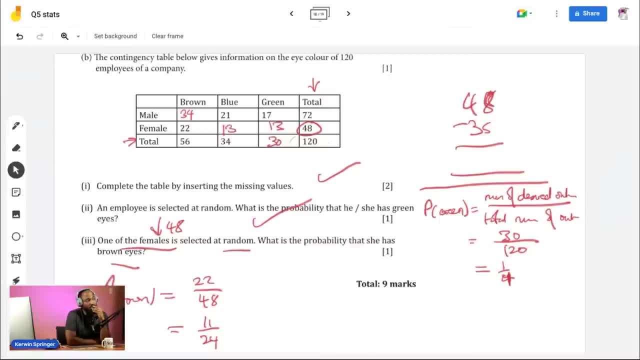 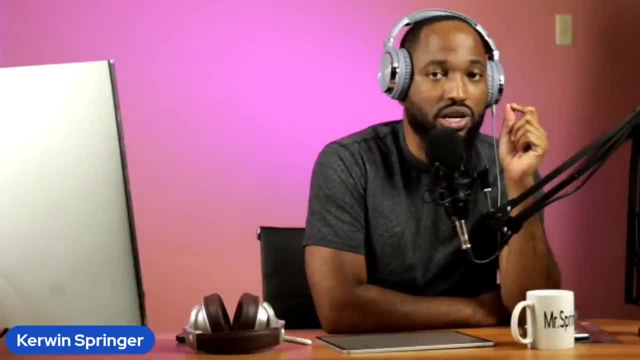 We did a bar graph. We didn't really look at histograms, Did we No? So go and search Kerwin's, bring out histograms on the channel and watch out them. histogram video. Watch out the other statistics video After we do every session. 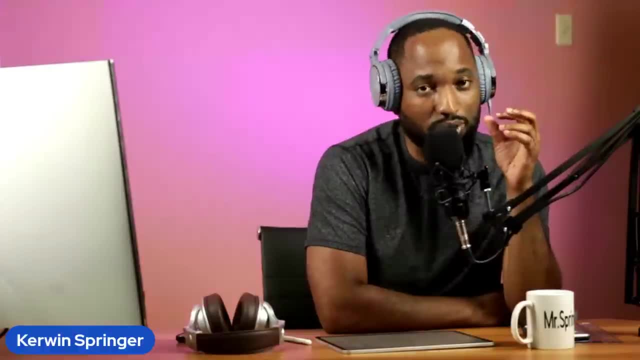 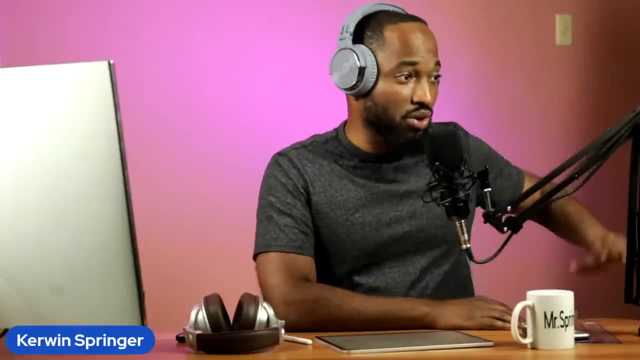 you could go out and look up the individual topics on the channel and you'll see little snippets- Those of y'all in my class. after we do the topic you could go back in the whole class and watch over that whole class. You'll have an extended version of it. 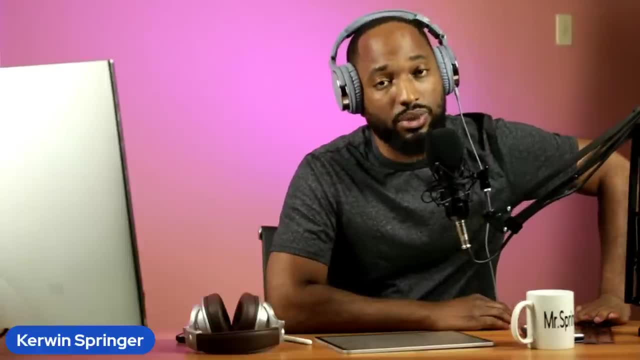 So y'all, could I know y'all- have good type of notes and then you'll have all the compilations and the assignments and the solutions And you know which. you tell your nice in the classes any student up, So run the. 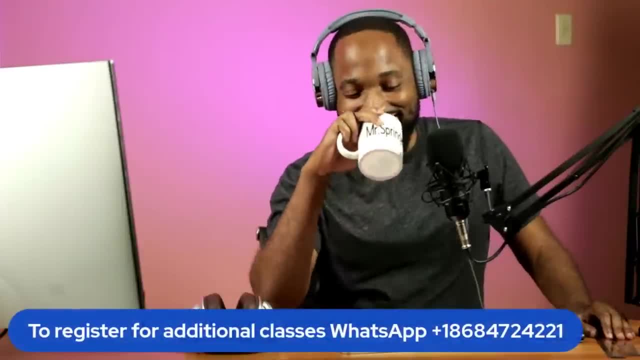 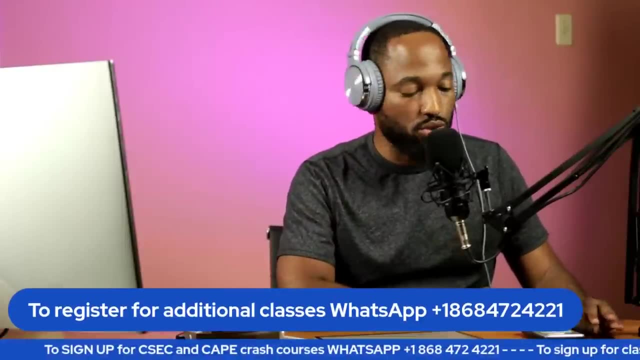 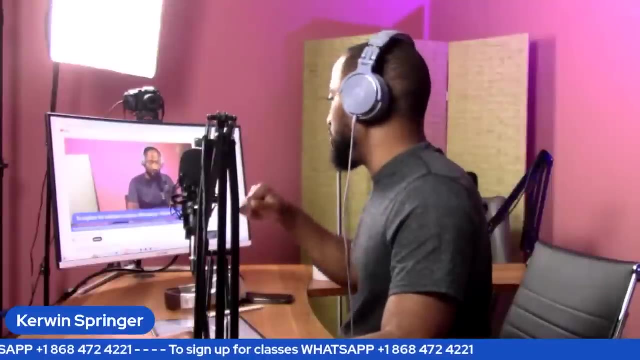 run the ad day one time Next week, Saturday crash course. Those of y'all in my class, y'all in free, Those of y'all who not in the class, sign up by what's up in this number on the screen for seven to four to two one. 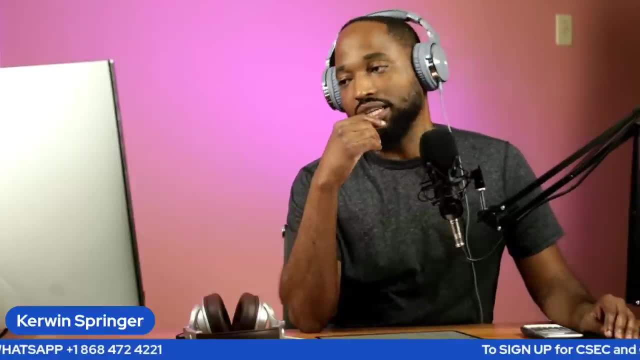 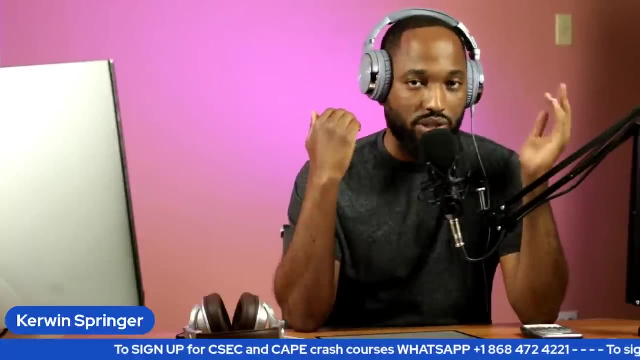 Remind us, to remind me to change that number to the new number. Right, But you could still use that number for seven to four to two one. We have students from Jamaica signing up. We have students from Barbados, Of course, you always have the Trinidad and Guyana. 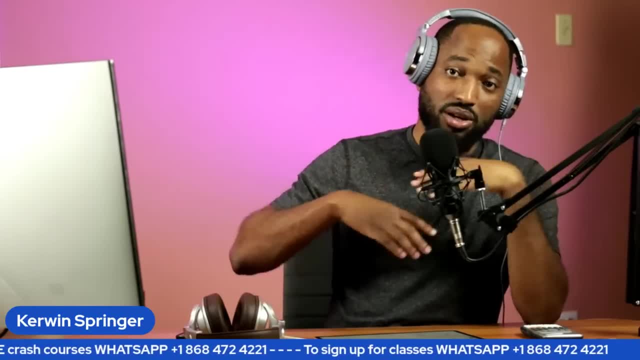 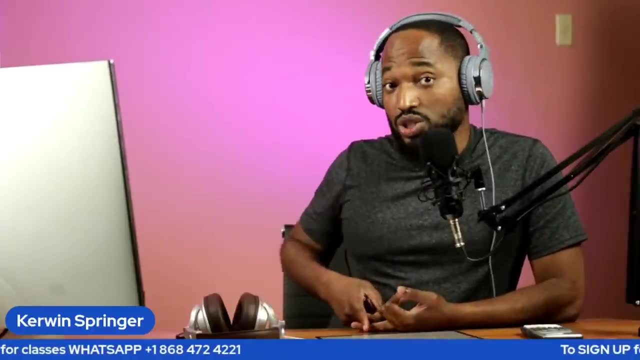 Those are the two largest countries for the student hub classes, right, But we actually have students from all over. We have had students from every single country in the Caribbean. We always have a clip from Grenada, from St Lucia, from Antigua. 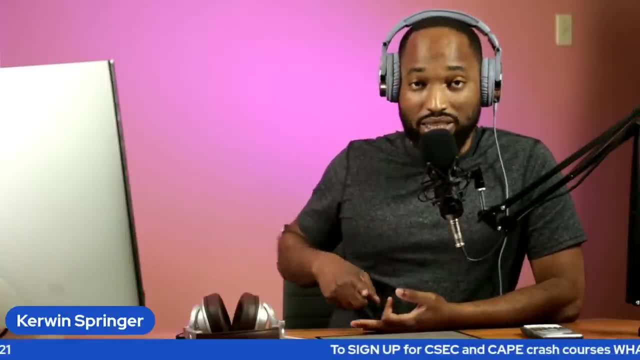 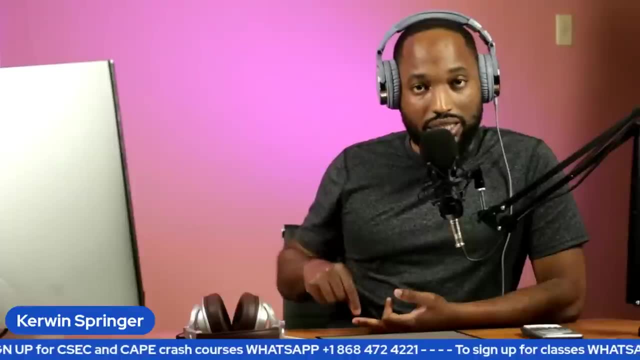 some of the top students in Antigua, Grenada and St Lucia Like. when I say some of the top, I mean the top, the student who did the best in CXC. for certain years we got them from Antigua Most. 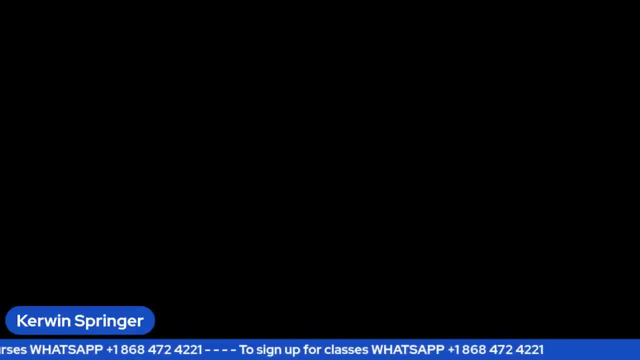 most number of subjects: 15, 14.. So the student hub is really the place, is really really pleased to be. love arm lessons.